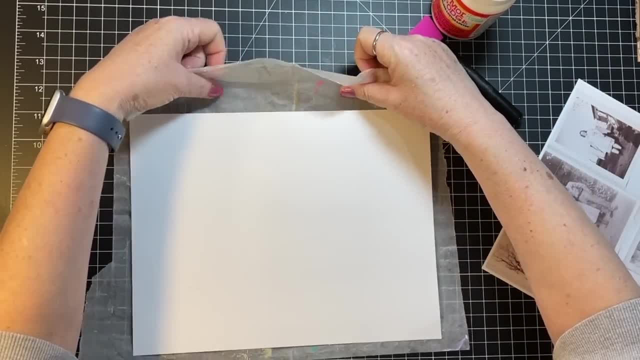 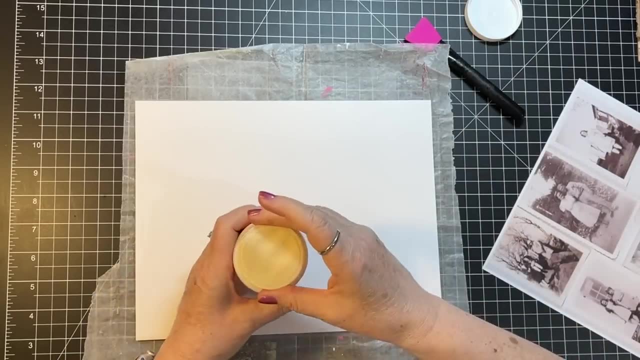 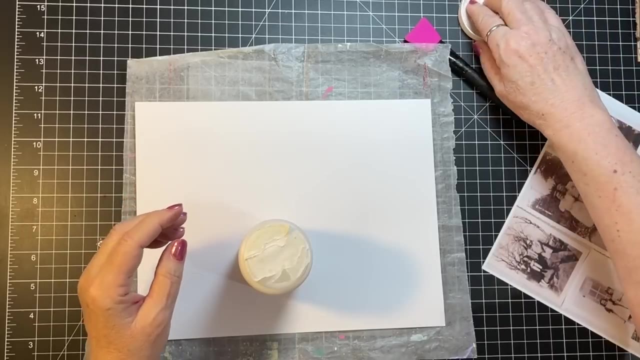 gonna do is then I'll just, if it curls, I'll put it under a book or something to flatten it out. I find that works pretty well, Let's see. Well, obviously I haven't been into this Mod Podge. I haven't been into this Mod Podge in a while. 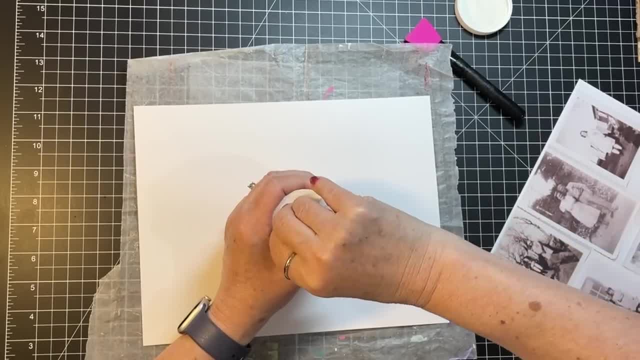 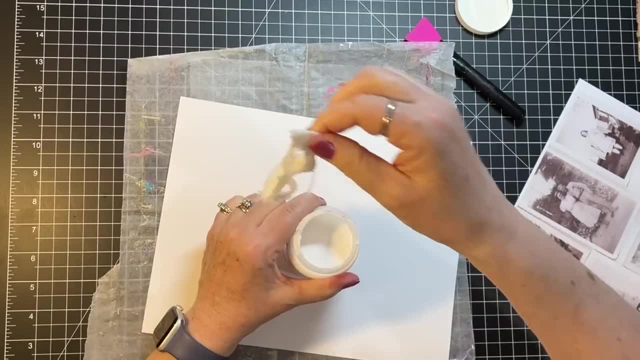 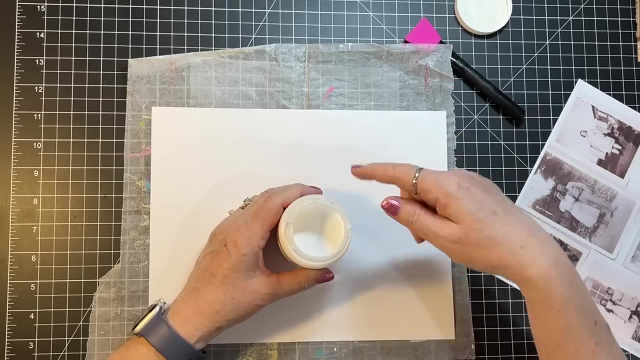 Yuck, Excuse me. while I Maybe it's never been opened, It's still got like plastic on it. There we go. Okay, I'll have to get some. I like to put wax paper on when I put the lid on so it doesn't stick. 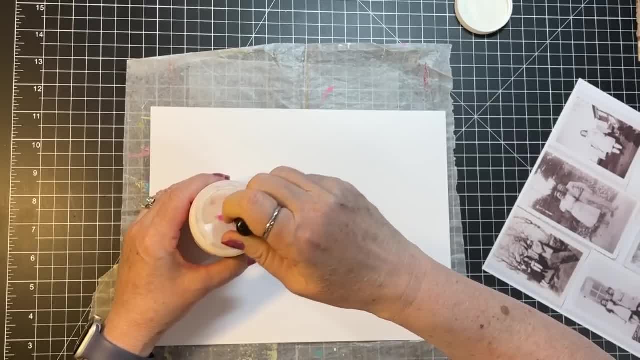 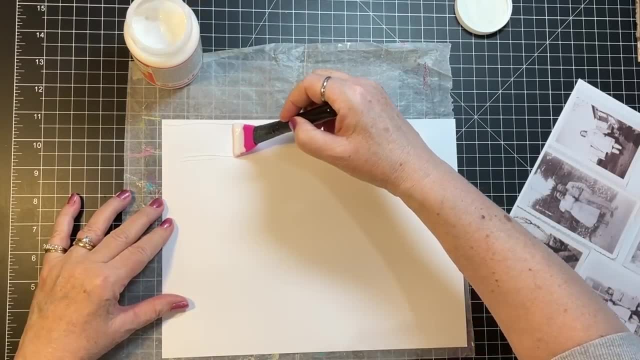 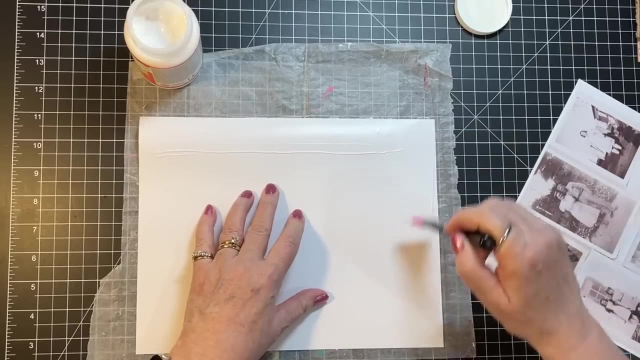 But anyways, let's see. Let's see how we do. Okay, I'm going to try to just put a thin bit on this. Oh yeah, it's going to curl. Oh well, we'll see if we can do it kind of quickly. 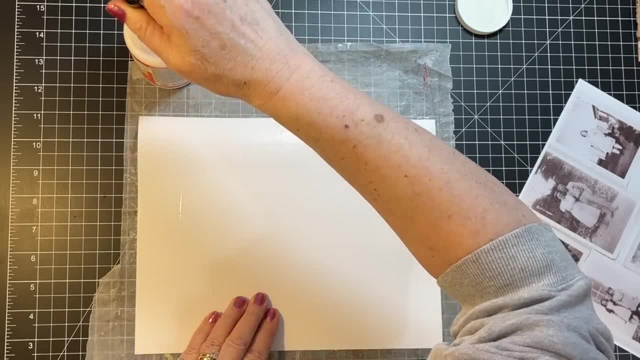 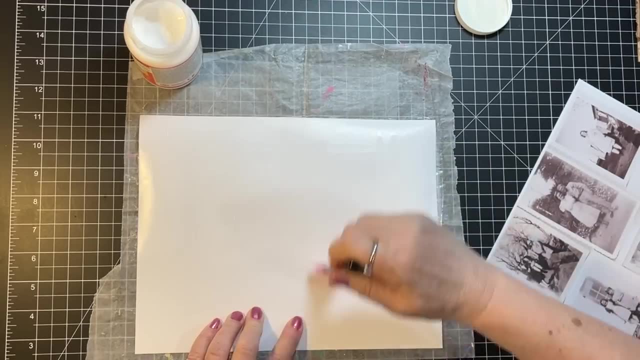 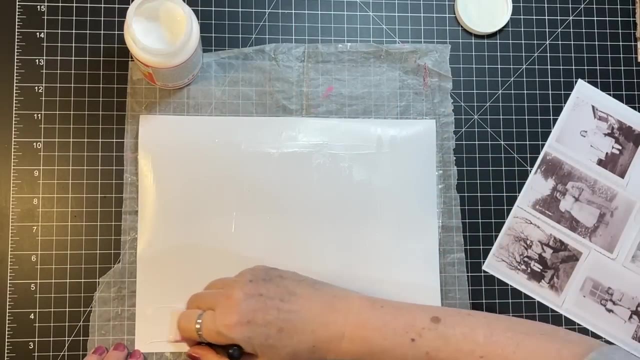 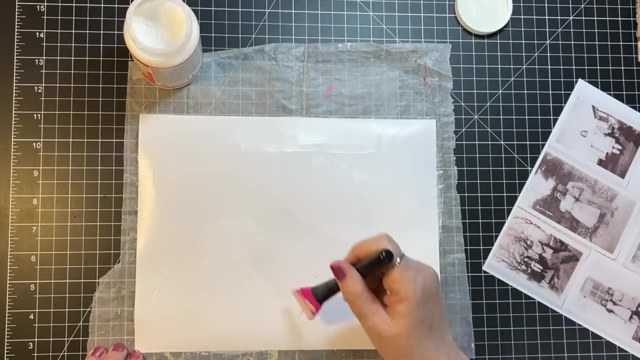 So maybe should have done half and then the other half, I don't know. Hopefully I can do it quick enough. Let's just see. Let's just see what happens. Play day, Play day, Total play day. Put another bit down there. 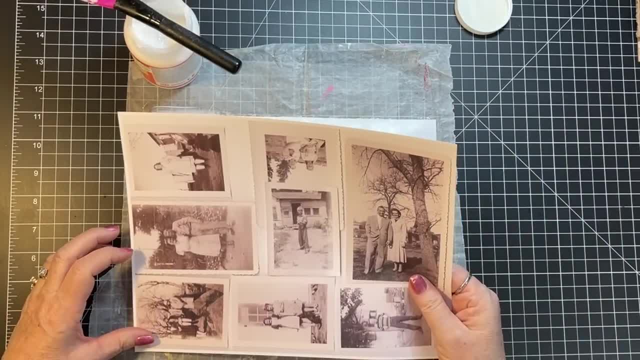 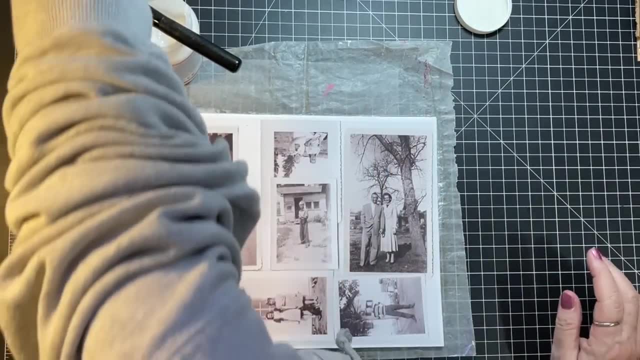 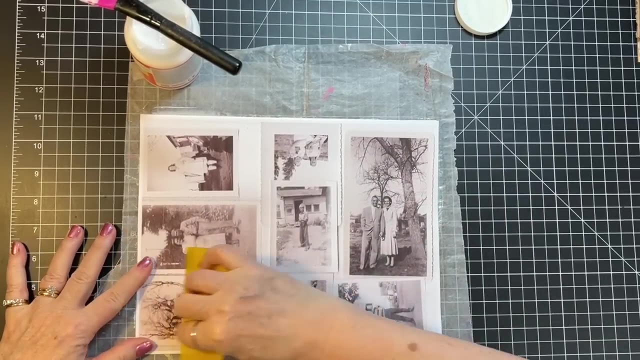 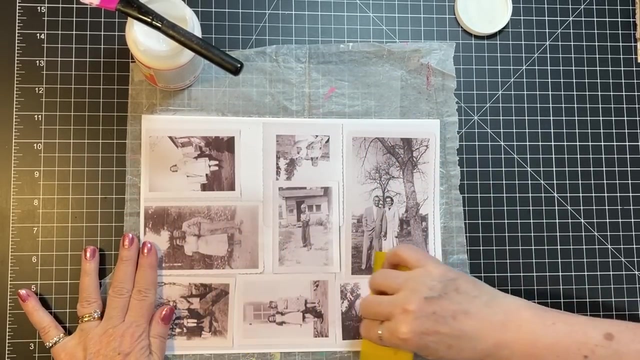 Okay. Okay, now I'm going to stick this on there Like that. Okay, maybe we'll use: Oh, excuse the reach This thing, Smoosh it down. Okay, I wanted to do this first so it could dry while we're doing other things. 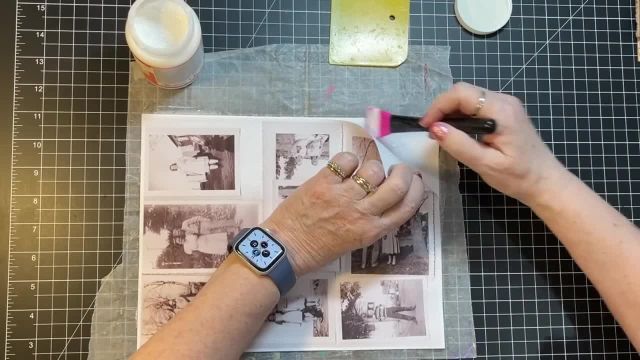 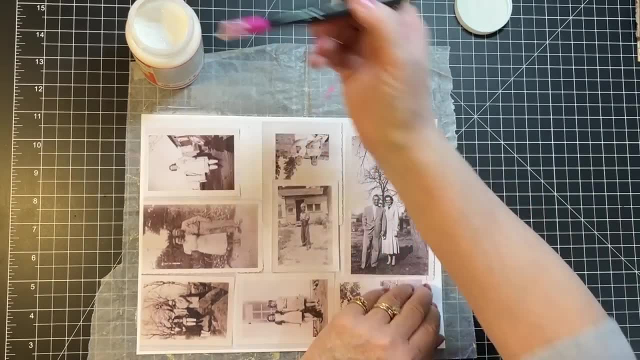 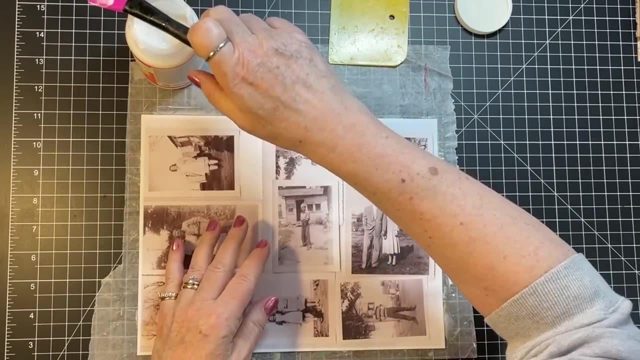 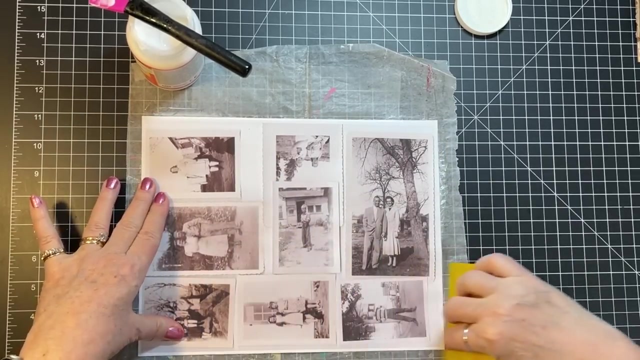 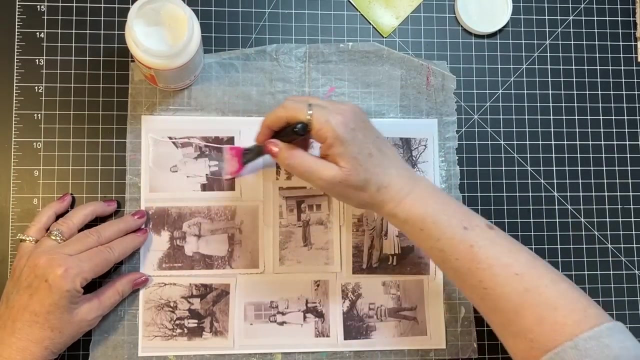 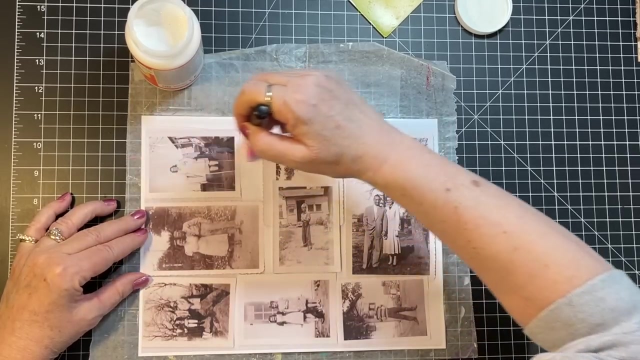 Well, I didn't get enough on the edges here. Okay, All right, We'll see. Okay, So there's that. Then I was thinking, if I just put that over the top to see, Okay, I don't want streaks. 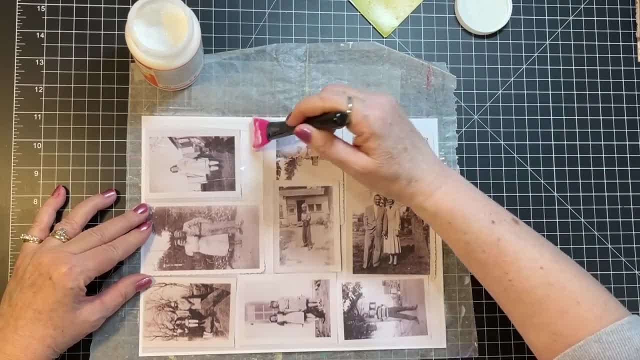 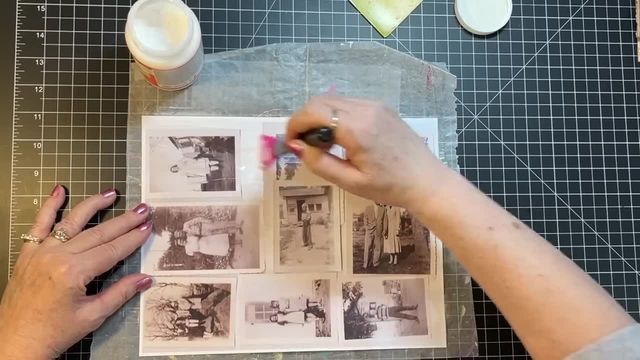 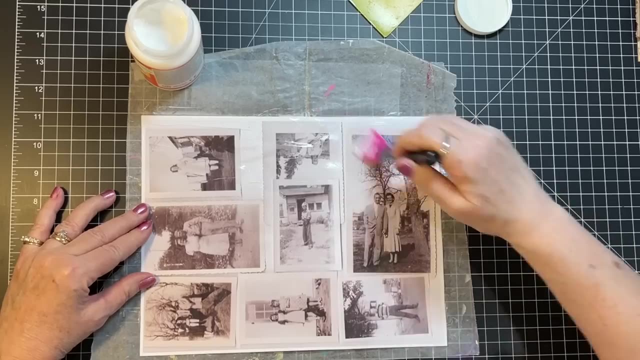 I don't want streaks, though. I don't know how that one's going to work, because it's kind of half and half. I love having a play, though, and just seeing you know, nothing ventured, nothing gained. That's what they say. 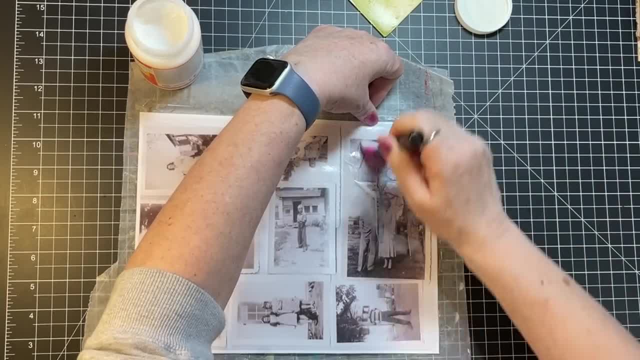 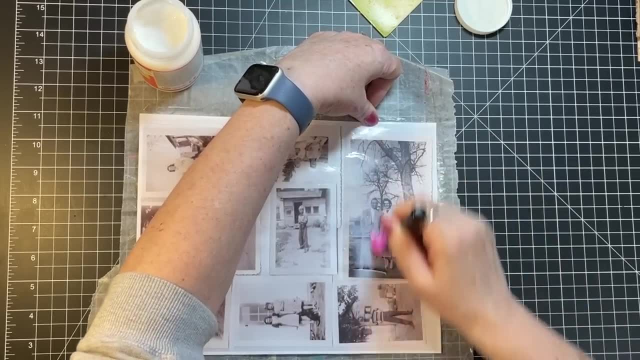 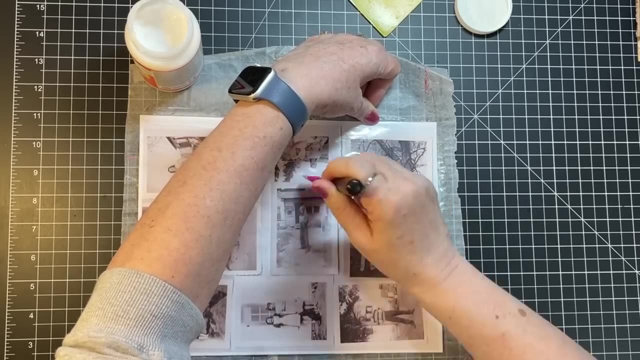 I don't know who says that, but they do And I agree, Just give it a whirl. If you have an idea, give it a whirl and see what happens. And, like I say on this particular project, if it doesn't work, I've wasted a piece of paper and a piece of cardstock. 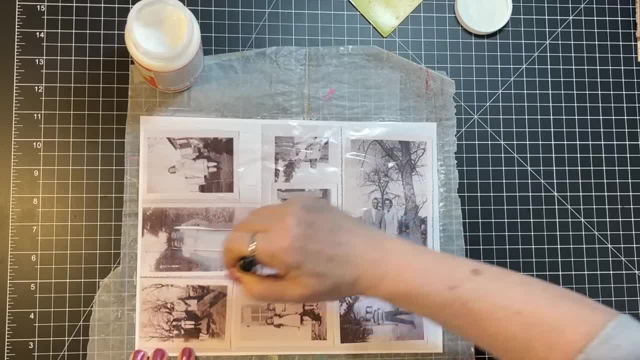 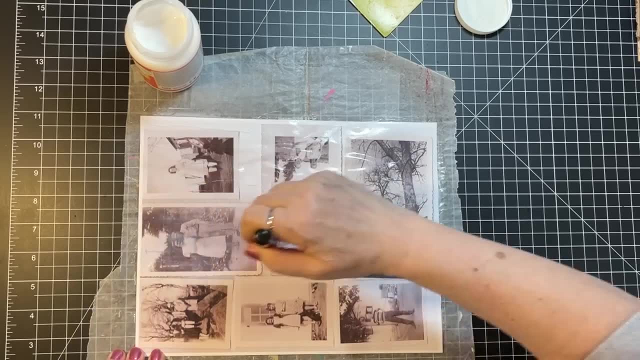 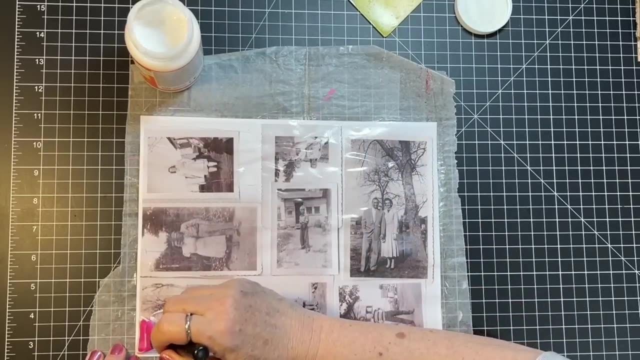 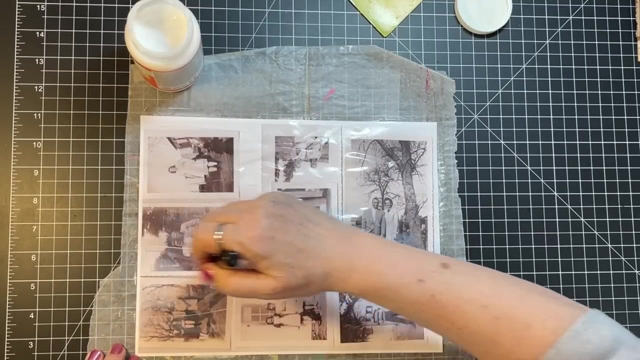 Not the end of the world. So I had a lovely morning this morning I called my brother. Today was his birthday. He had a nice catch-up. They were just on a trip. It sounded amazing. They took a cruise out of Hanoi, Vietnam. 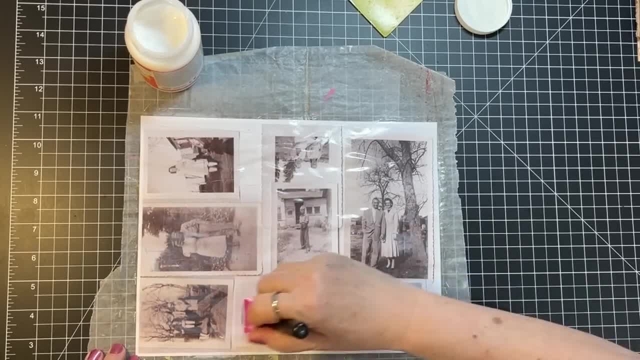 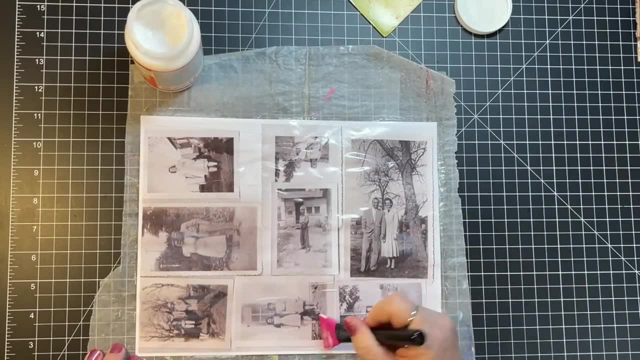 Yeah, They're quite the travelers. They love kind of the world traveling. I'm going to show you something. My sister-in-law is from London, So they've been to, of course, Europe many times, but they've been all over the place. 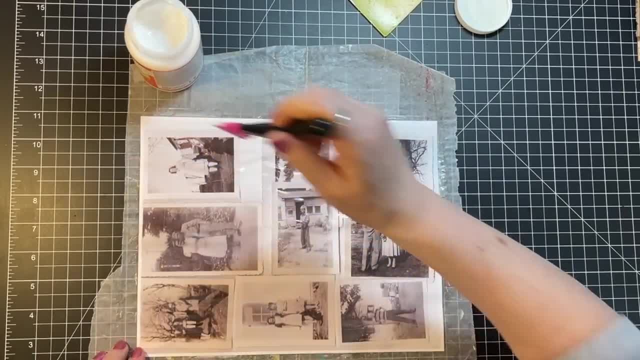 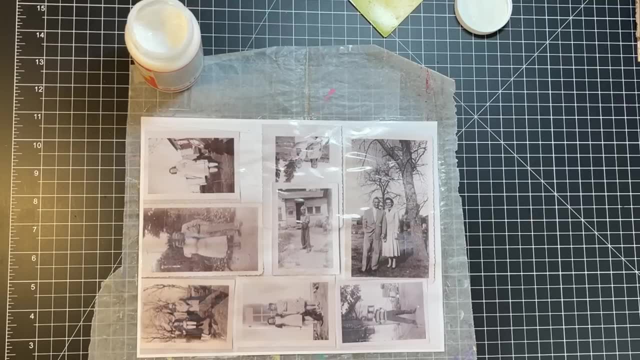 I don't know if this is going to work people, It's kind of buckling. Well, we'll just see. We'll just see, Let's get. I'm working on trying to get out a baby wipe. More than one has come out. 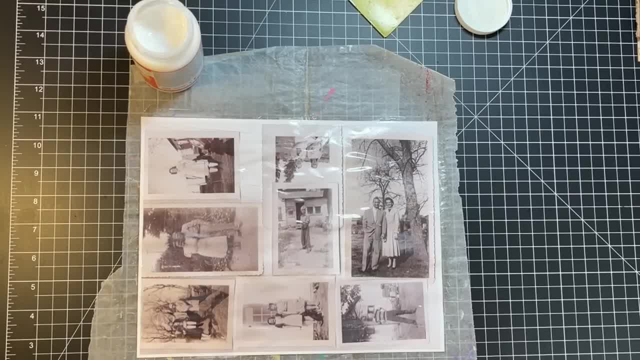 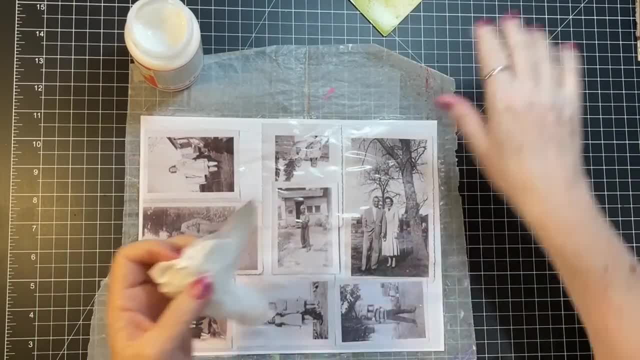 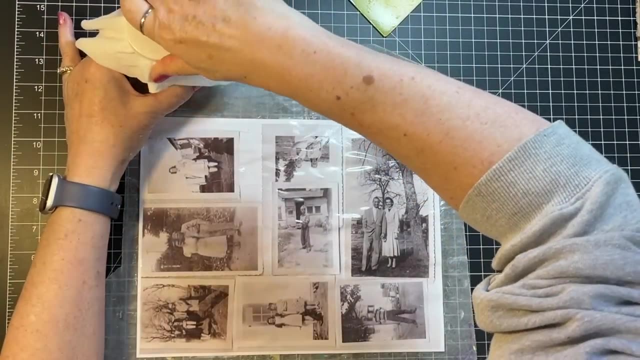 Okay, Well, we'll see. We'll see what it does. Okay, That is done, And maybe what I'll do is just put this little. I'm going to put that on there. That'll work. That works too. 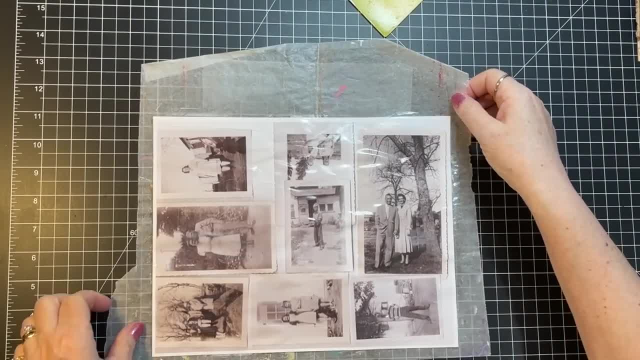 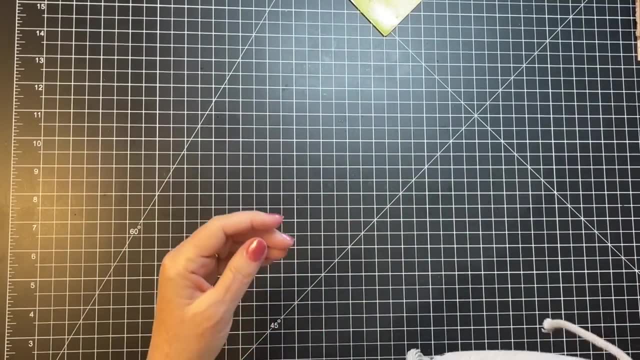 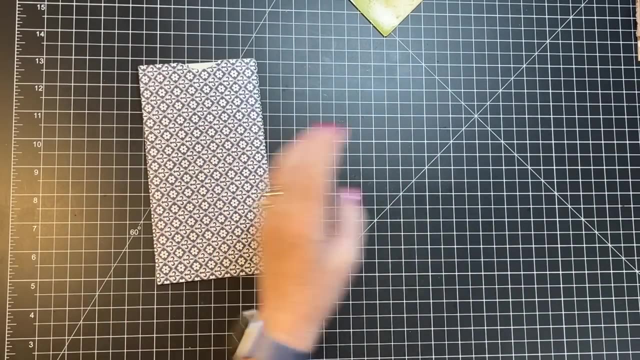 Just something so that the lid doesn't stick closed. Okay, I'm going to set this aside and we'll play with other things until then, Until that dries, Okay, So I have this. that is from one of the Roxy Weekly Challenge. 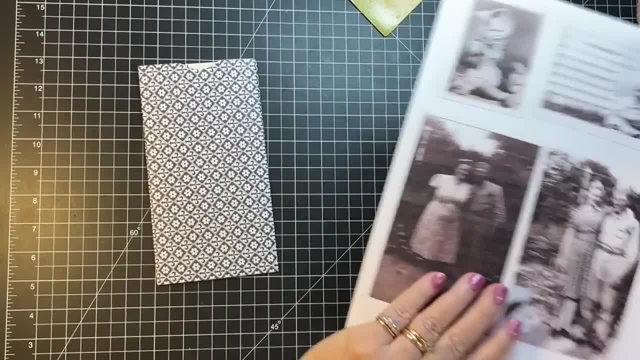 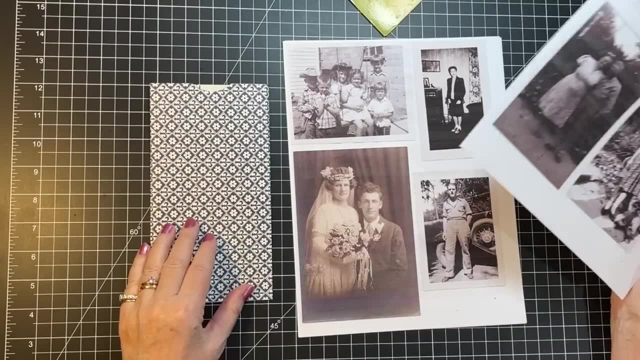 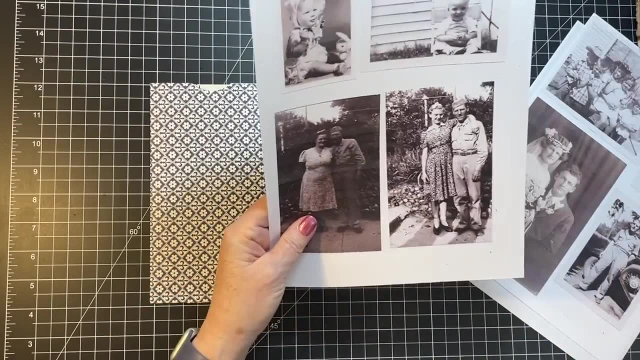 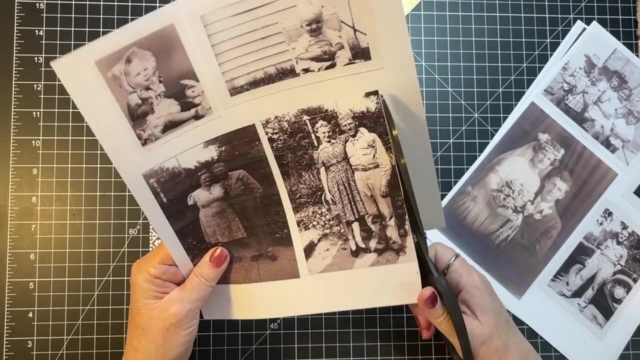 One of her things And I was thinking it'd be fun to put like that one maybe. Okay, I think I'll put this one Okay And I'll decorate that up a little bit. I've just been dying to play with these. 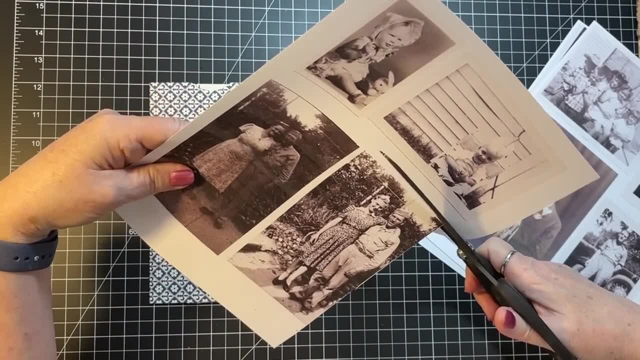 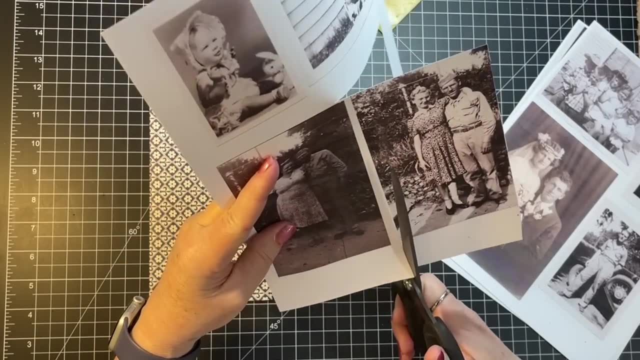 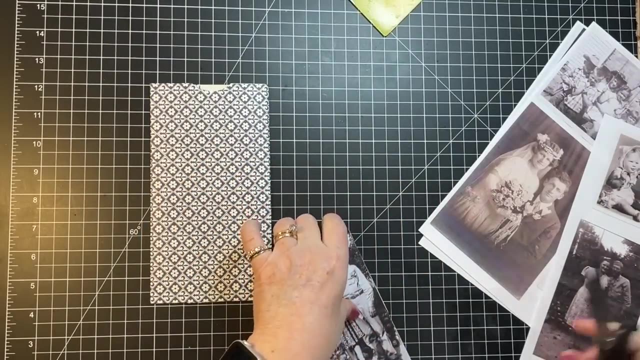 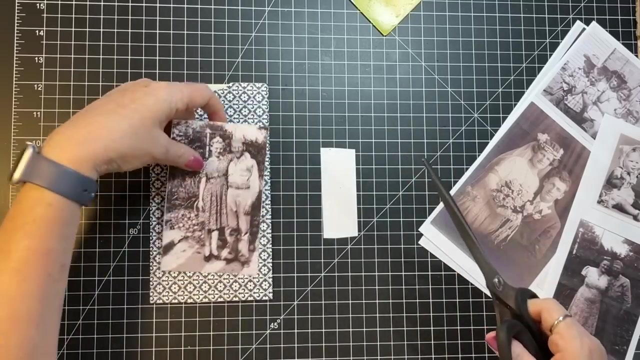 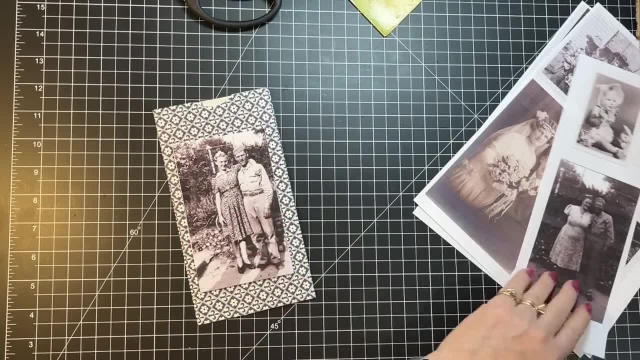 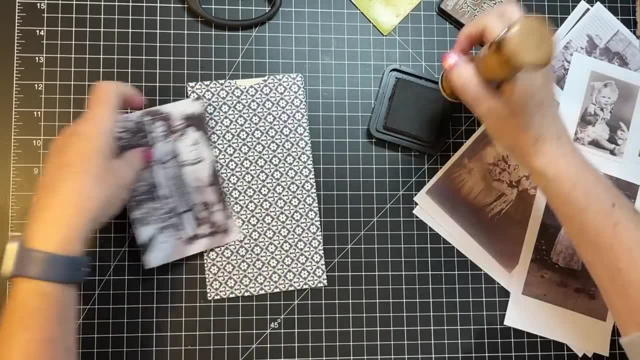 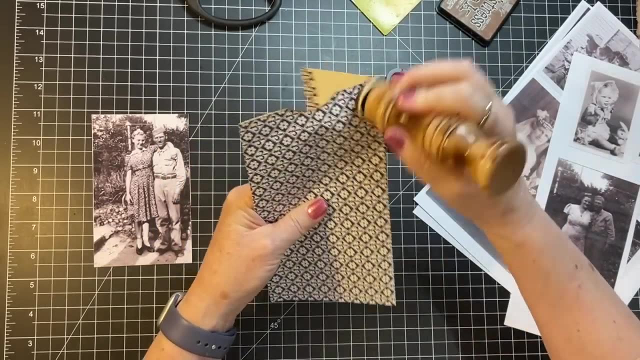 Okay, Okay, Okay, Okay, Okay, Okay, Okay. Yeah, that's a great size. Okay, Let's see, I'm going to put a little of this on the whole, The whole kitten caboodle, as they say. 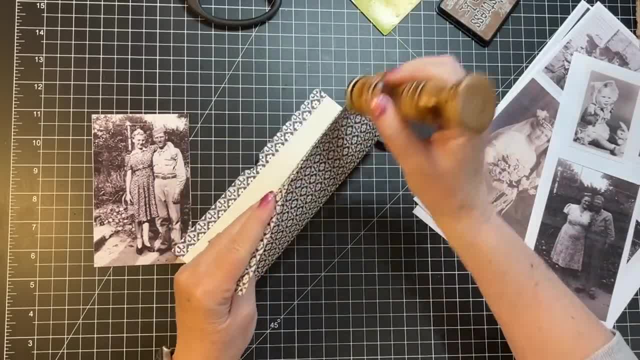 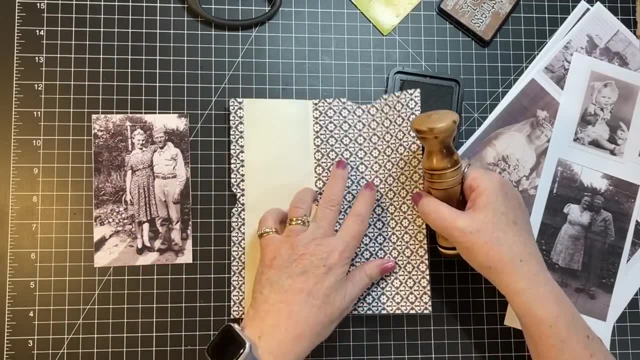 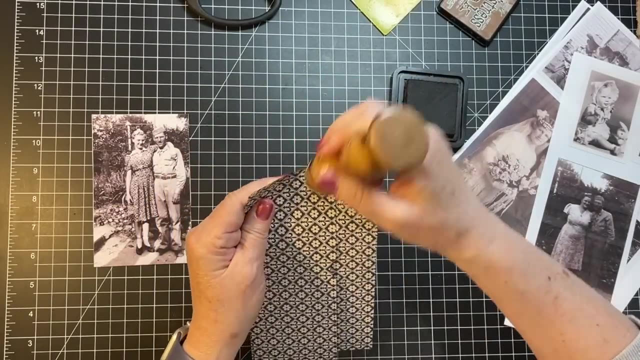 Let's see, And this will flip out. So I might want to put some coffee dyed paper on the inside And then That's writeable then, And then this will be on the other page. so we'll kind of deal with it later. So yeah, you know, I'm in Montana and my brother is in Florida, so it's tough to get to see him. It's like he said. He said maybe we'll get to see each other someday, But he's kind of hard to get to. You have to fly into one city and then drive to his town, and I don't know if we're quite up for doing that anymore. It is funny how your world gets smaller, isn't it, As you get older. Some of you young folks don't have an experience. 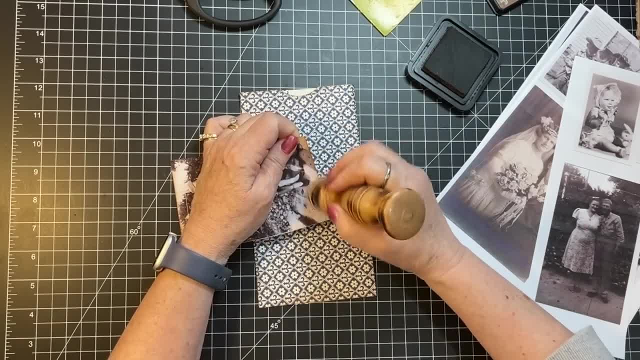 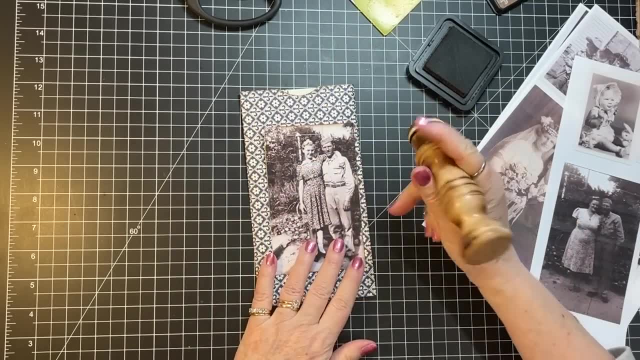 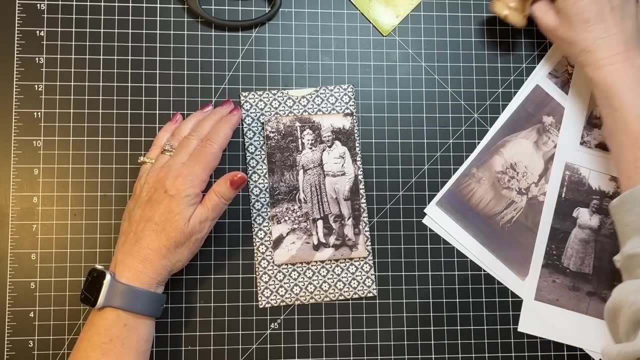 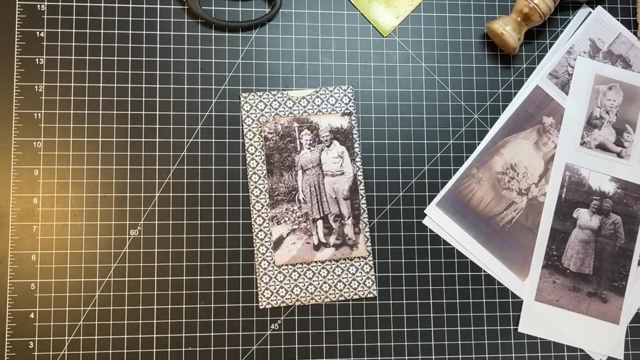 I don't, I don't, I haven't experienced that yet. but Okay, I think what I might do is kind of put this over to the side And I want to put something here And I was also thinking: wouldn't it be fun? 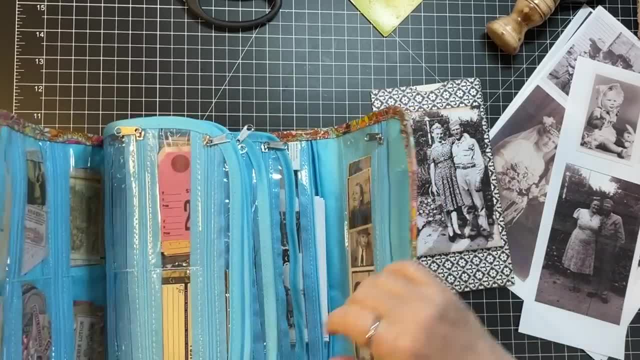 I hope they're in here, Maybe they're in my other, I don't know, Maybe they're in my other. Let me just look. Oh yep, This is what I was thinking. Where are these gauges? But I kind of want a clock. 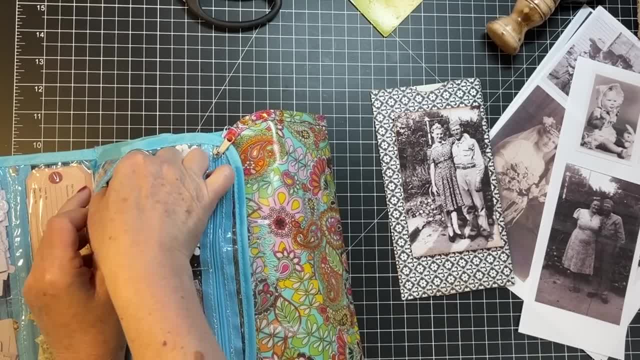 Are these all gauges and not clocks? Yeah, Kind of. Oh, there's one that's a compass That might be kind of cool. Okay, I'm also going to. I think I have Tim Holtz clocks, but they must not be. 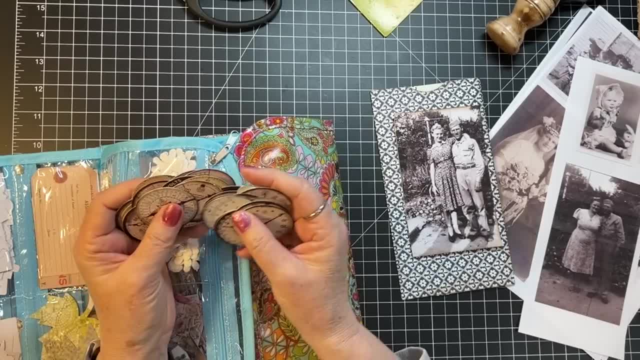 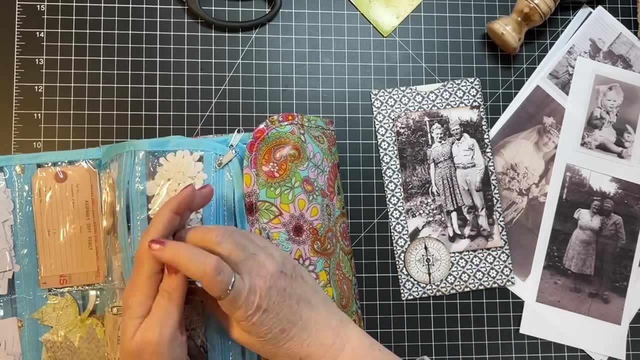 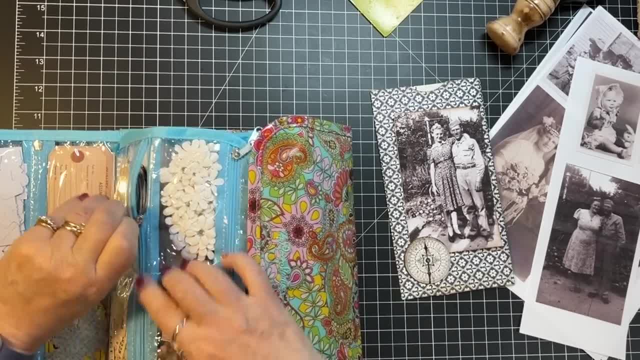 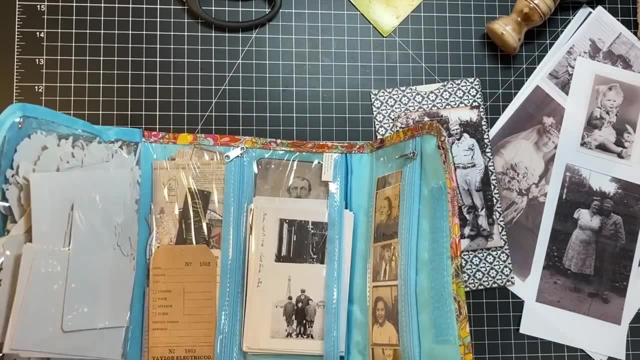 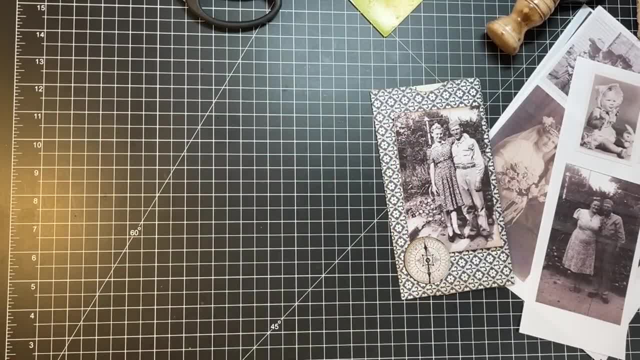 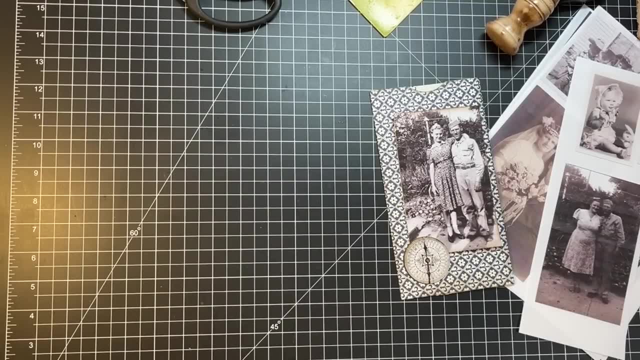 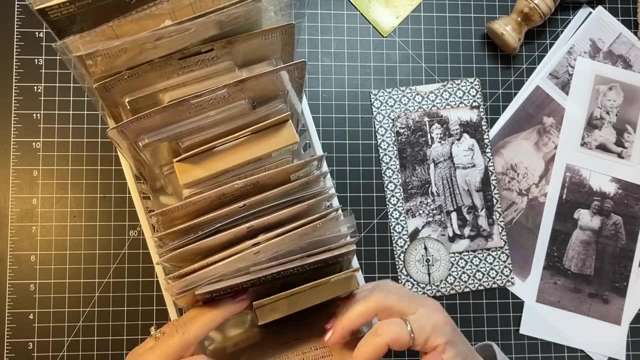 Nope, I don't think so. I think the clocks would be a bit better size, maybe, I don't know. Oh, I cleaned out my. I cleaned out my Tim Holtz drawer and put it all here so I could access it right. 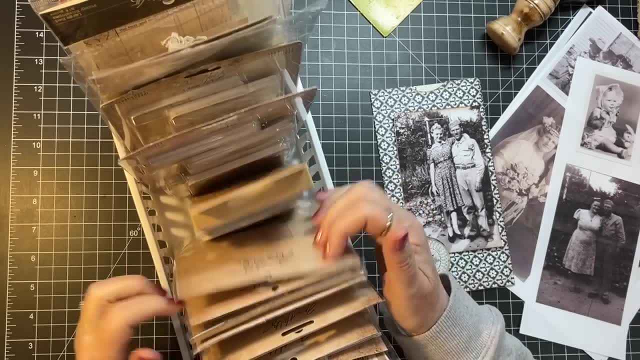 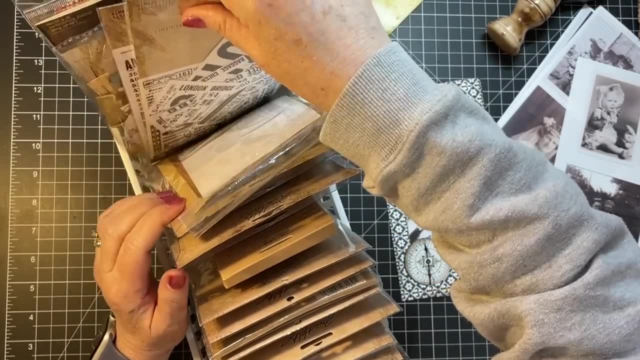 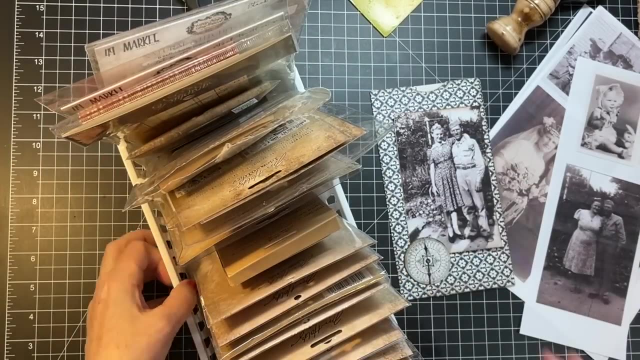 I think so You can. Um, do I have a Tim Holtz problem? I think I do. I'll own that. I do like my Timmy stuff. Oh well, I don't know, but I want that anyway because there's some. 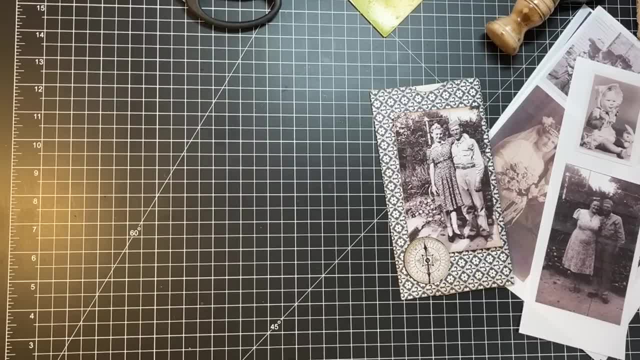 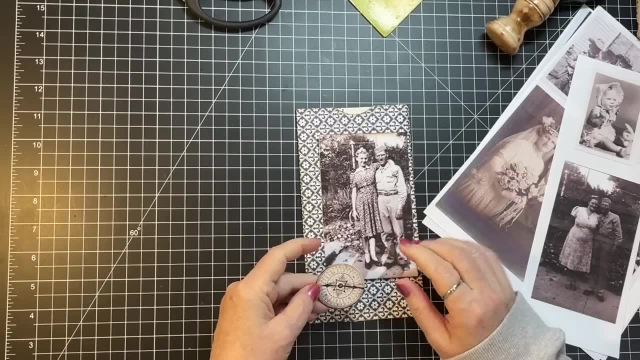 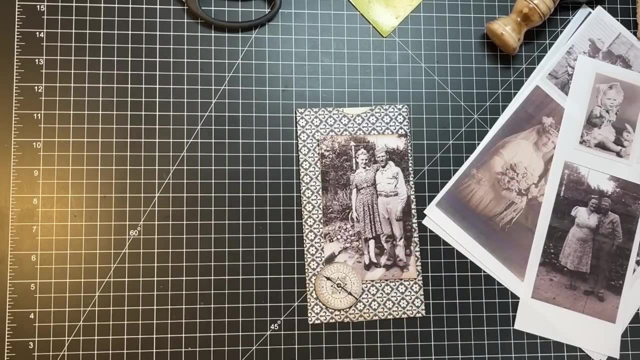 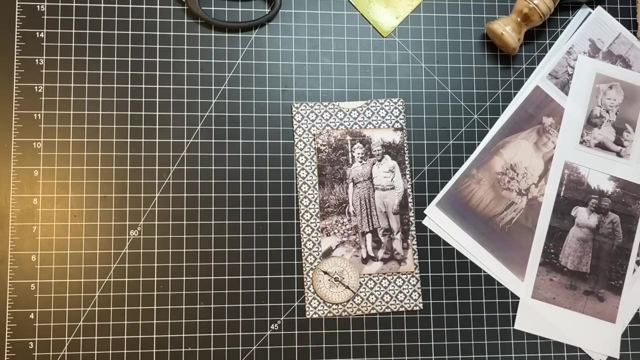 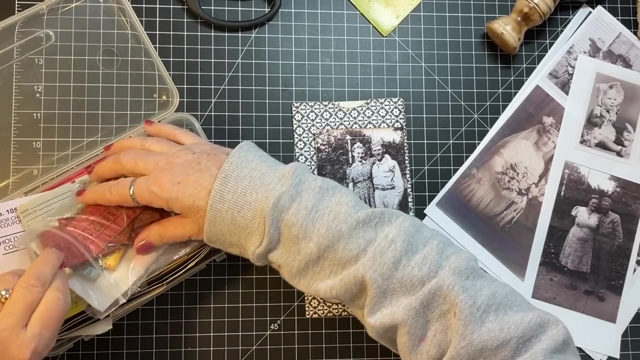 non-Timmy stuff in there I want to play with too, with these. Okay, let's see, So that. but I want, let's see- north, south, east and west. I want something right there Like a ticket or something like that. Let's see. Ooh, maybe, like I don't know if this is too big. 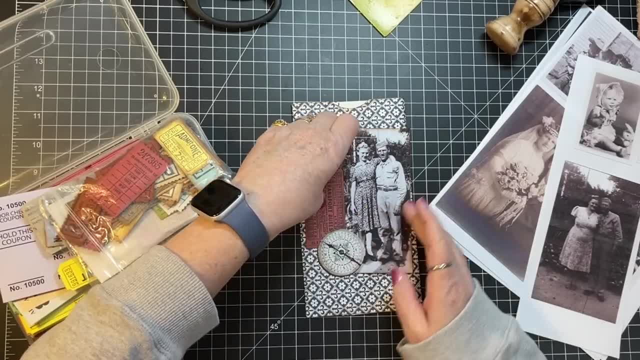 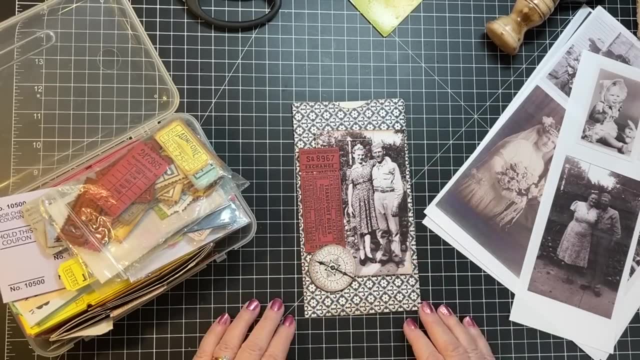 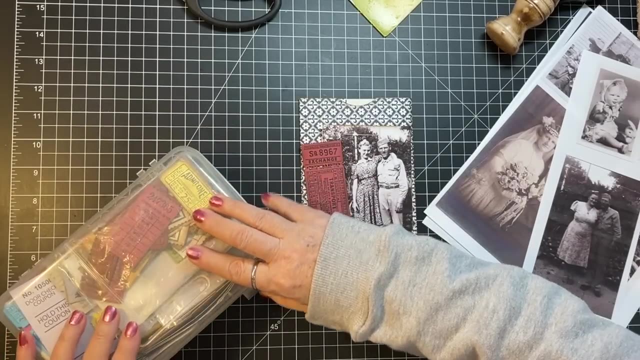 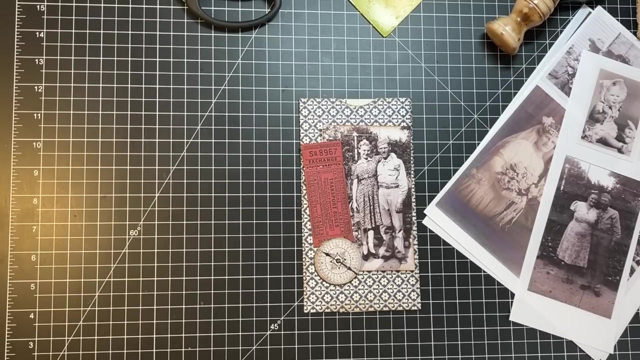 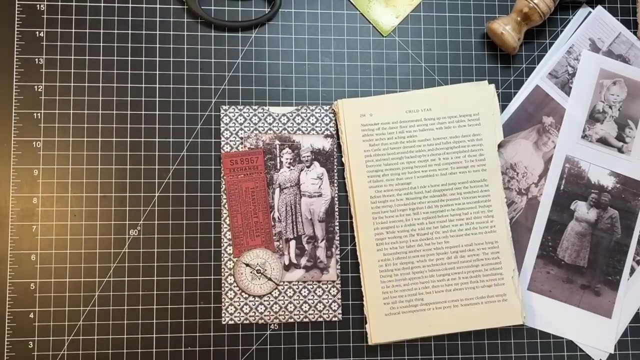 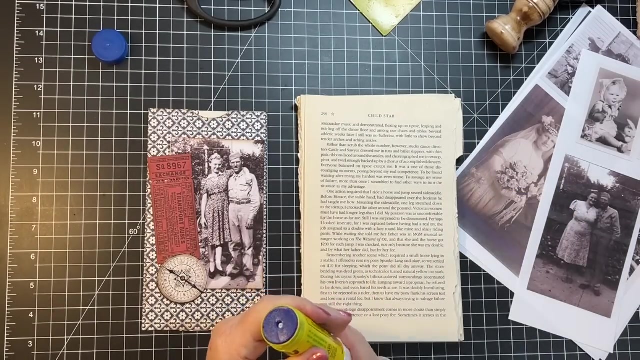 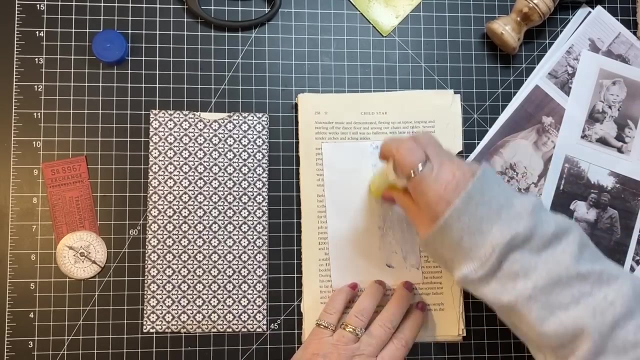 Something like that. I think that's good. Okay, Thanks for being here crafting with me today, Just having a day, Let's see. This video will air on Sunday and we're supposed to be having snow about that time. How's that for end of March nearly and still gonna have snow? It's like 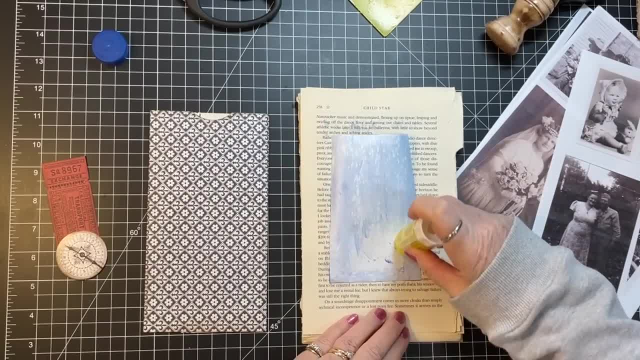 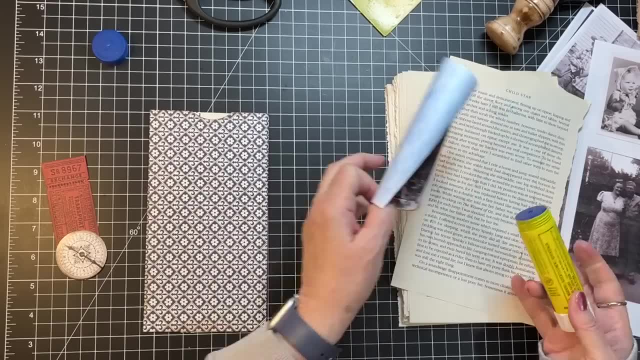 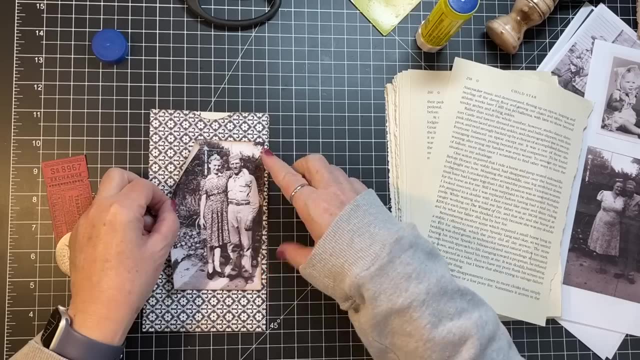 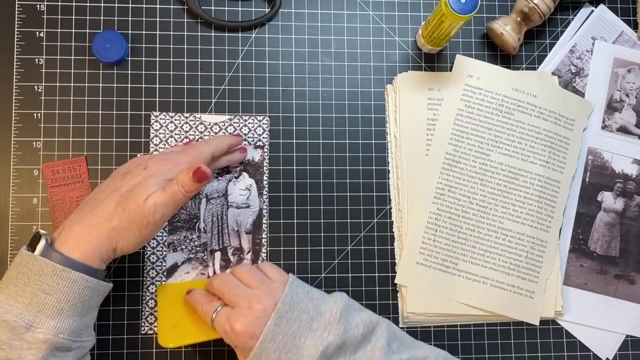 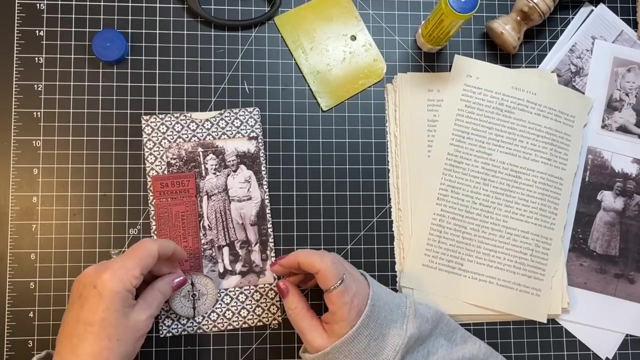 really Gosh. I'm so ready for spring, but got it, I'm gonna get through the winter and we really can use the moisture, So I shan't complain. Okay, And then that kinda right there and this down here: Okay, Art glitter glue, That's what I want. 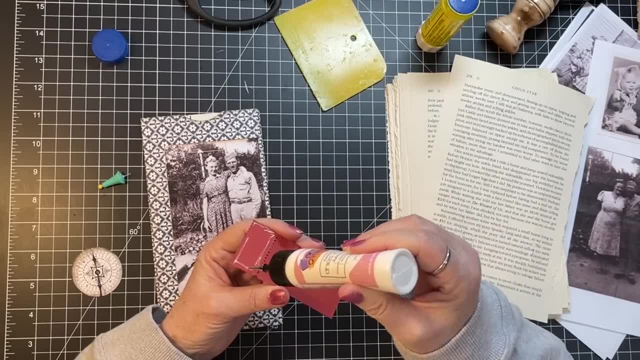 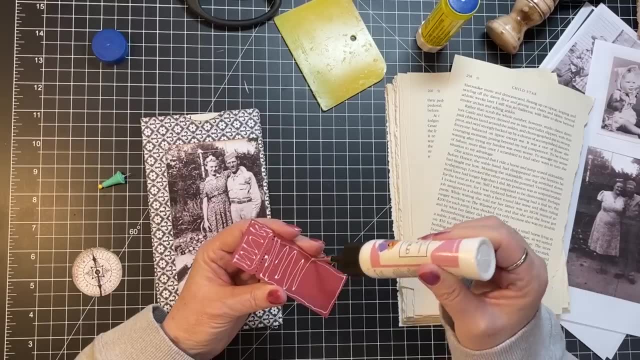 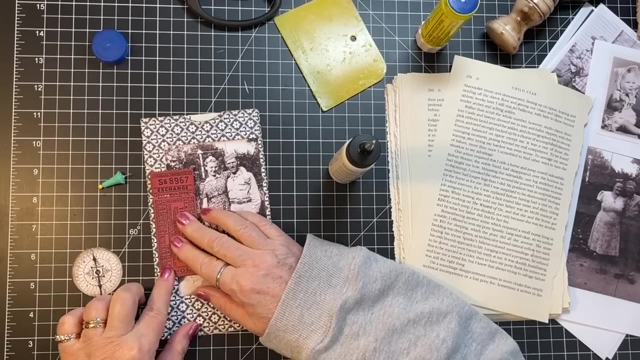 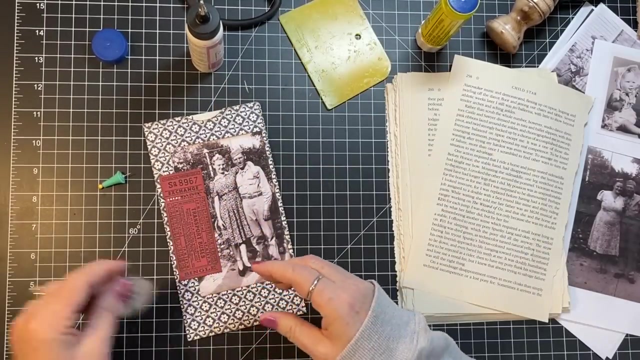 I don't know if you can see it, but I honestly don't know what I want. Thank you so much for watching And I look forward to seeing you next time, guys. Bye, Okay, And look at that, We'll have another piece of ephemera. 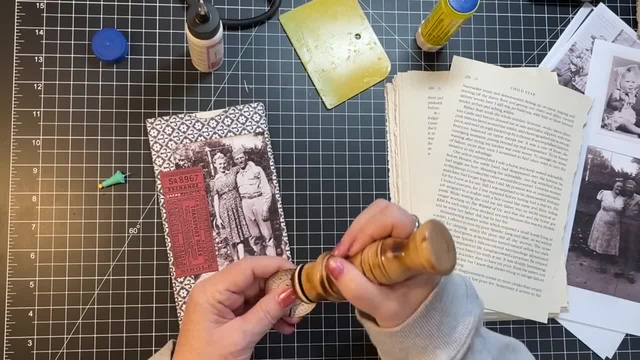 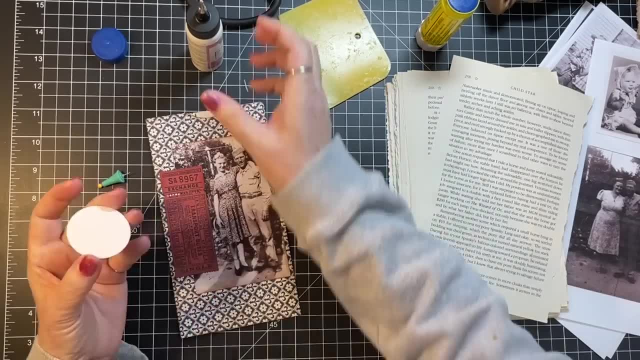 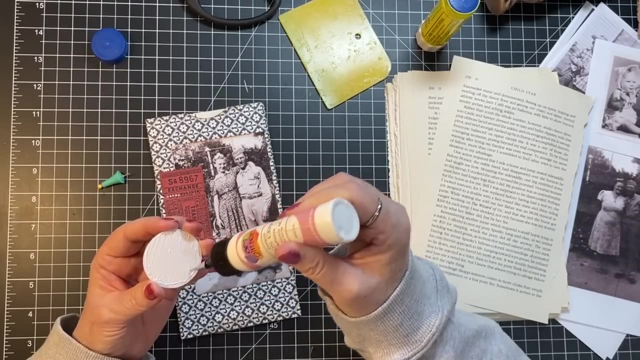 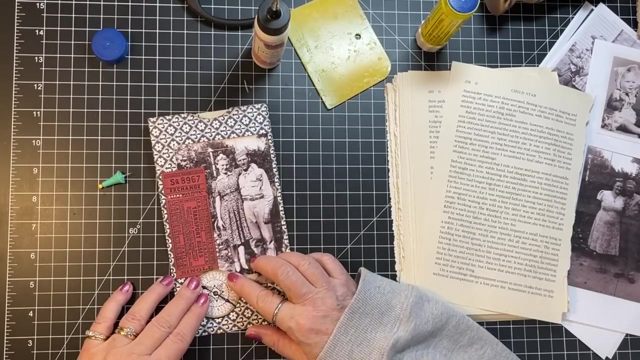 Another piece of ephemera. Another piece of ephemera that is all decorated can come out of the to-do box. you know, I've been kind of working on that a little bit, trying to pare down my to-do box. so yeah, we are, I'm doing some videos and then we're gonna watch little March Madness later. 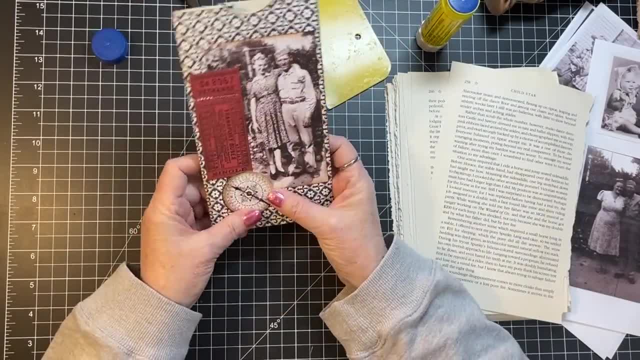 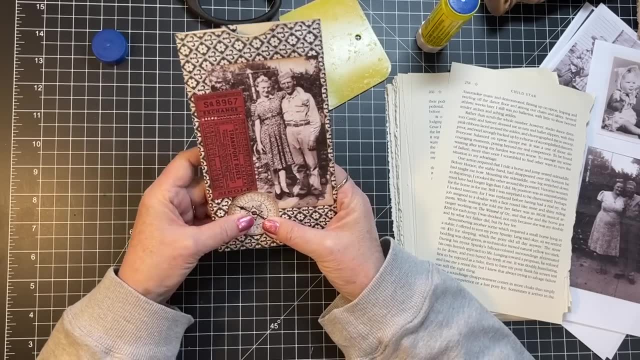 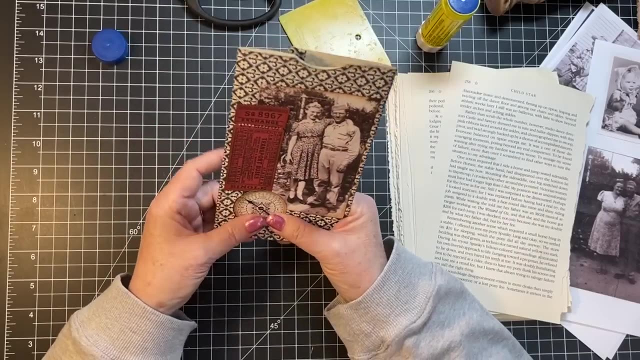 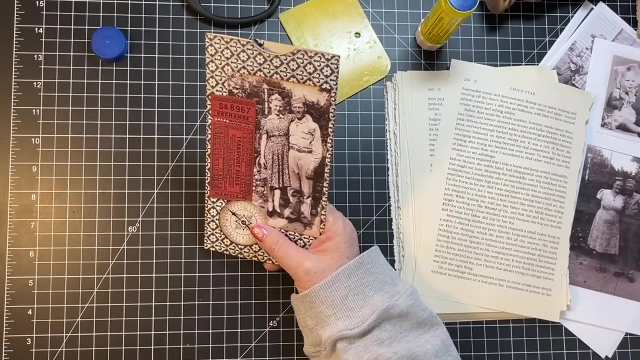 on this afternoon. okay, I'm liking that. what would we like to do on the other side? I don't know. I don't know. I'm kind of I'm looking around at stuff here seeing if there's something that jumps out at me that needs to go. whoops knocking things. 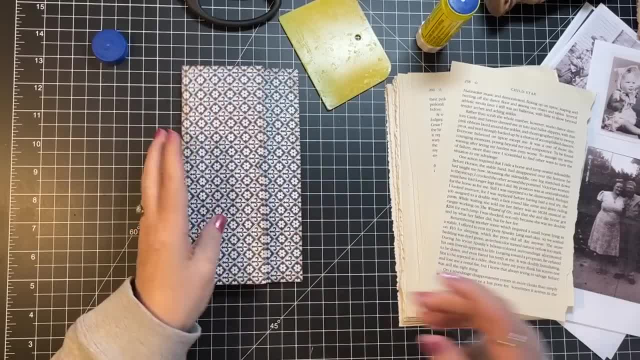 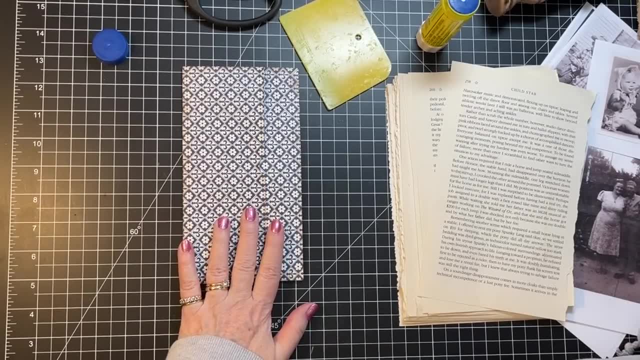 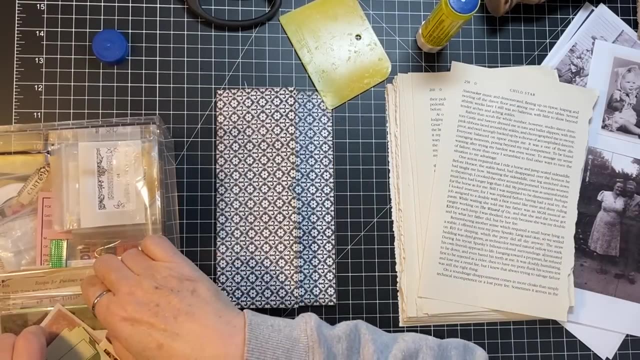 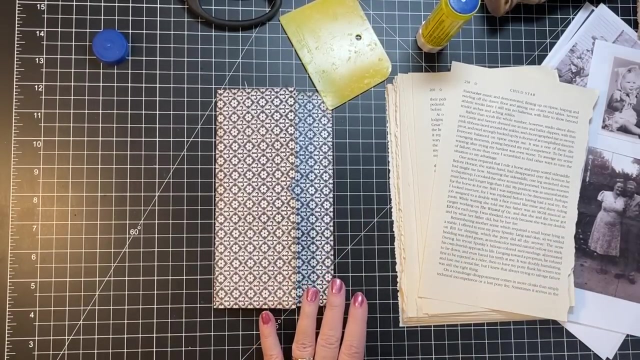 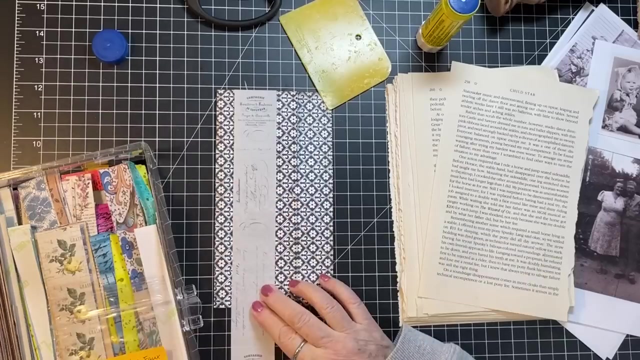 maybe a thick piece of uh washi. I haven't done my sewing on that's not washi. I haven't done my sewing on the pages we made yesterday so I can't show you those. but I was wondering if we have something kind of thick that might be nice on there. let's see. I've got. 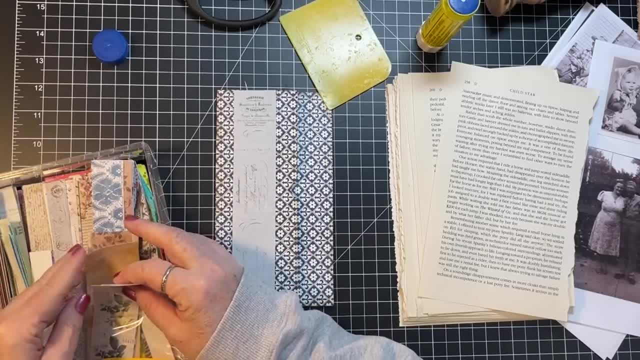 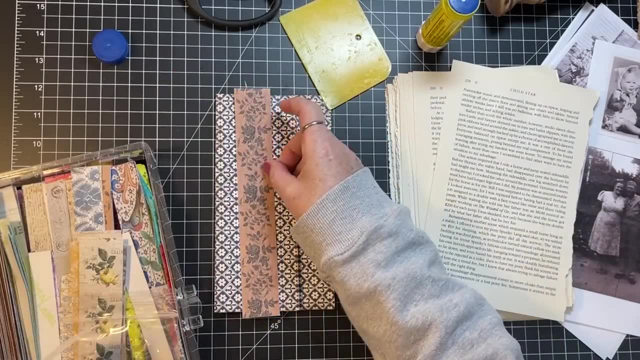 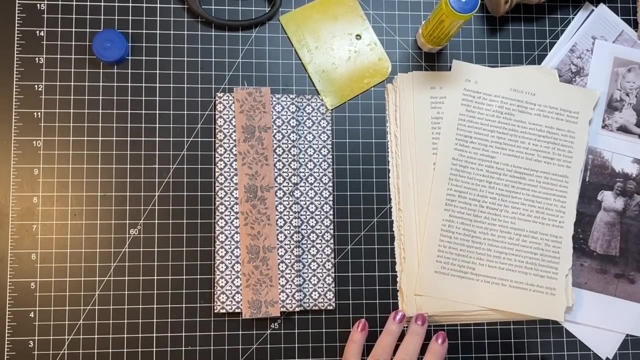 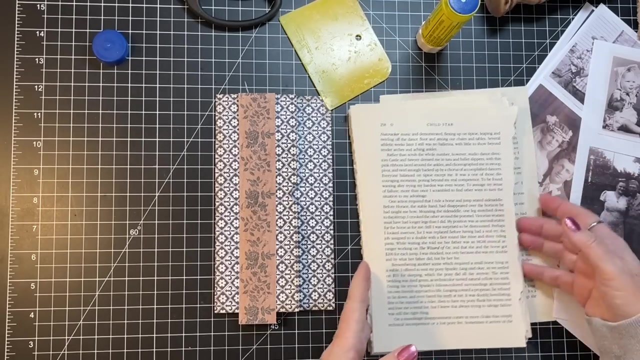 some here as well. oh, what that looks like on there. oh, I like that. let's do that. that's from Paper Baker Creations. so, and I'm my plan is tomorrow. I don't- I don't really have a have an idea what I want to do for mixed media. 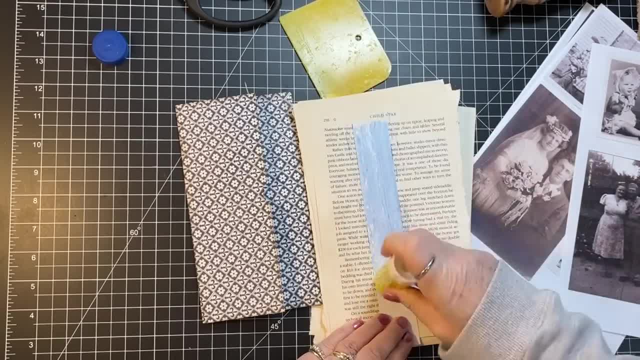 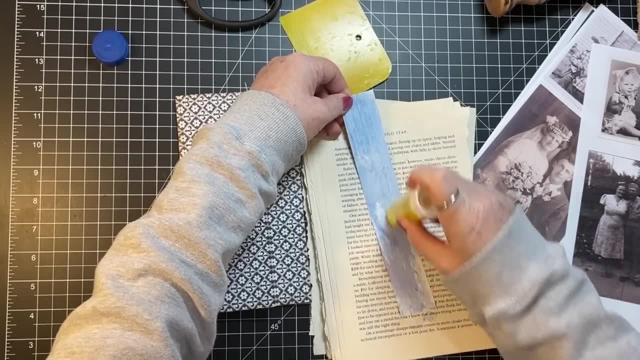 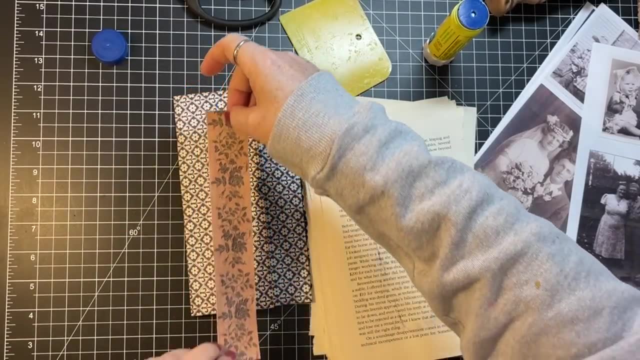 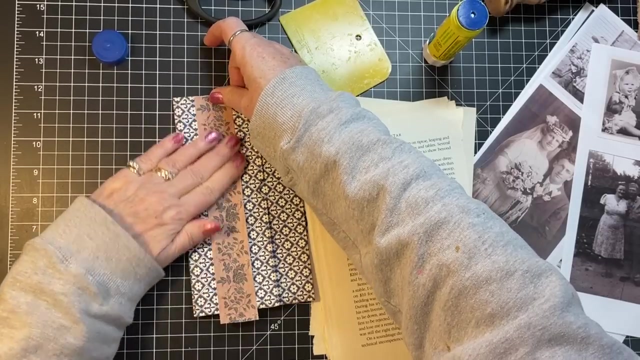 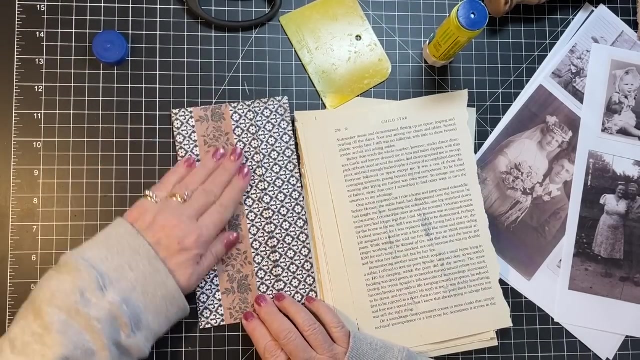 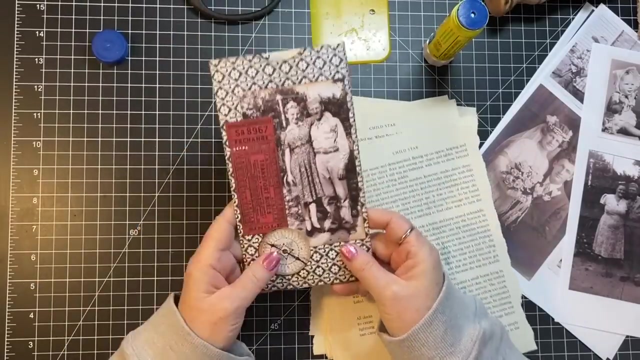 Monday. so I am in need of the vintage looking um decorative tape, and so I think I might do that like that. I'll just flip that up and over. okay, that's nice. okay, I'm gonna call that decorated. but isn't that cute with that little couple. 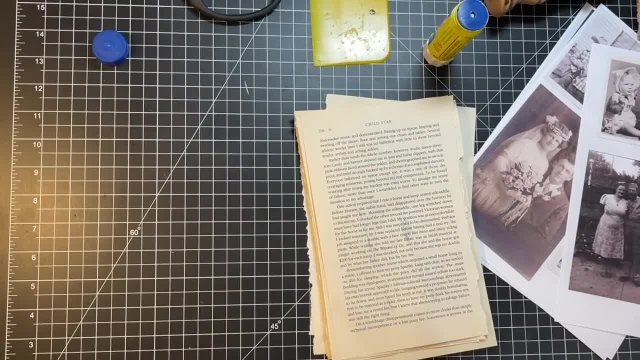 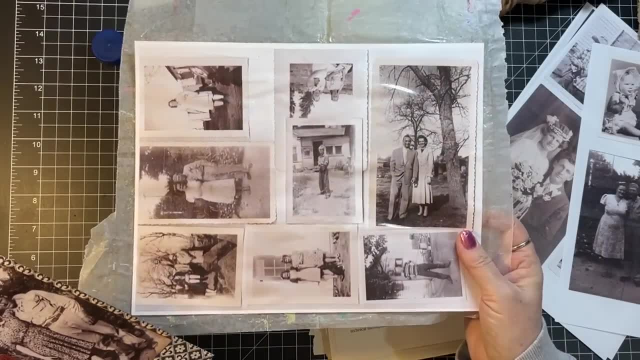 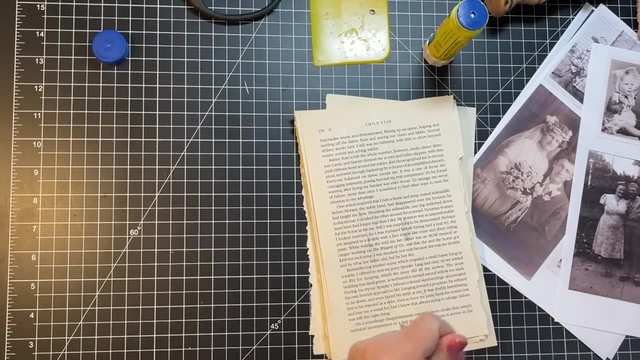 I love that. all righty, then let's how's my okay coming along? oh, I think it's gonna work. look how shiny. they're kind of bumpy, but that's okay, I'm not worried about that. okay, what else did I want to? oh yeah, I wanted to do this. 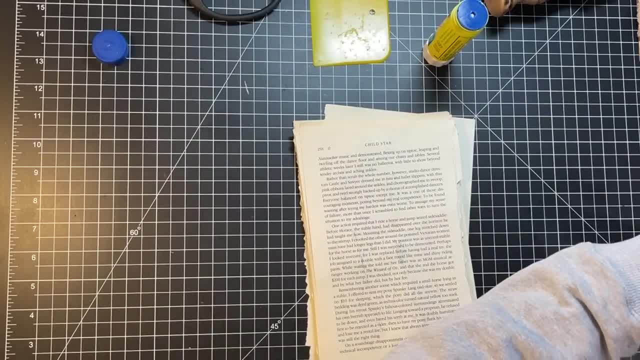 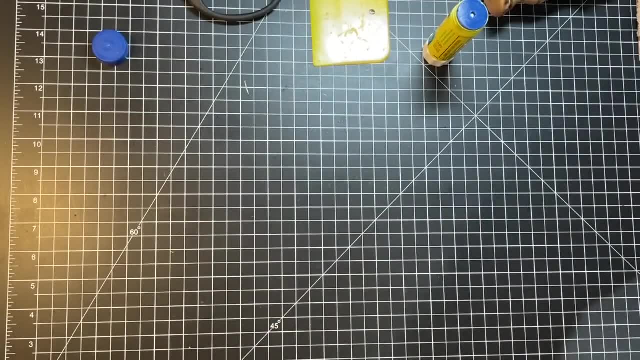 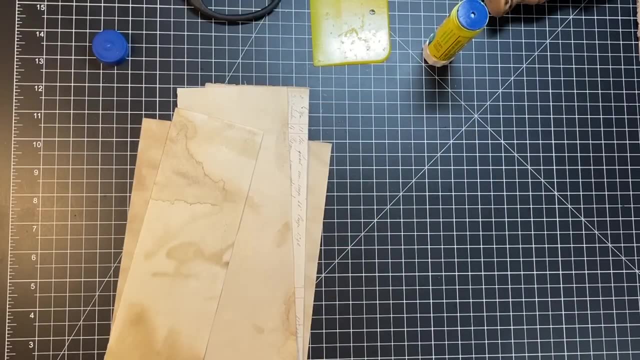 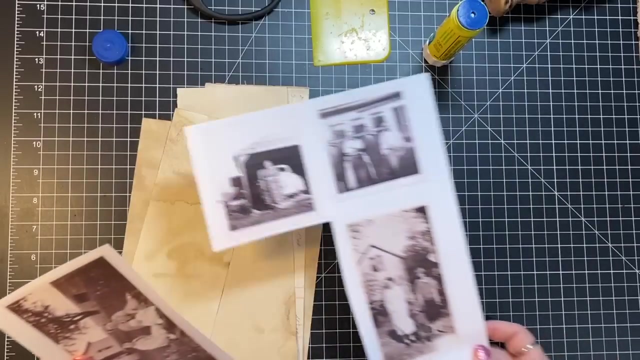 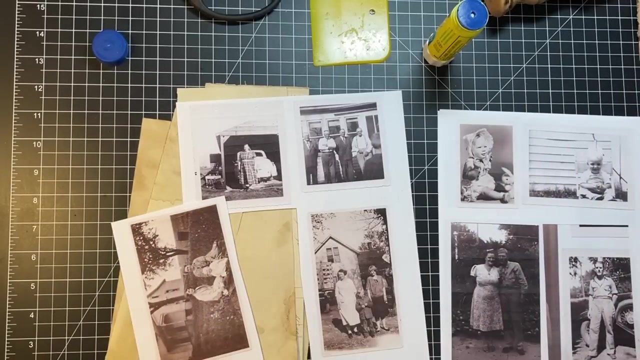 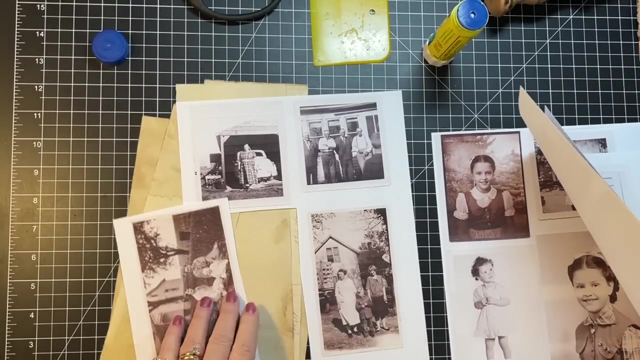 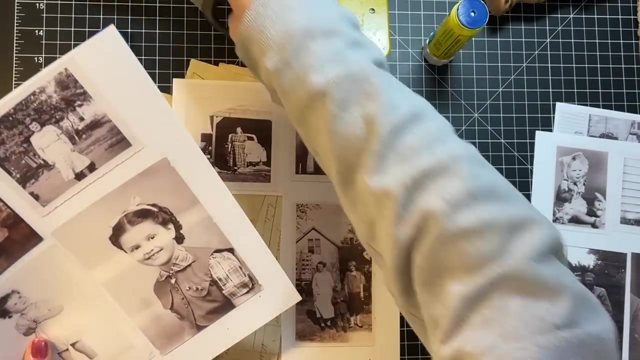 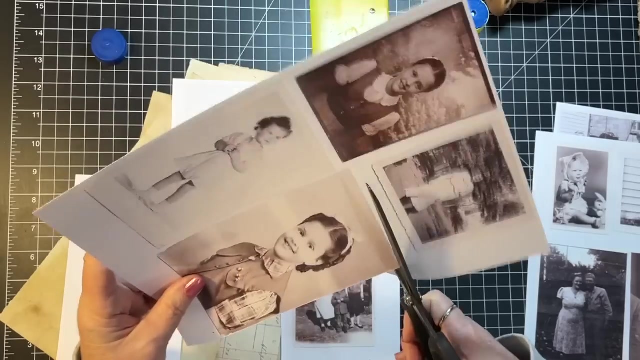 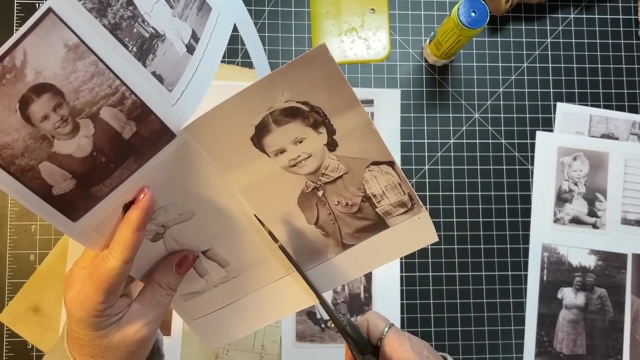 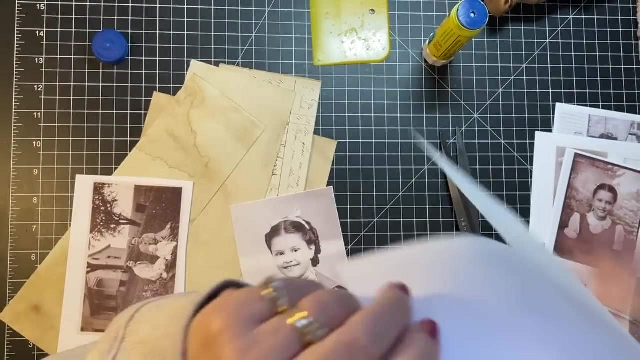 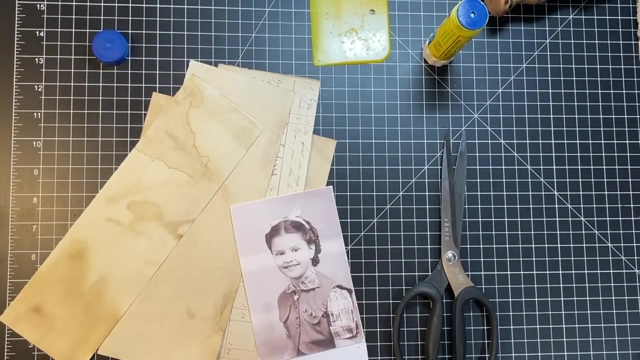 so let's move a few things aside so that I have room. but I was thinking might be kind of fun to to like do um a little, um like a notebook type thing, use this for the cover. why does that? I maybe could use her all my bits and bits. I don't really want to um cut them out though till I know what I'm. 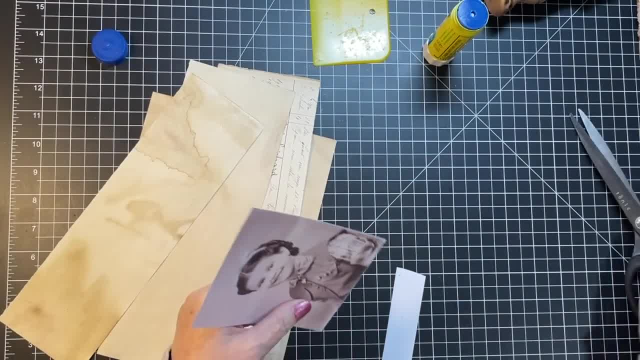 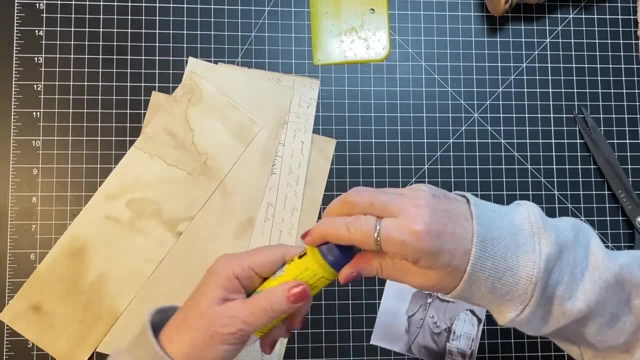 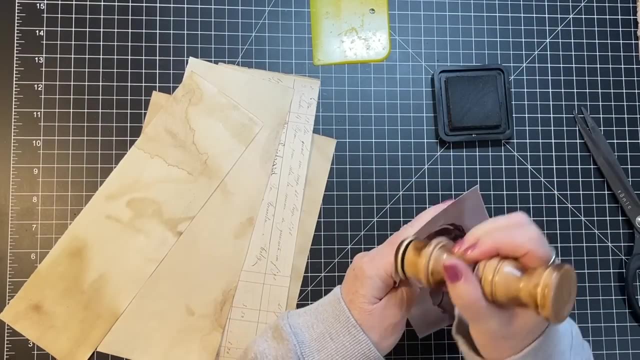 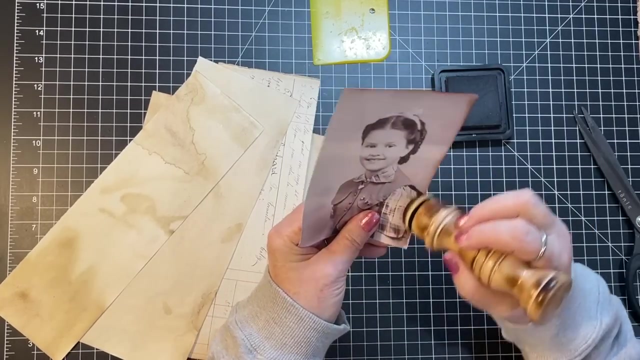 what I want to do with them, you know, okay. okay, little girl, see, I'm done with that, I think, yeah, I kind of kind of got some bits and pieces out and prepared for my video before I called my brother because I didn't know how long we would chat. but 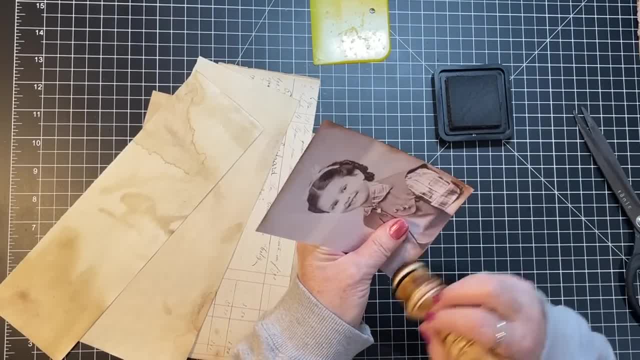 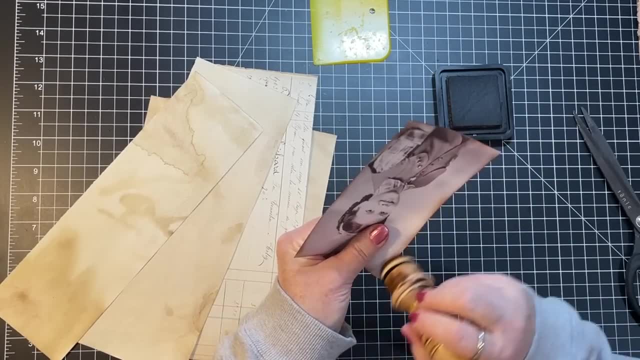 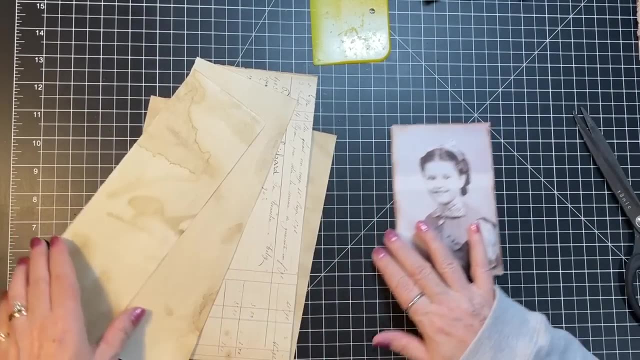 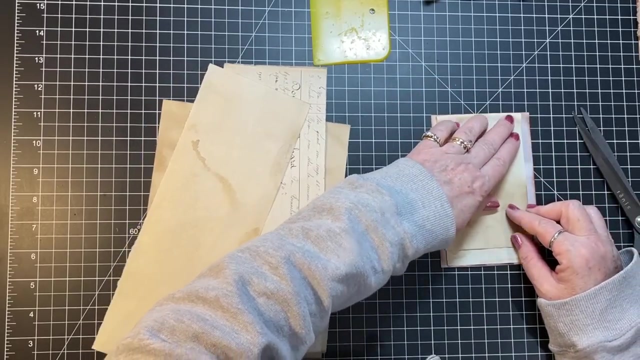 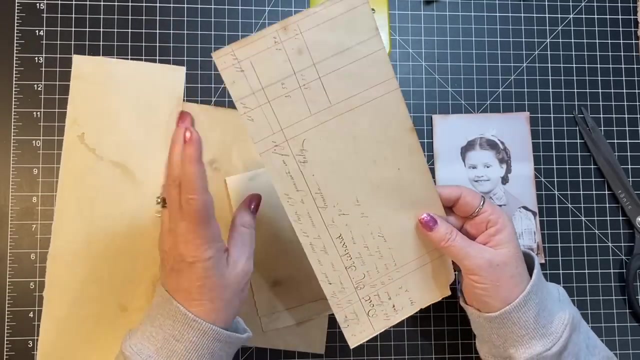 he's. he's my husband, half brother, and he's 12 years older than me, so but doing pretty good. you know a few challenges along the way, as we all have. okay, just fold some things. this is cool. I thought I had this as a scrap and I thought: 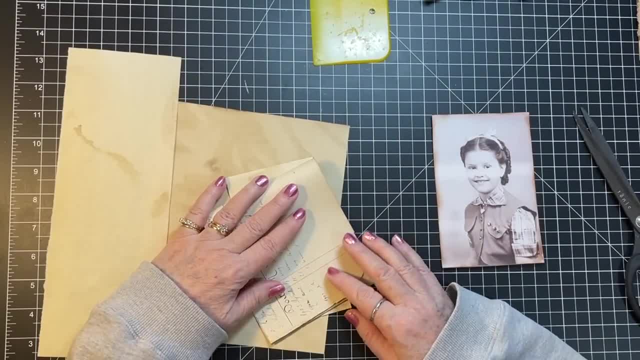 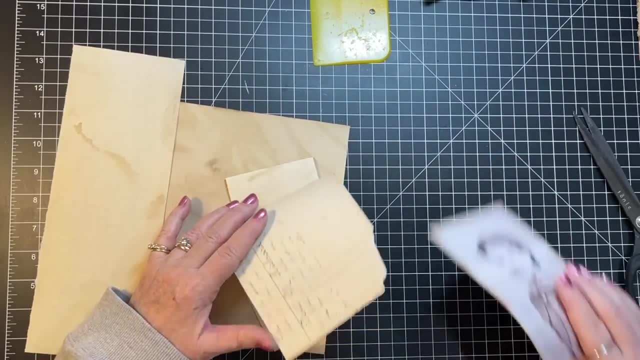 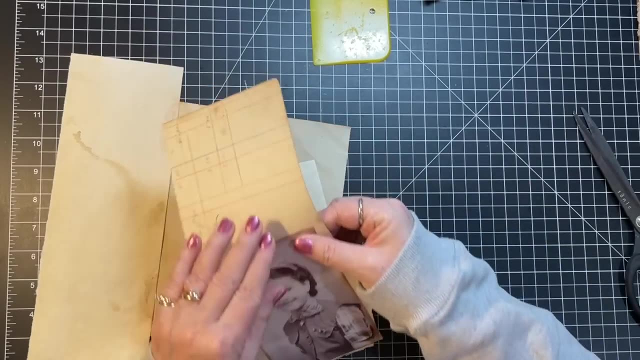 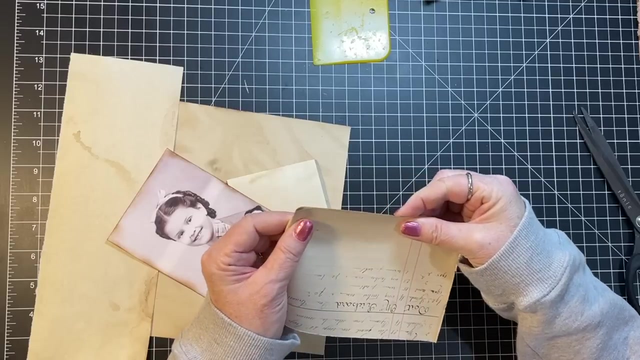 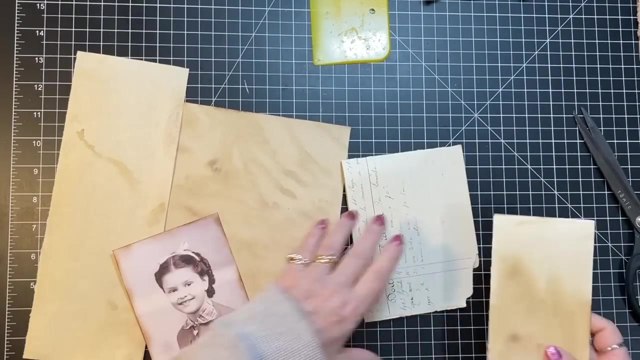 that might be kind of neat. yeah, that's gonna be cool. okay, so I think I want this to be as long as her, maybe a little bit longer. so fold that right there. I'll just use the edge to theoretically fold it straight, okay. so then in there, let's put this and this: 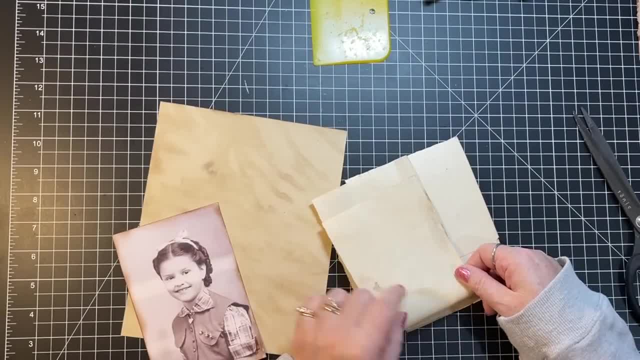 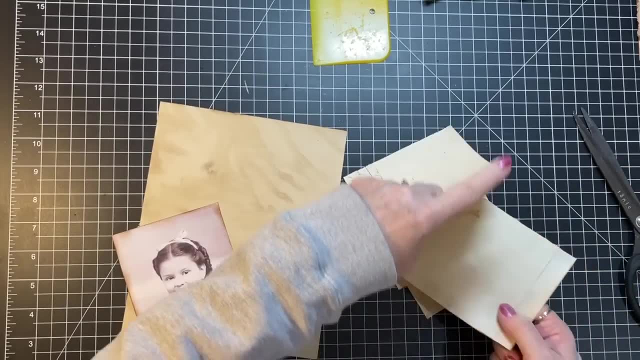 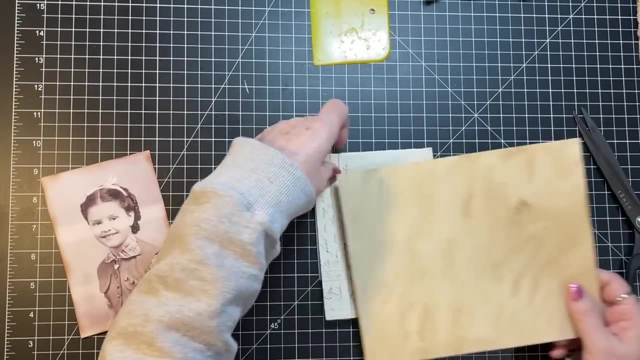 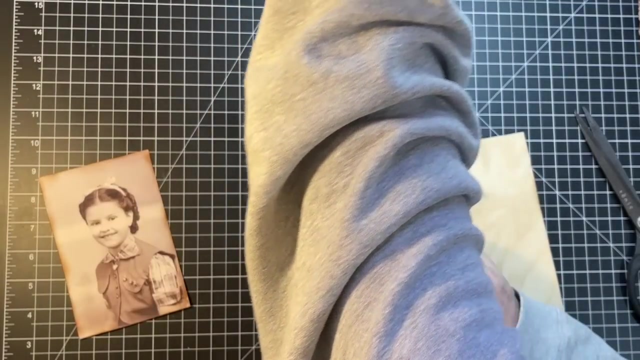 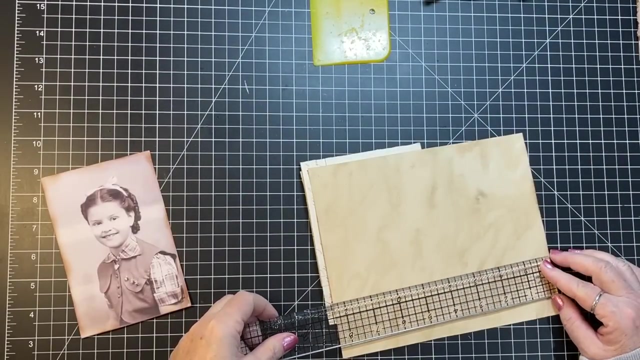 I don't want it any longer than that. okay, put that in there, a couple of scraps of coffee bag paper, and then maybe I can do this just a little bit longer, and then, whichever one looks your best, you're gonna have eight and a half, so go four and a quarter ish. 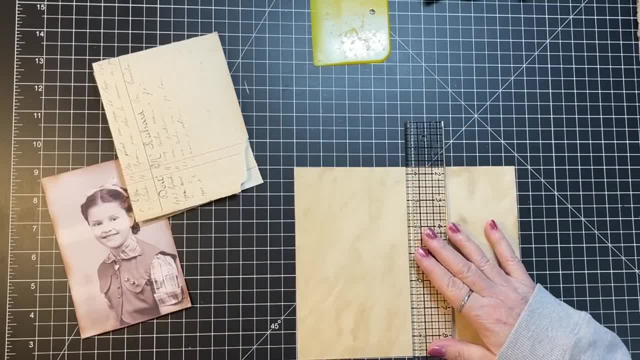 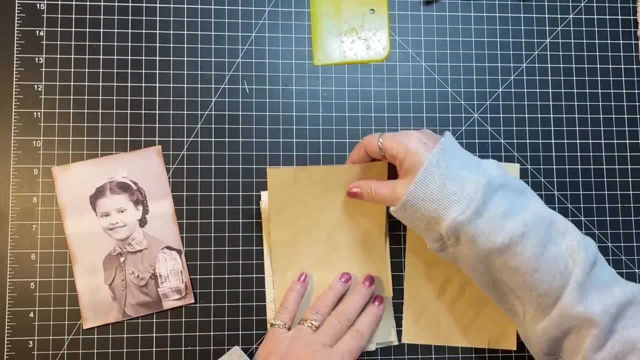 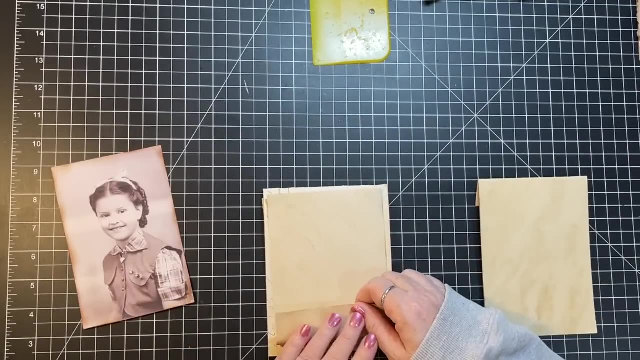 and this one's gonna be just have a little little lip at the top. wait, is that because of the discord? yeah, that's what it did, and it finally fits me okay. so there's a couple more things I want to show you. okay, I think I'm gonna just cut. 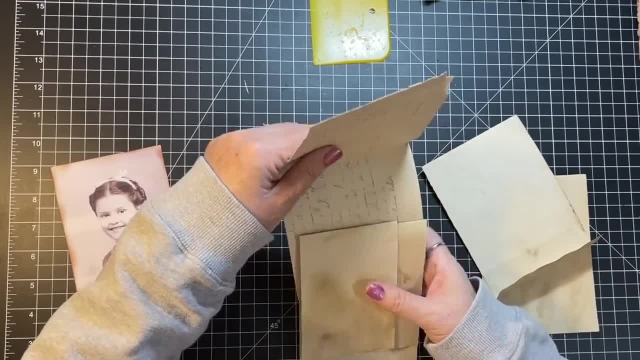 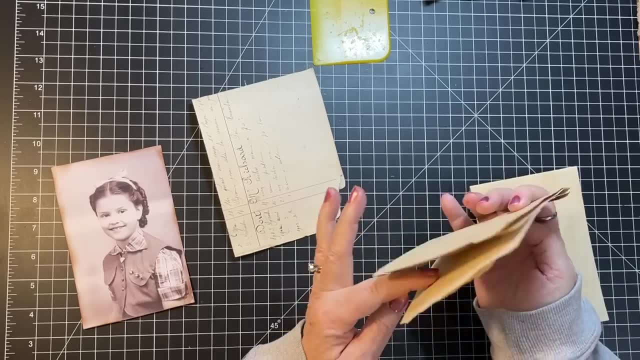 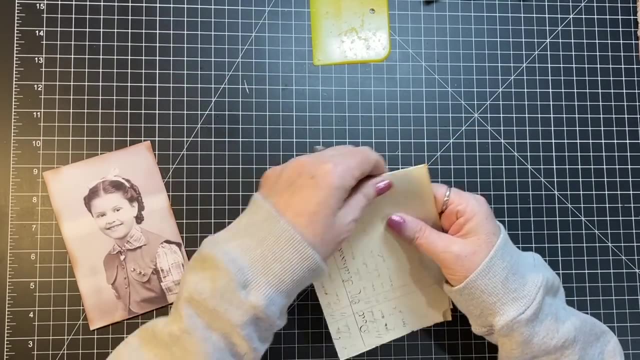 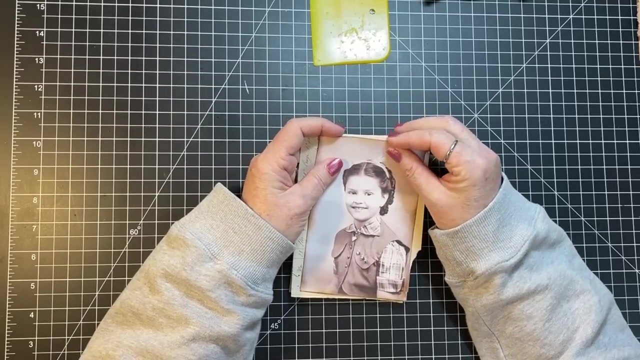 okay. so I think I kind of need to cut this one a little bit longer so I can do this like that. Okay, So I'm going to go like that, that, that, and then I'm going to go like that, put that together and then put that there and put her here. What I was, let's. 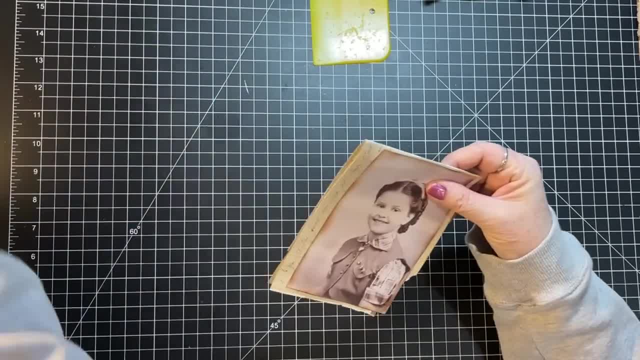 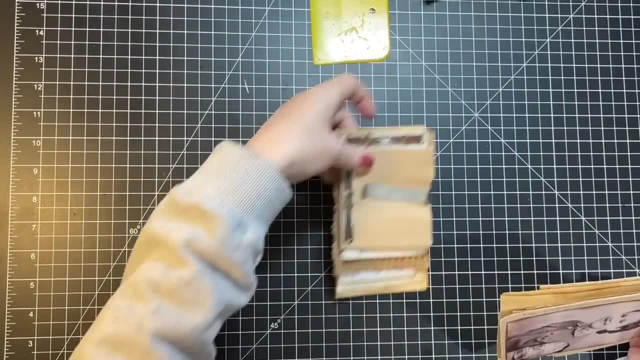 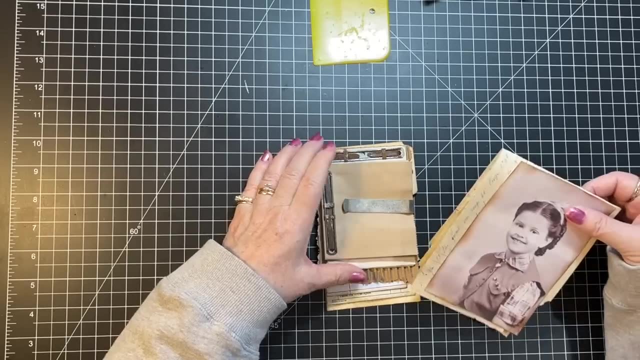 see how wide is that? Oh, that's good, That's going to fit on a page just fine. Okay, What I really wanted was I wanted like one of these. I've just put an order in for rust paper scissors again, cause I love their stuff, but I don't have one of those. So I was thinking would 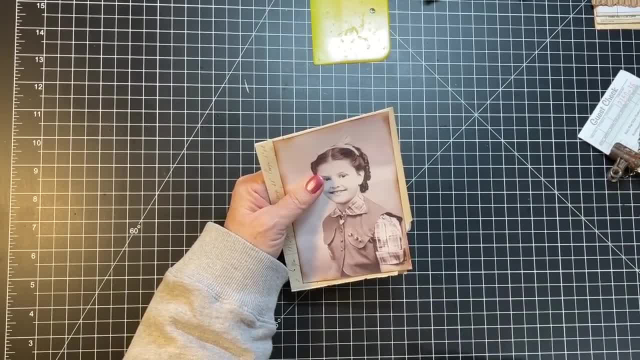 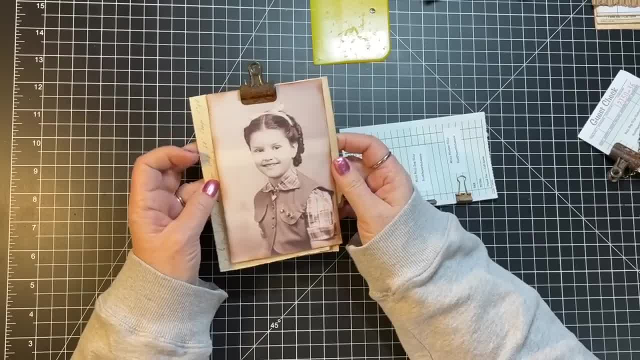 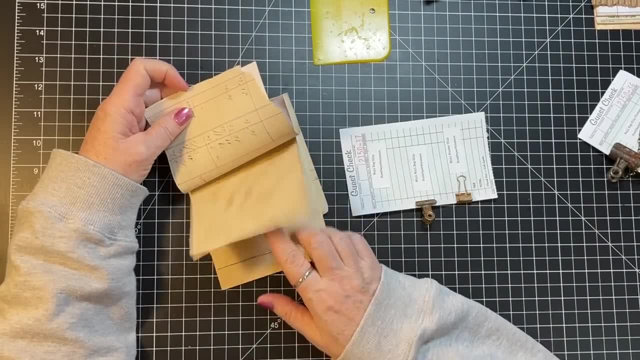 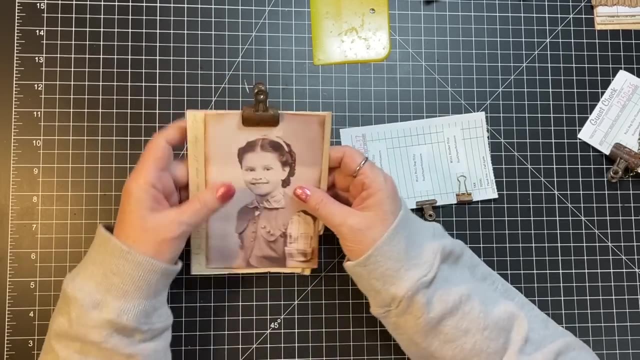 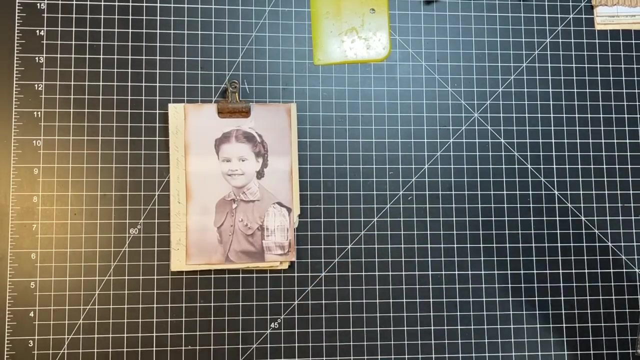 One of these at the top and that can just slip into a journal, have lots of writing pages, lots of sort of variation in sizes, and that's fun. So, yes, yeah, Rust paper scissors. I love her rusty bits So I'm going to do that. That's another fun piece. 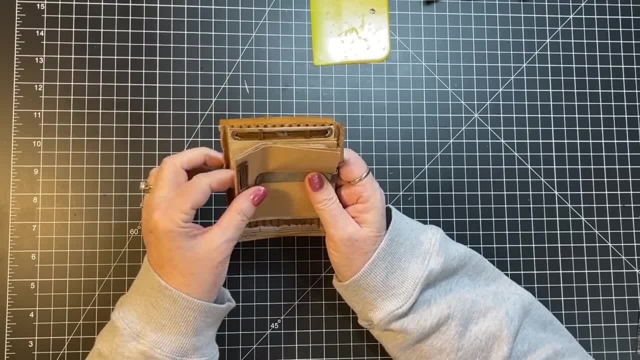 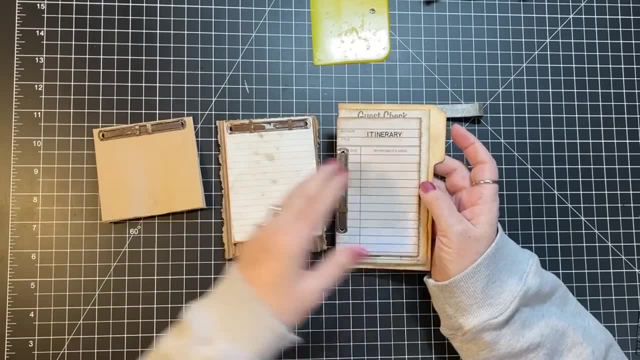 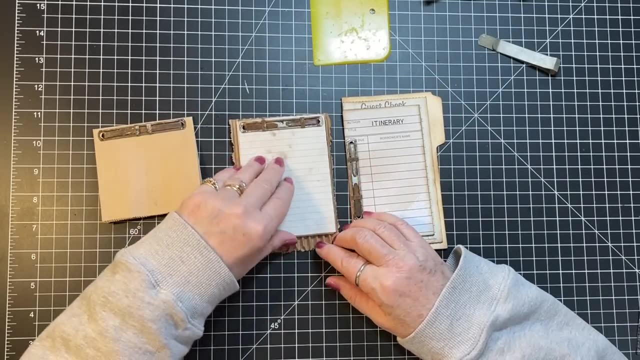 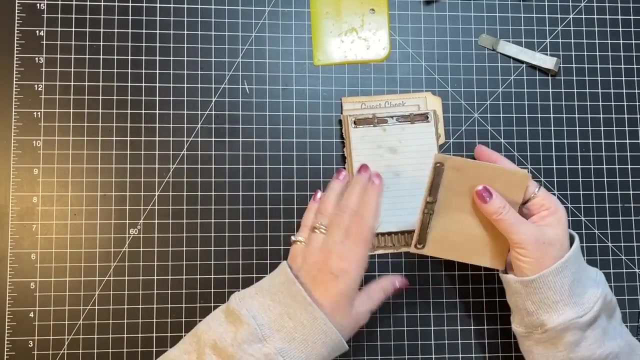 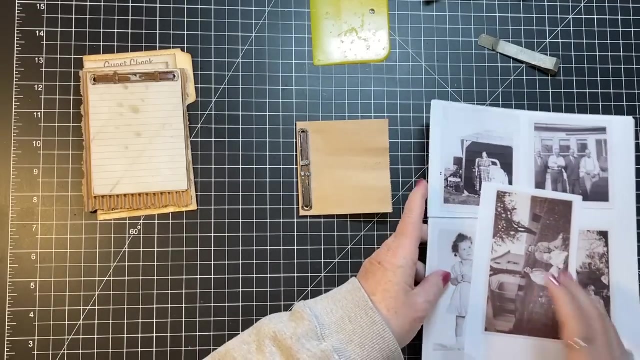 Then I was looking at these, these um she had sent me when, when she sent the um, uh, when she sent the Etsy share, and I love how this stacks up, how she made this stack up. but I was thinking, do I have a picture to go kind of on there? And I think I think our, our baby would work. 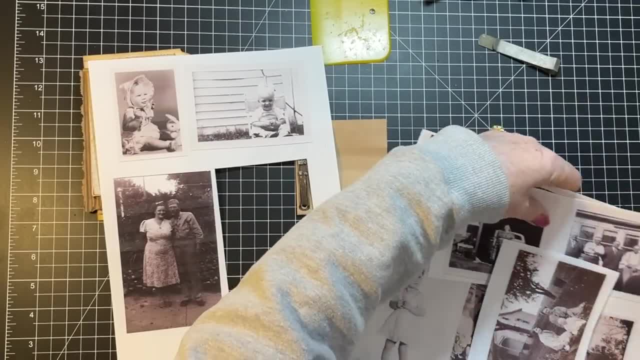 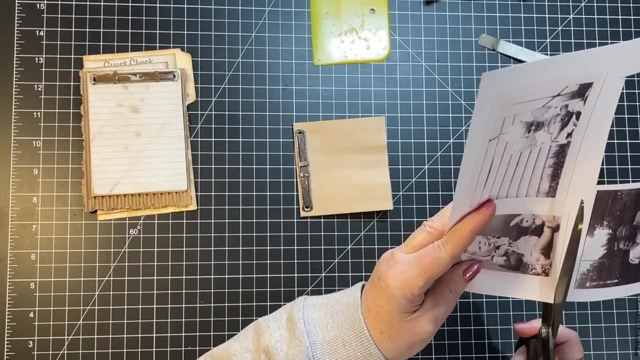 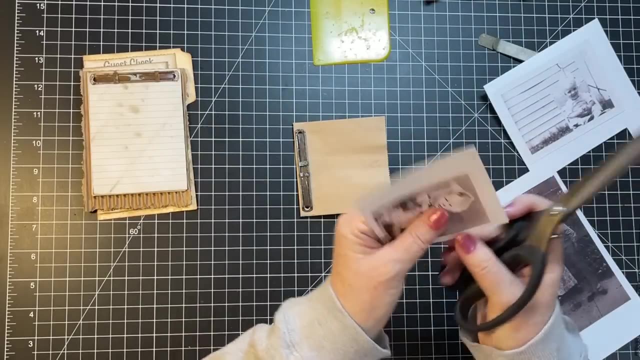 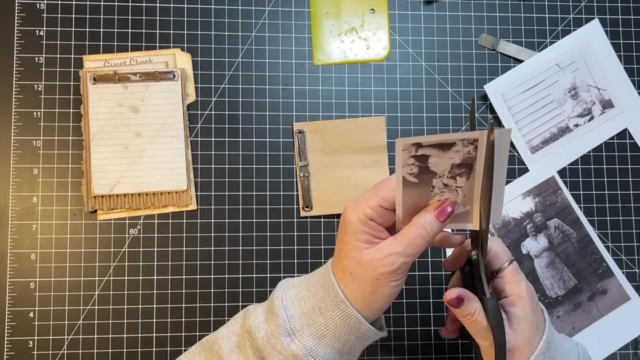 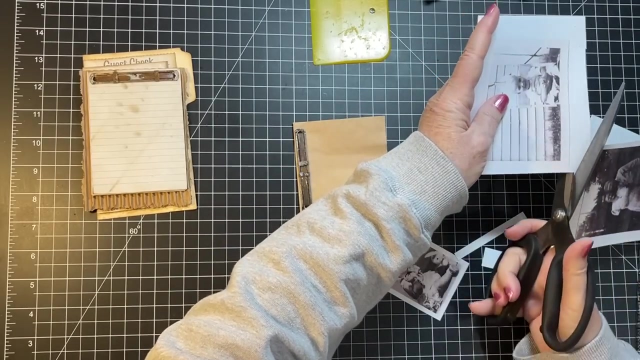 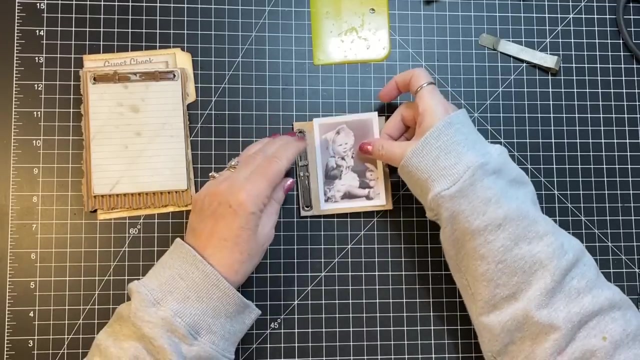 Yep, Okay. So I'm very happy to be playing with this, because you know what's the good of having it all printed out when you're not? you're not playing with it. So, oh my goodness, if she isn't perfect on there. 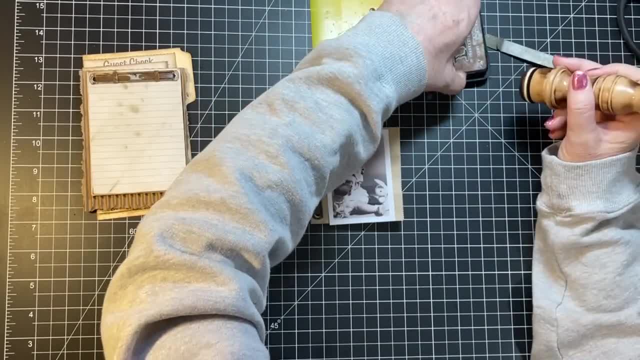 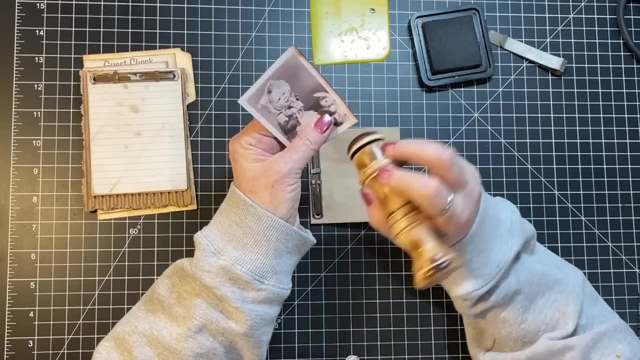 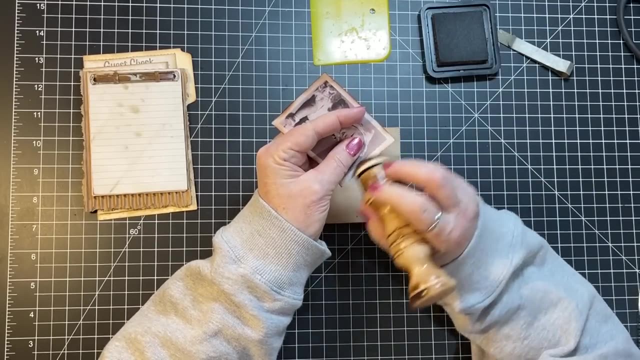 So cute, So cute. Okay, Let's, I'm going to grungy her up a bit, and a bit more than normal, because- because, with the rusty bits and everything, it's all so grungy, So I'm going to do that. 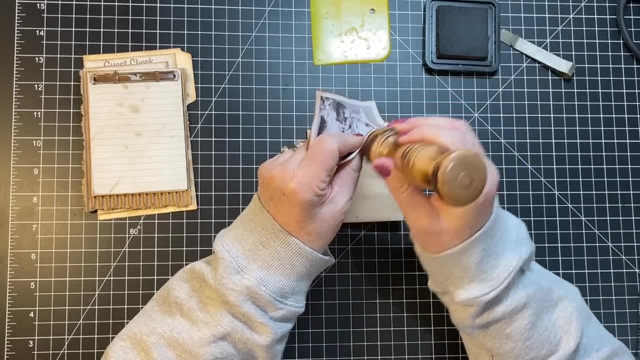 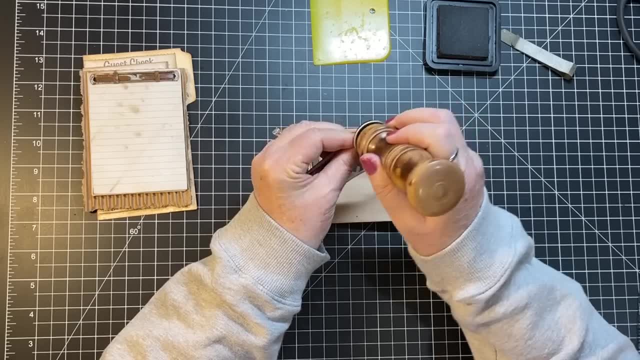 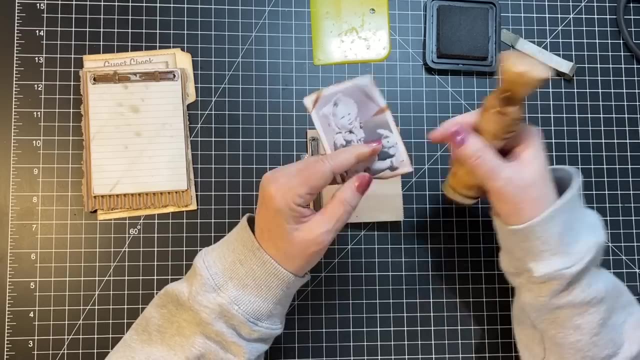 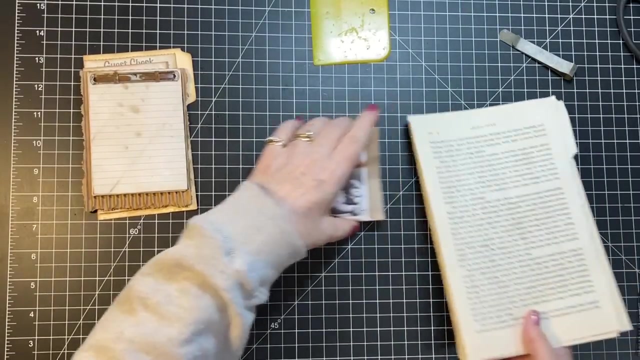 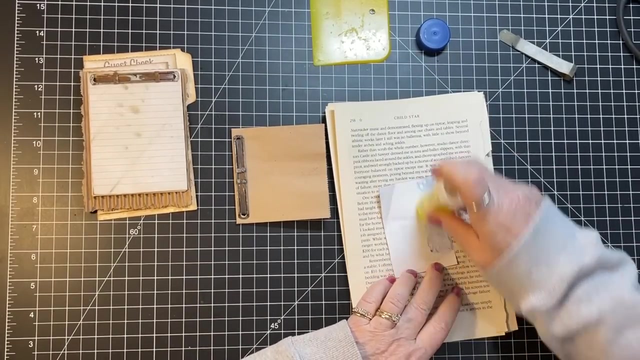 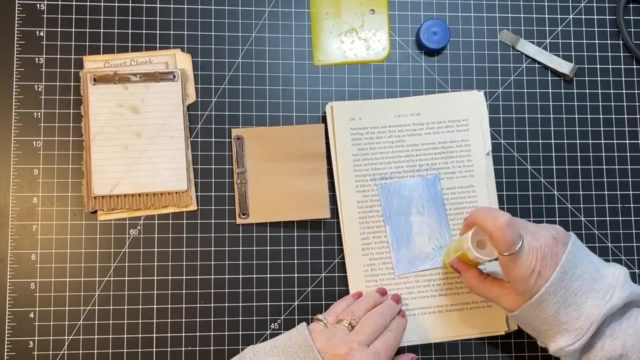 And then I'm going to just put a little, a couple of creases in it. There we go. Okay, Let's just get her on there, Just easy peasy to just glue, stick them on there too. So yesterday my friend Lynn came over and we had a great time. 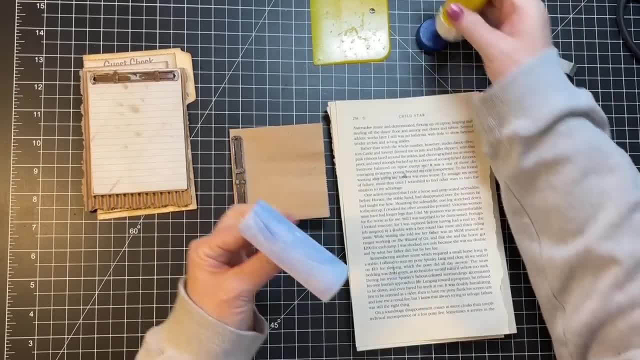 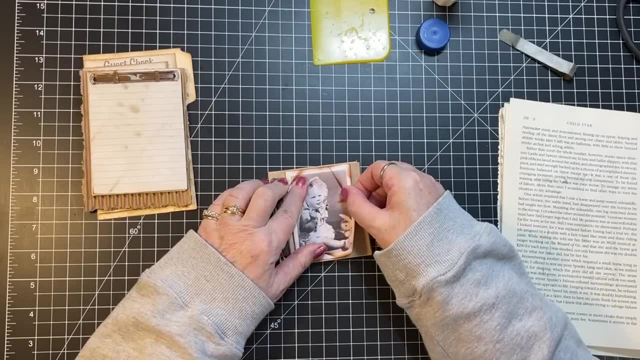 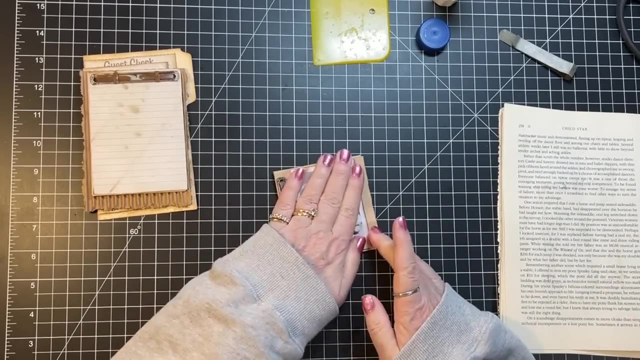 Oh my gosh, She's just the best. I love her so much And, oh, I missed her while she was gone. So we got together, We had a big play. It was a fun day. So she's working on a slow stitch journal cover. 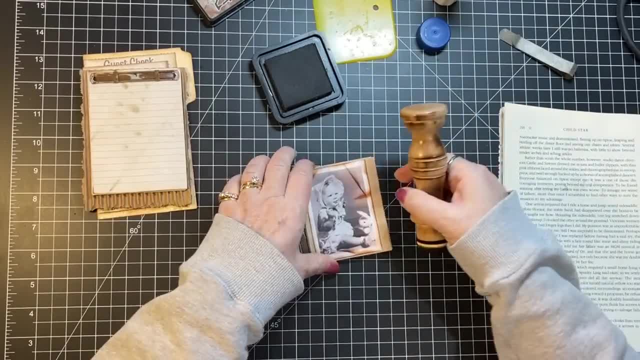 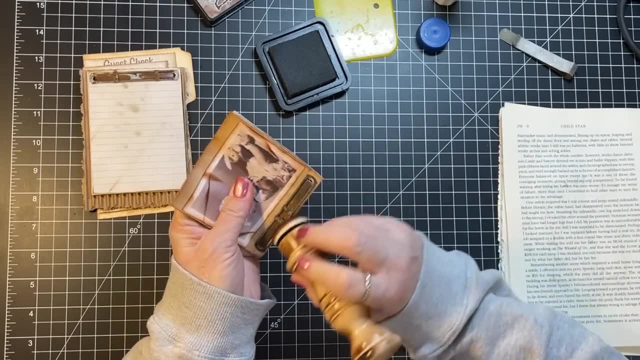 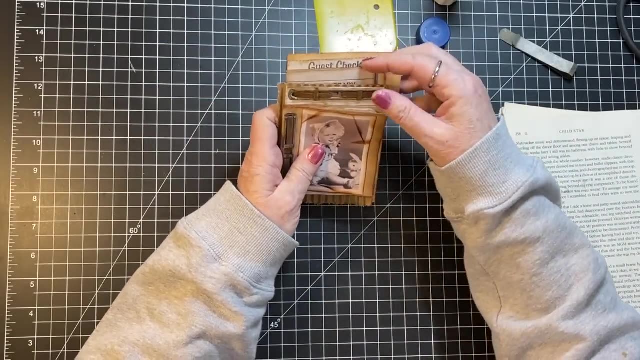 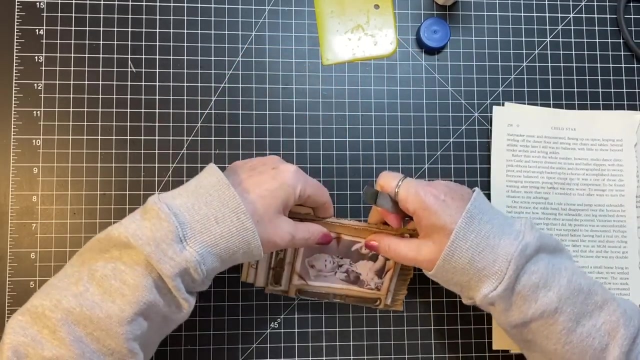 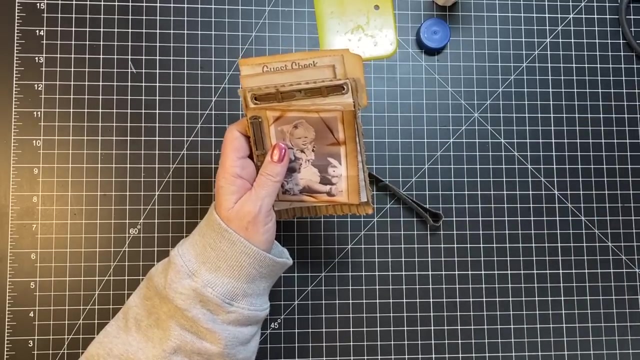 I did fussy cutting, which is going to come in handy here in a second. Okay, So now we can put this back together again in all its cuteness. I'm not very coordinated at these, but I think they're cool. I can't do it. 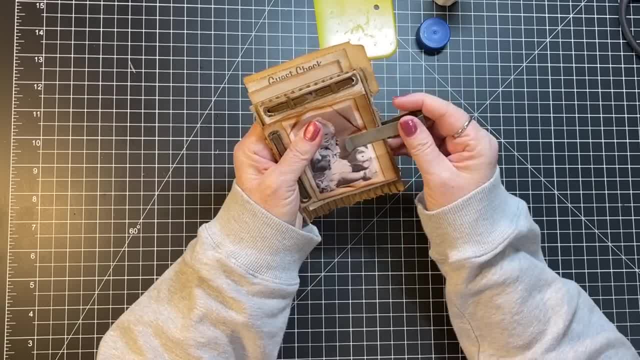 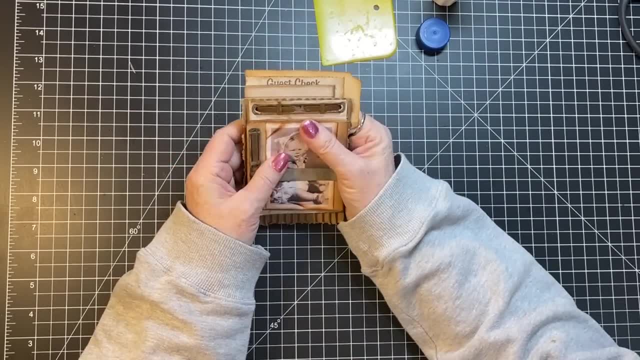 Oh, there it is. Yes, Okay, Okay, I'm going to move. I'm going to move it down a little. I don't want it to be on her cute face. So super cute for a grungy journal. Love it. 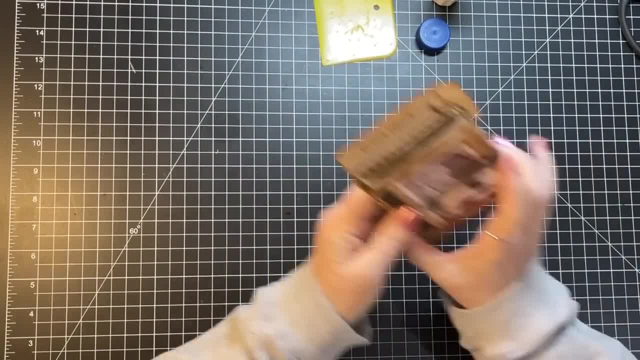 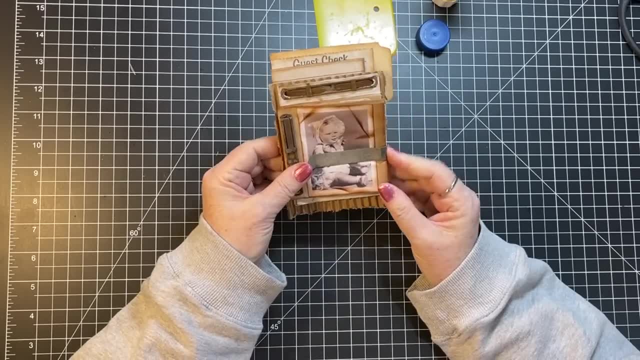 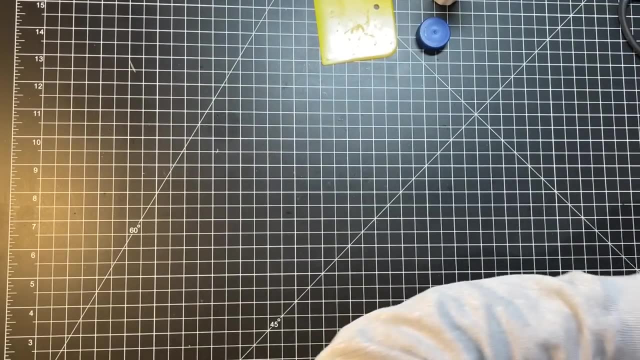 Okay, I think we might have to. once I get my order of these, we might have to make this, Make a, so I might put that with my idea journal. actually, Oh, key, dokey. Then the other thing I was saying I did. 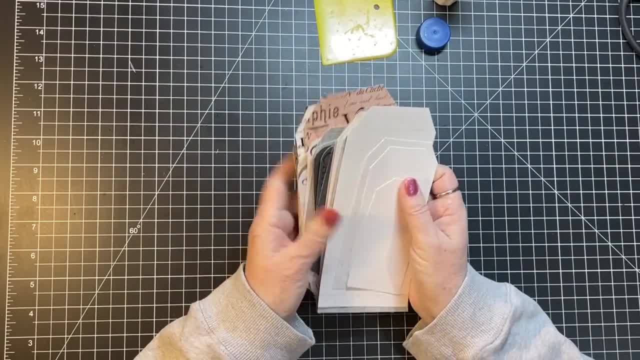 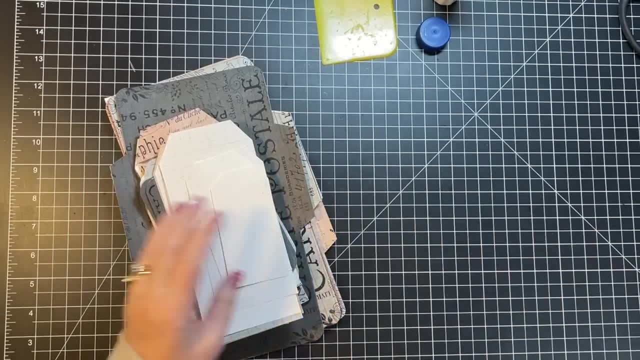 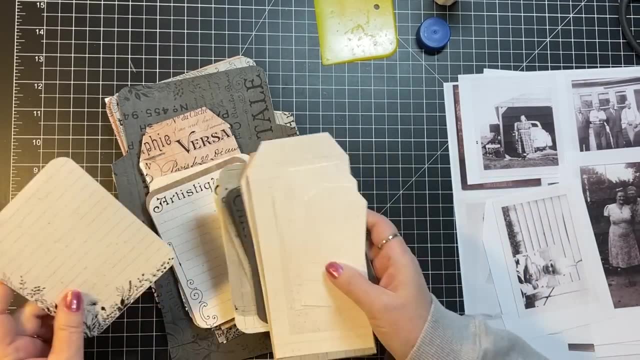 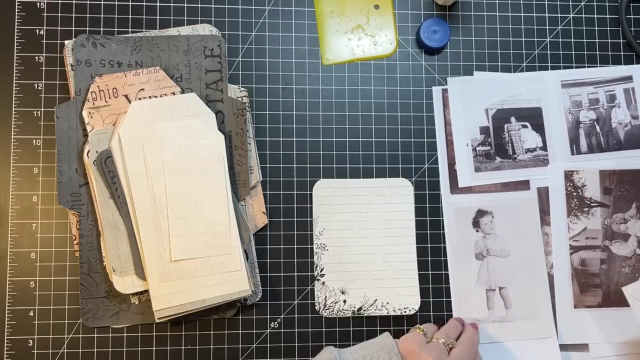 I did some fussy cutting. This is paper baker creations, envelopes and tags and stuff, And I was thinking like some of these, like maybe even that one- Do I have a tall one that would go? I mean, she'd be cute on there. 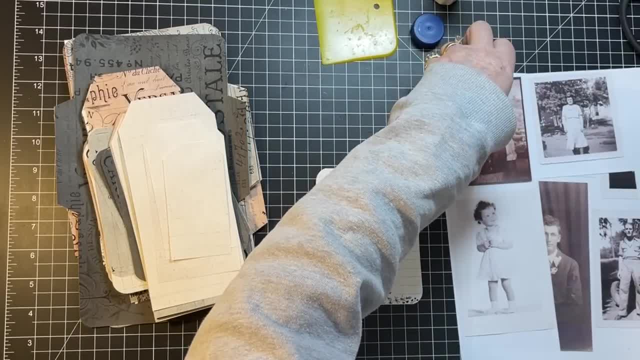 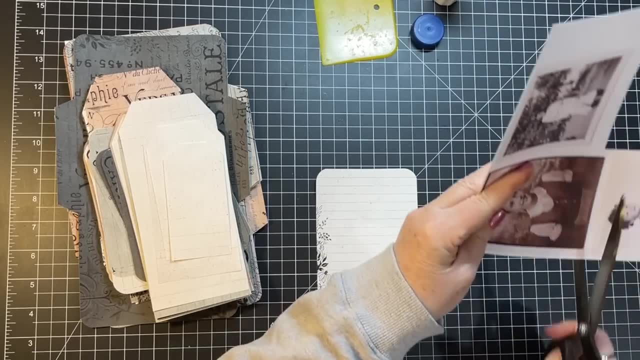 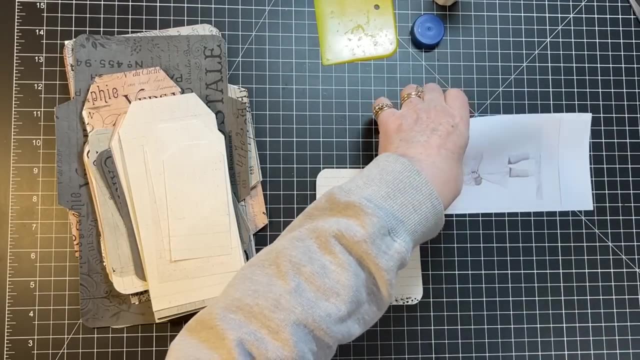 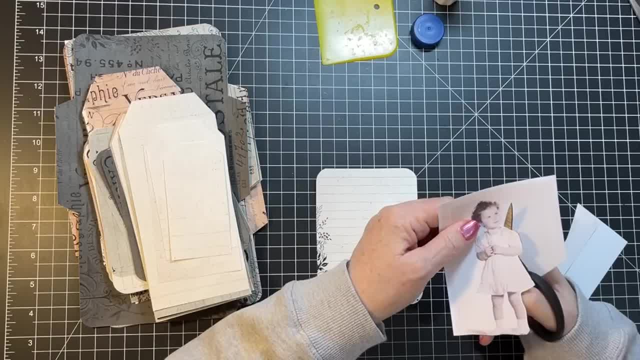 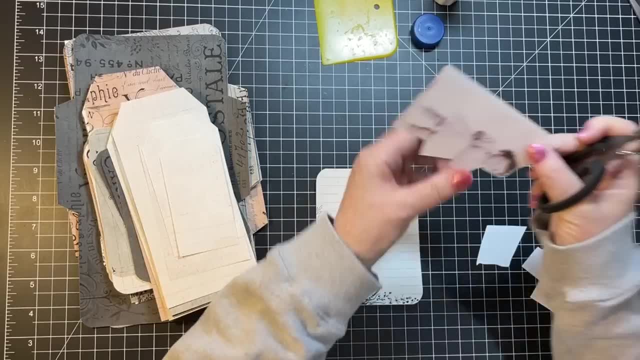 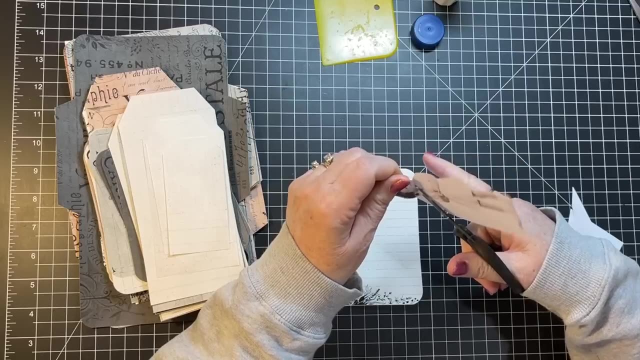 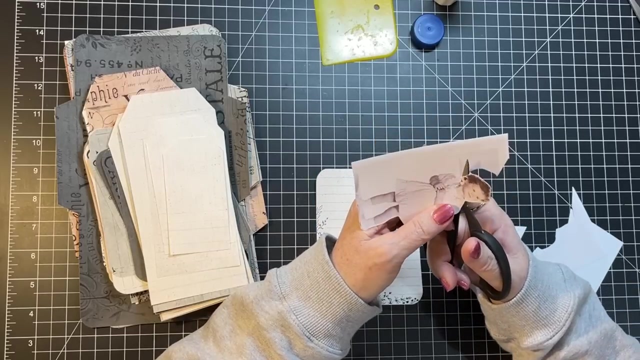 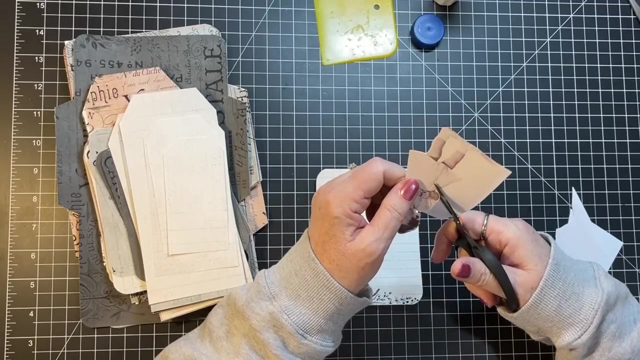 Okay, Okay, Okay, Okay, Okay, I'm going to take the sort a less saturated sort aquele bit board over the random card. Okay, so yeah, one of my brother's grandkids grandsons is um graduating this year, just like mine. 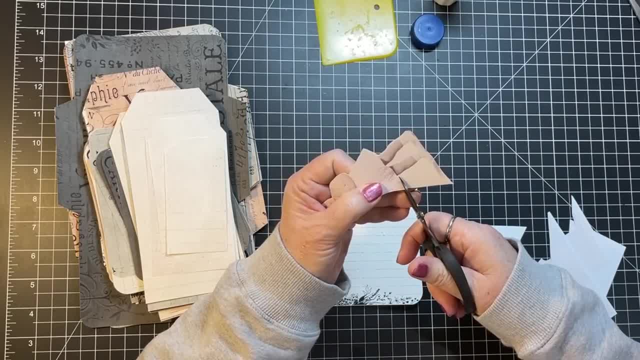 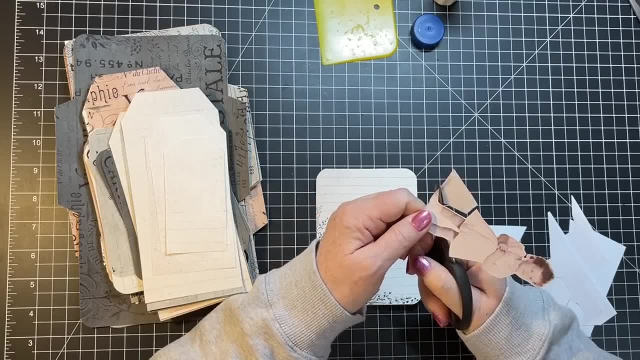 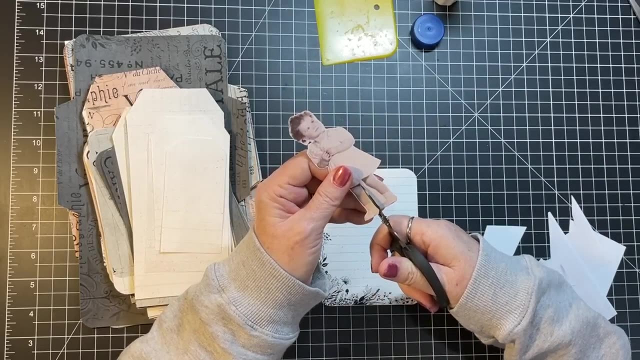 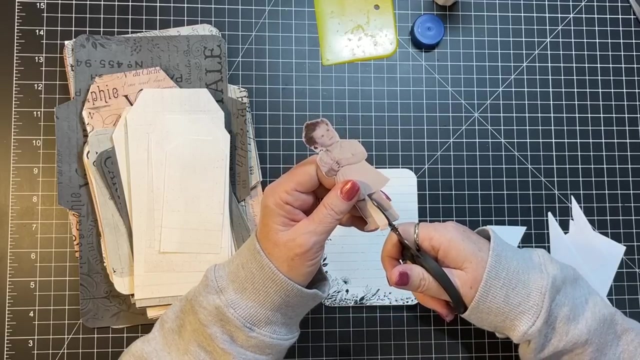 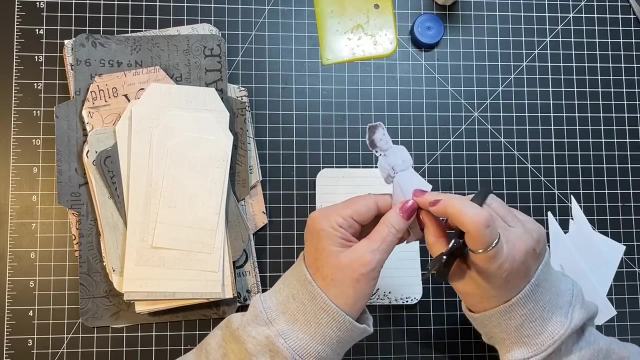 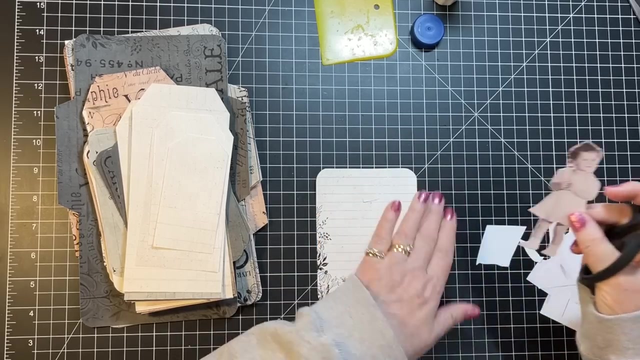 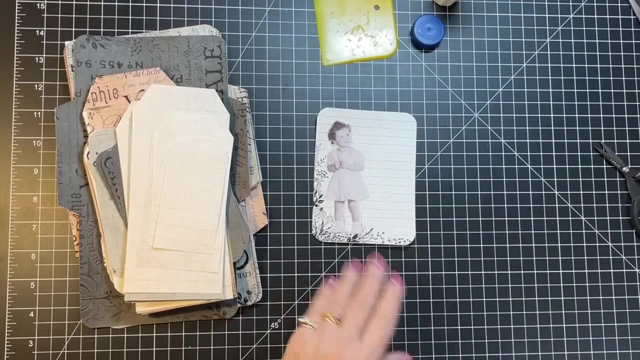 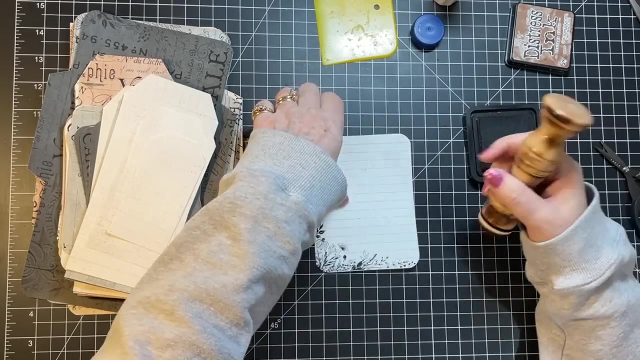 so that's kind of fun. they're the same age. okay, we just about got it here. okay, okay, okay, did a bad job on her little leg there. there we go. oh gosh, she's the perfect size. okay, I'm just kind of making bits and pieces, aren't we? 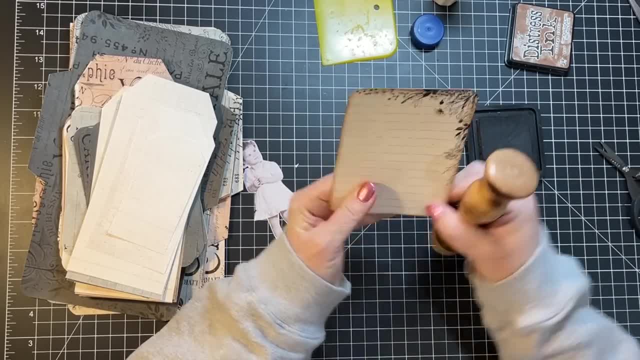 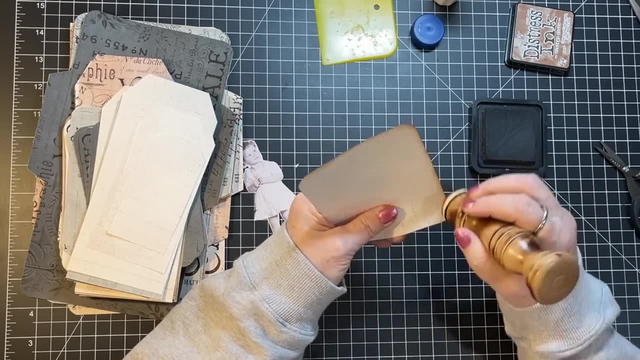 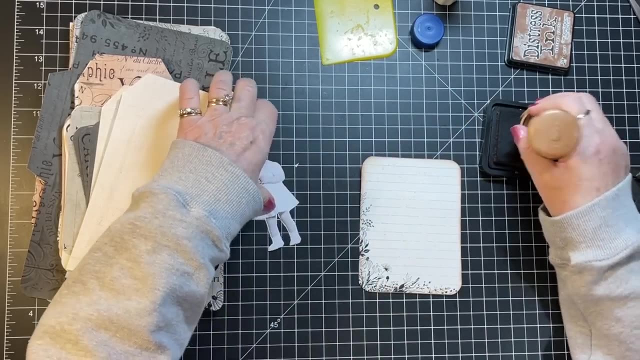 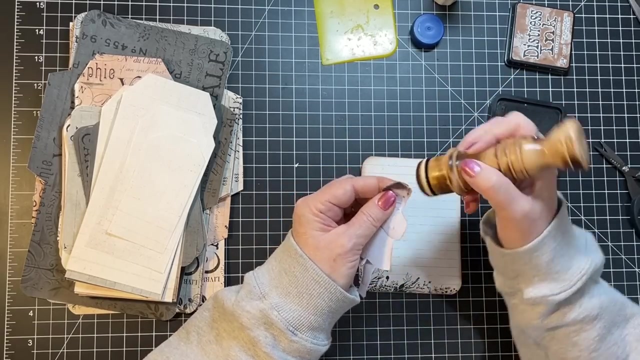 I should grab my to-do box. these were the ones that i had in mind, these little projects. so, oh, i bet you, our thing is ready to cut now too. okay, and on her, i'm just gonna go a little tiny bit on the edge just to make her stand out from the card a little bit. 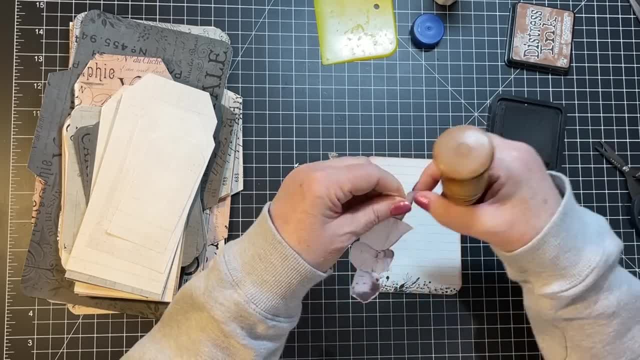 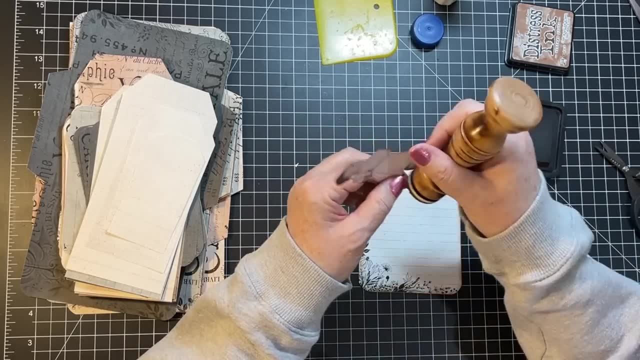 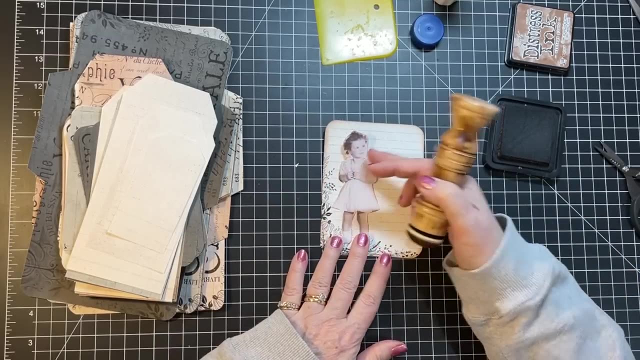 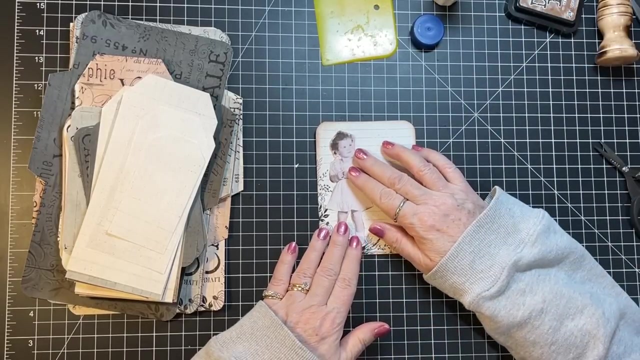 okay, okay, she looks like he has a skin knee, all the better. and she's just standing in those little flowers. i don't know that i want anything behind her either. i think i'm just gonna put her down and then i'm gonna find her and i'm gonna put her on the other side. 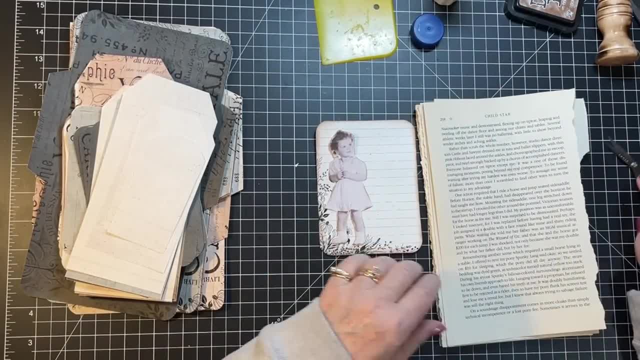 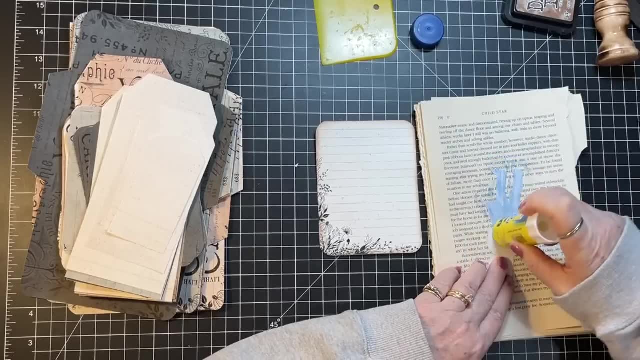 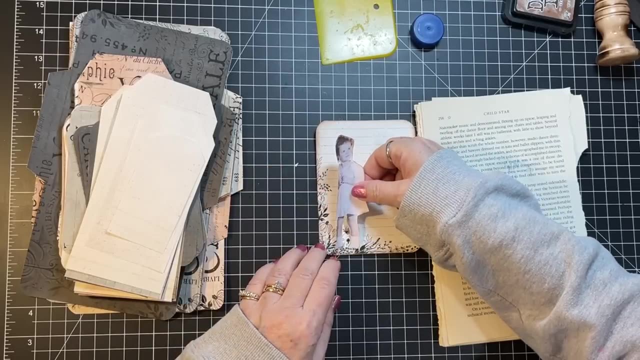 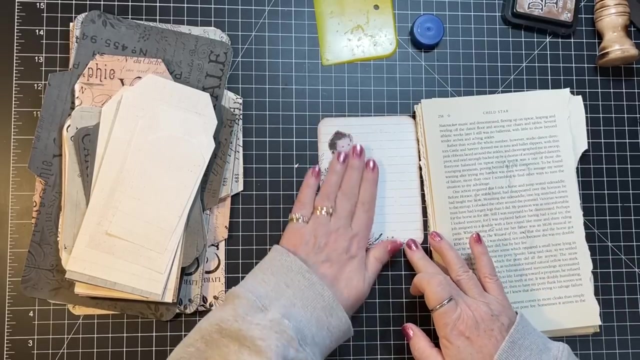 then i'm gonna find her and then i'm gonna put her on the other side of fun word for her, like I had the word pretty or something like that or kind. she looks like a kind little girl. then there's still room to write there, let's. 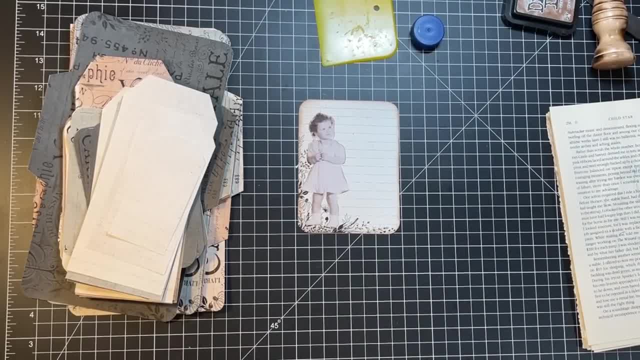 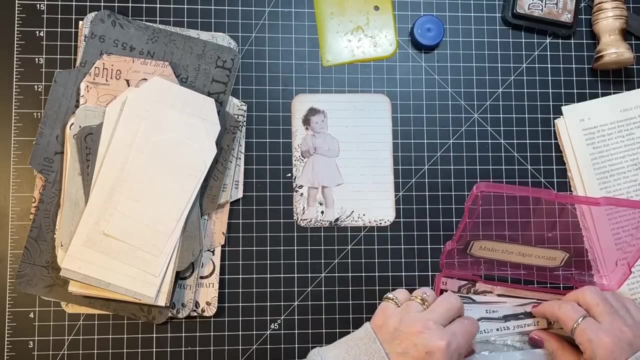 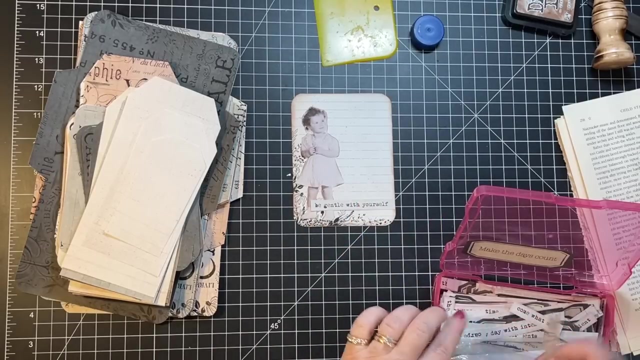 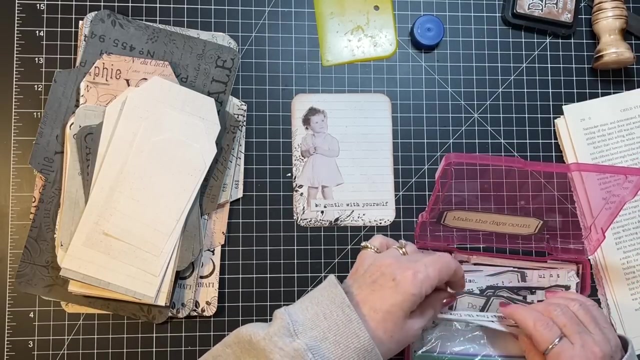 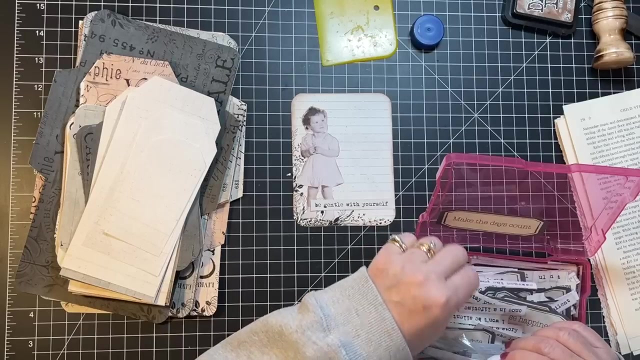 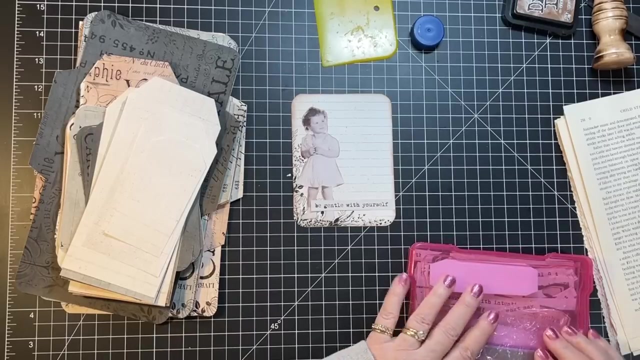 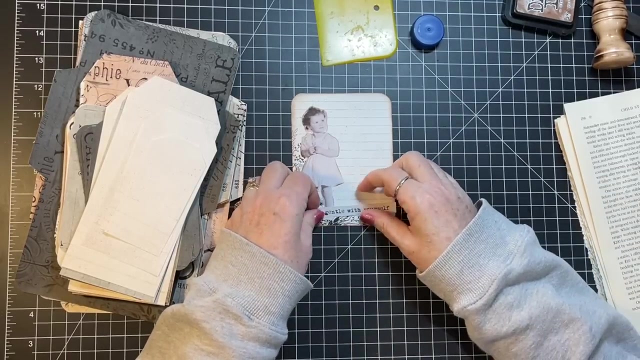 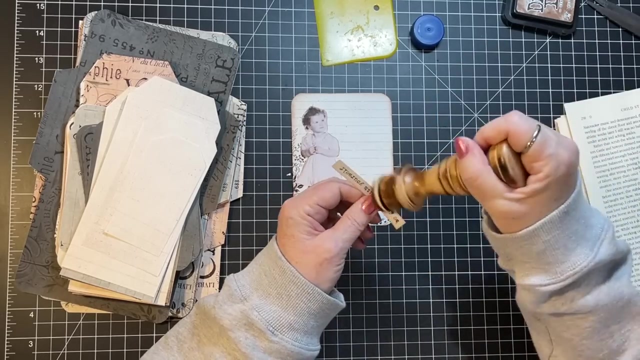 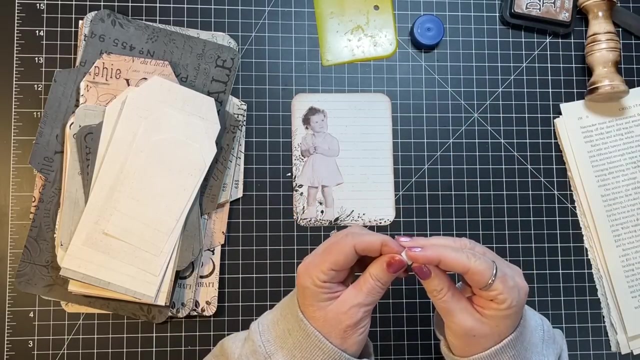 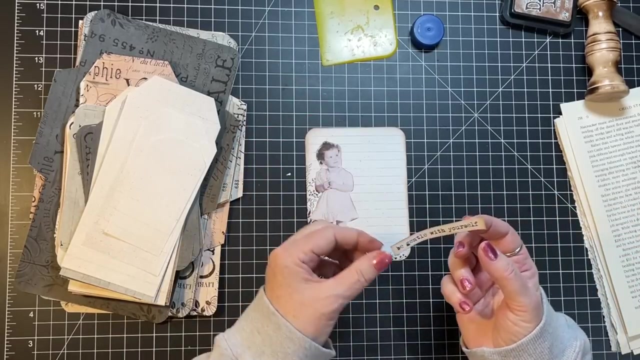 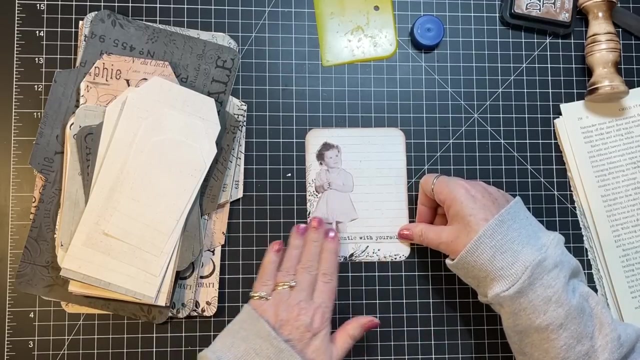 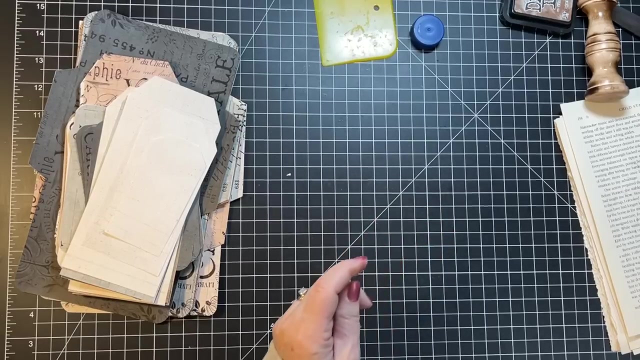 see words: good for her. I'll be gentle with yourself. that's cute. this is from pink monarch prince. yeah, I think be gentle with yourself is sweet. do the edges a skosh? okay, I think we'll just go right here. fun, that's a sweet little card. okay, let's check this out. 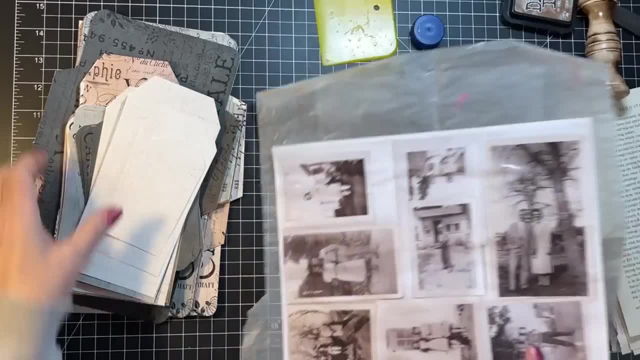 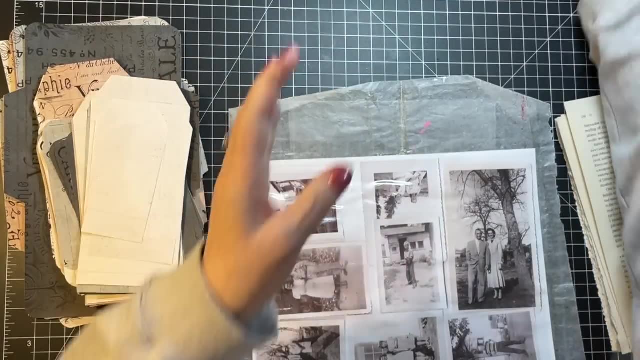 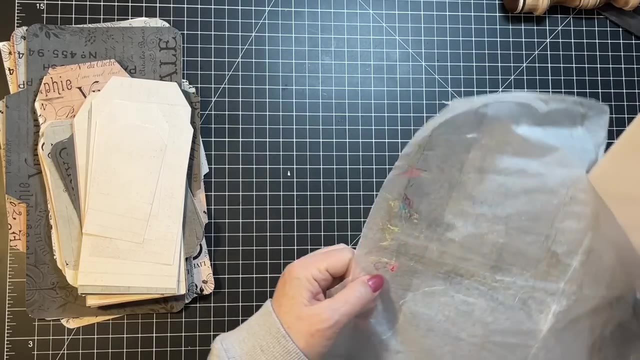 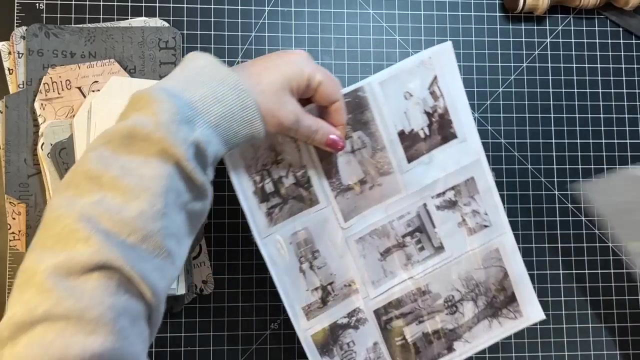 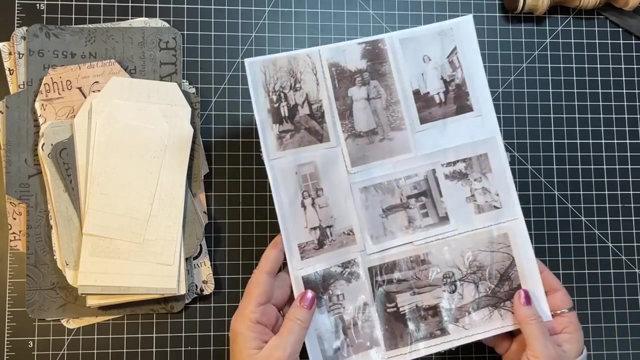 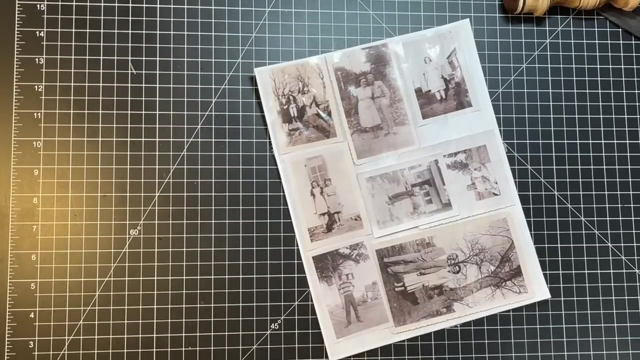 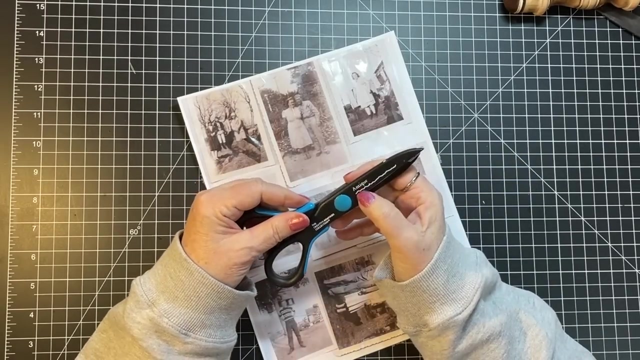 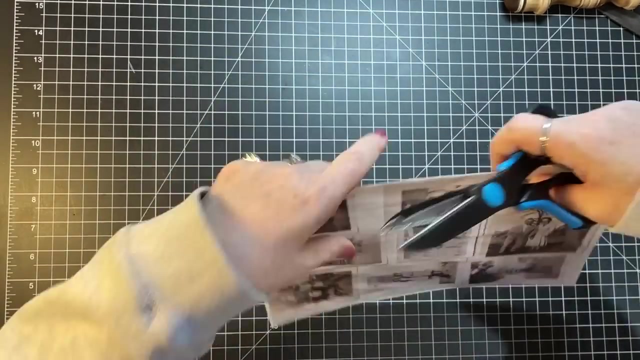 okay, okay, move, let me move a few things. things up a bit, give myself some more room. it's mostly dry and it is shiny- I don't know if you can tell very well, but it is- and so then these are creative memories, scissors, and they're called antique and they're just jiggy-jaggy, and so I was thinking to cut. 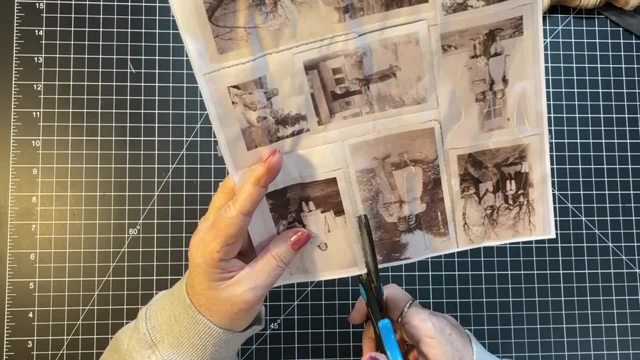 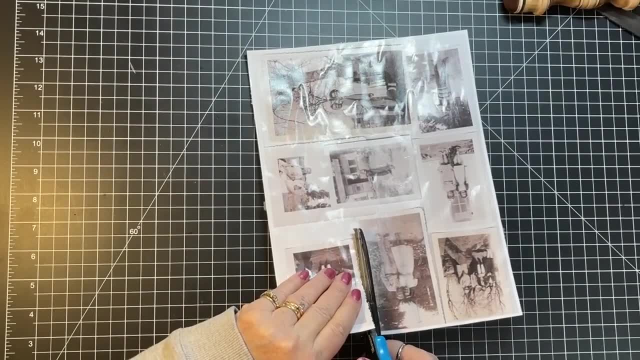 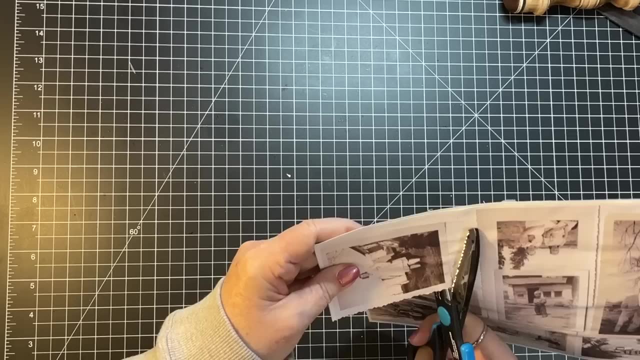 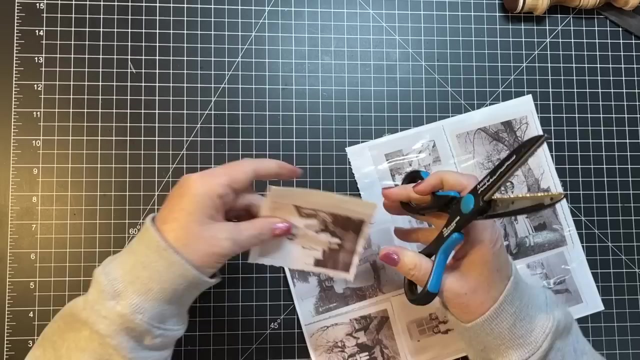 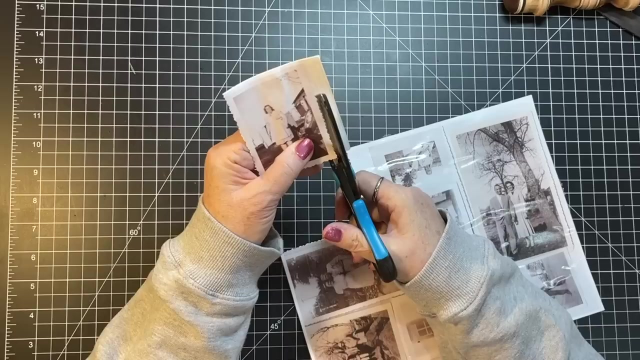 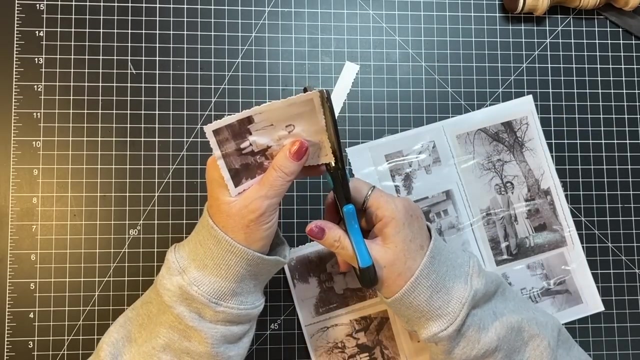 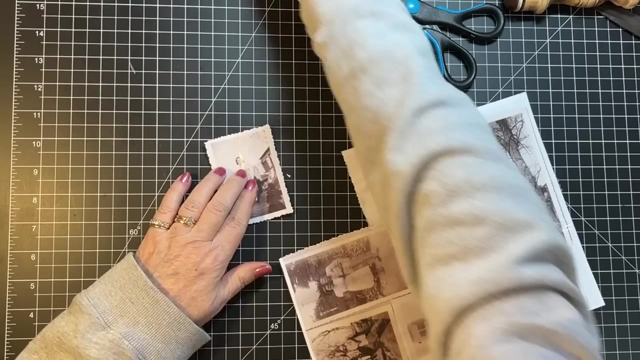 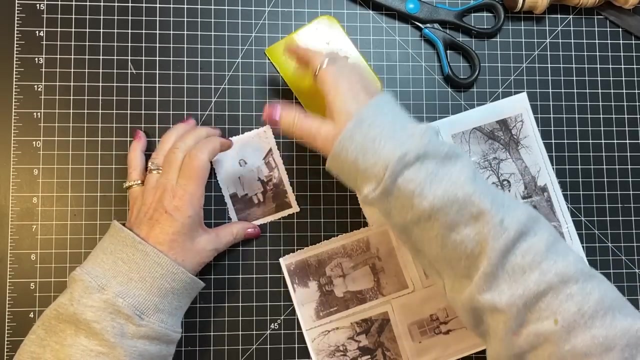 these out just like, and have them look like an old photo. It might not be dry enough, Okay, Okay. so I don't know if I can smoosh that down a little bit. Oh, my gosh, though it worked, you guys. 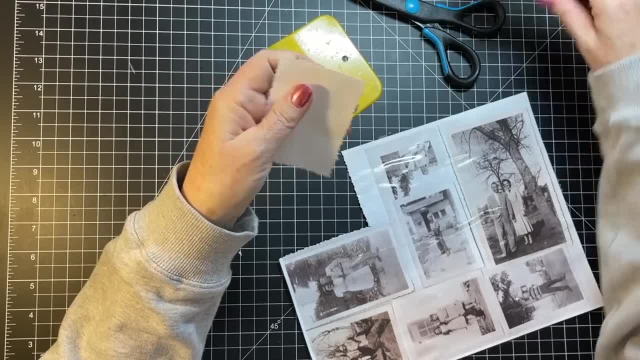 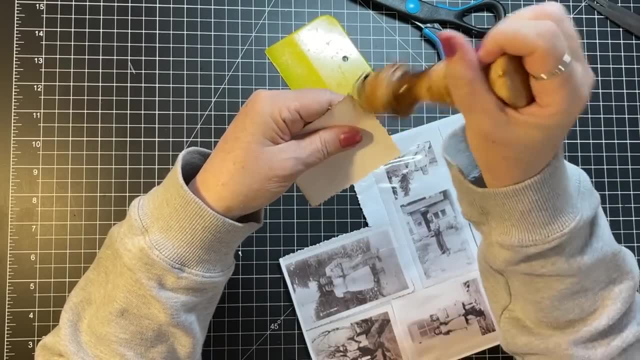 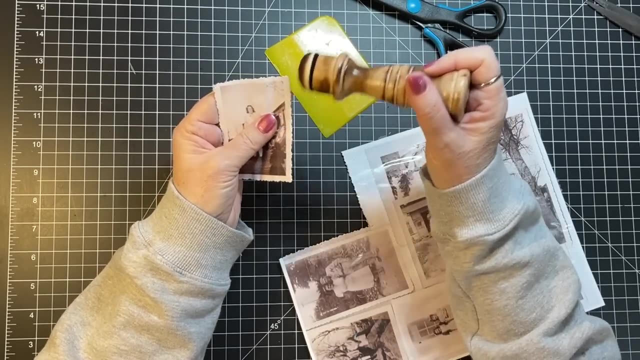 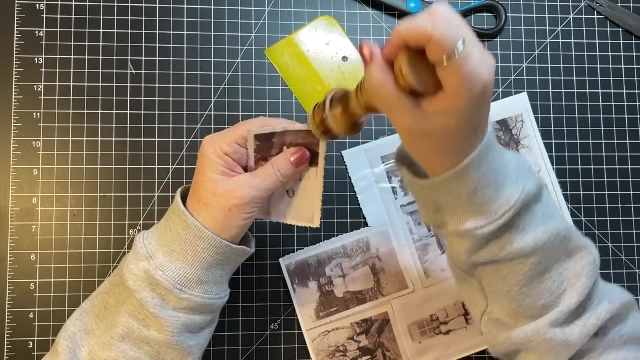 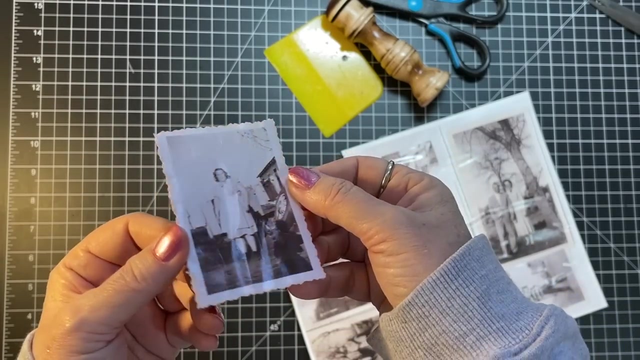 It looks like. I mean, it's a little journal card, but it looks like an old photograph because it's got this shiny. So I'm going to do just the very edges. So you see that It's got some lumpy bumpies. 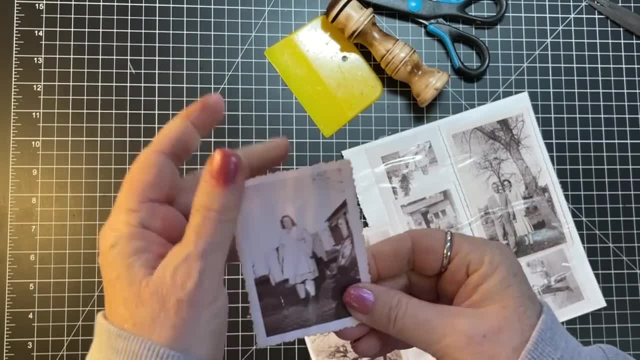 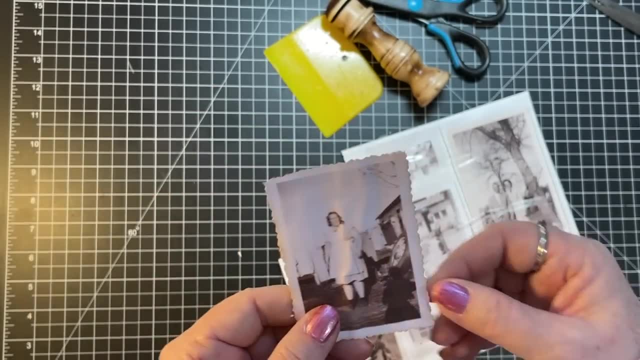 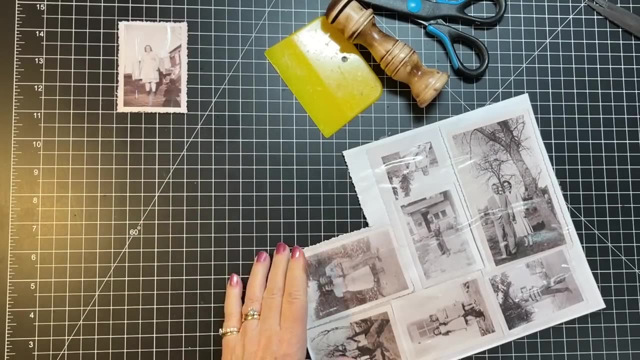 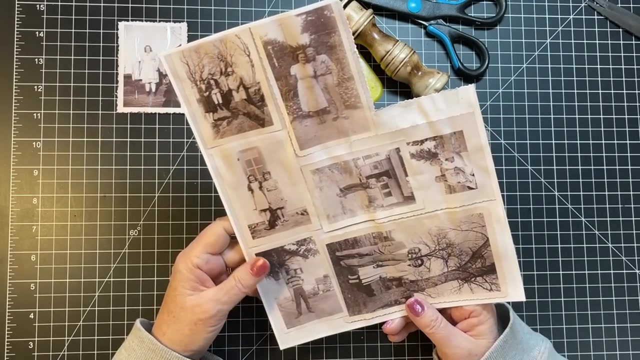 but I'm just going to go ahead and say that gives it character like it's been, you know, in a box in somebody's closet For many, many years. That's fun though. Okay, I'm thinking I'll just go down this side maybe. 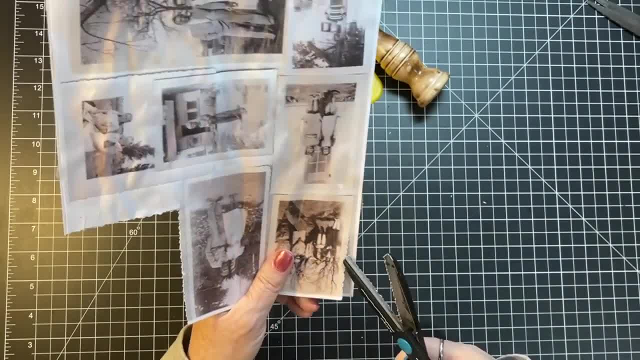 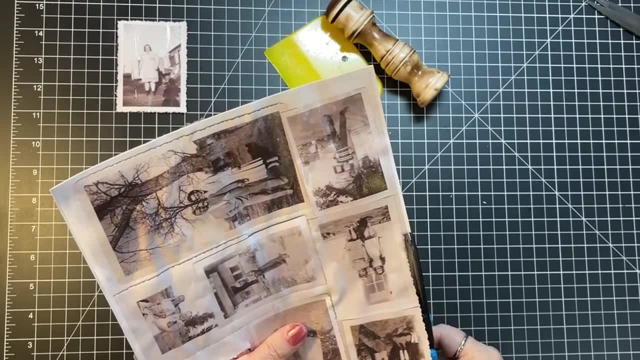 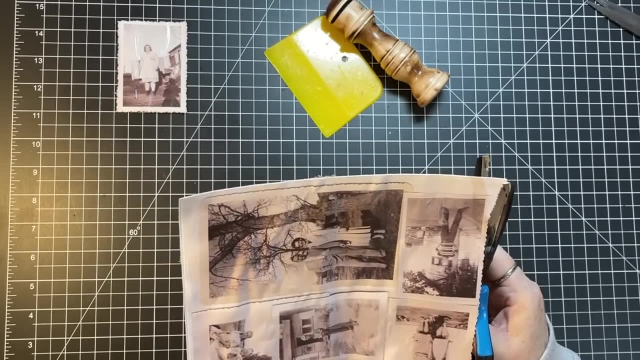 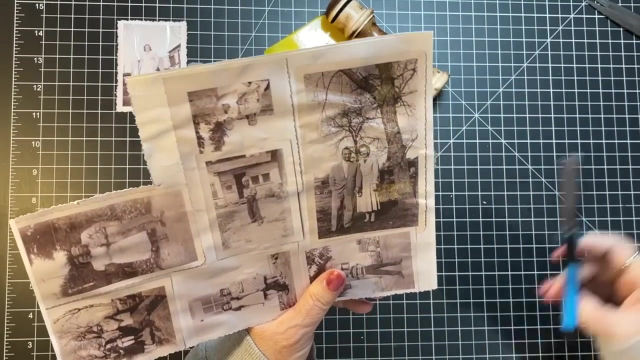 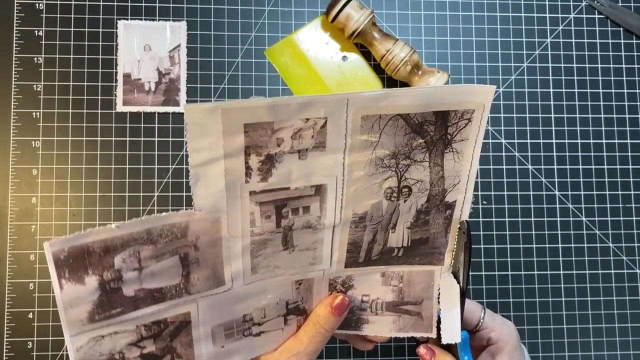 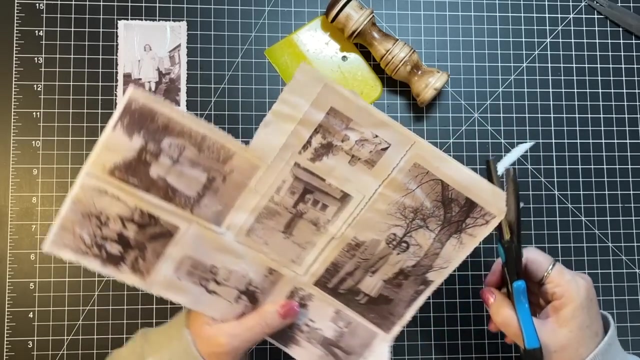 Maybe I rarely use- I don't use the glossy Mod Podge, so this is a good way for me to use it. Okay, I'll go here And This side of this. Okay, Okay, Okay, Okay Okay. 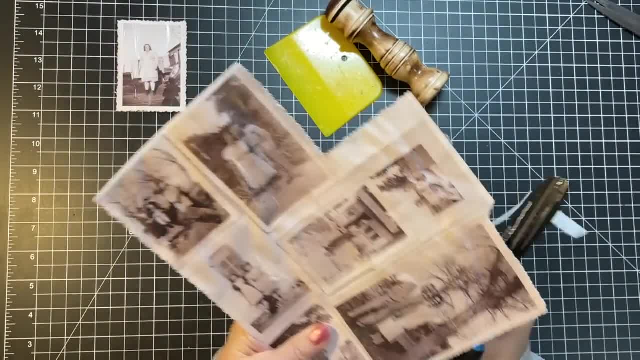 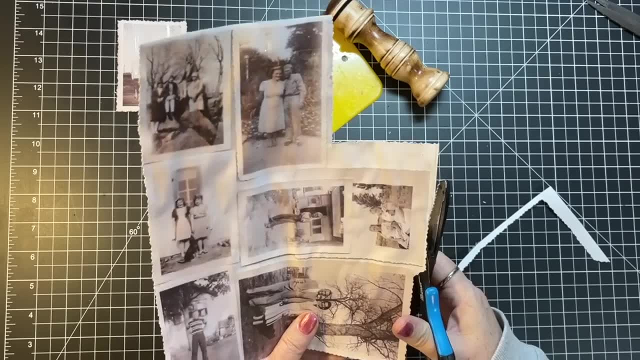 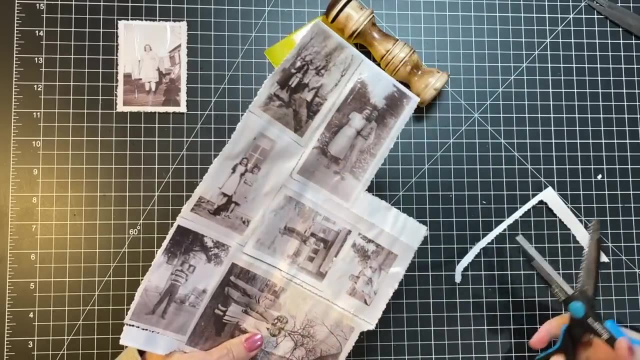 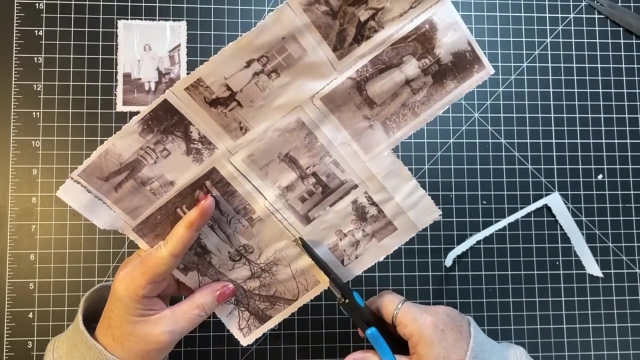 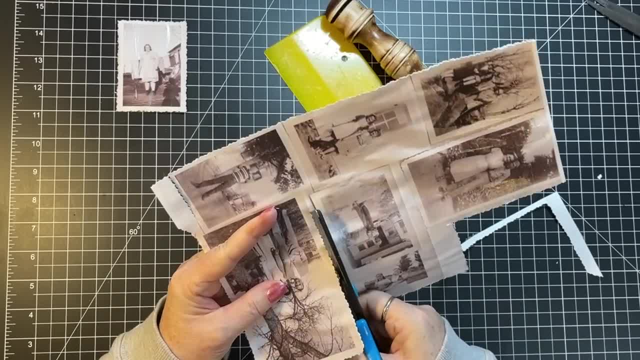 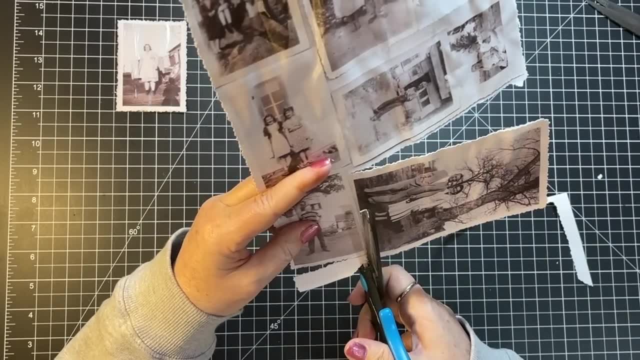 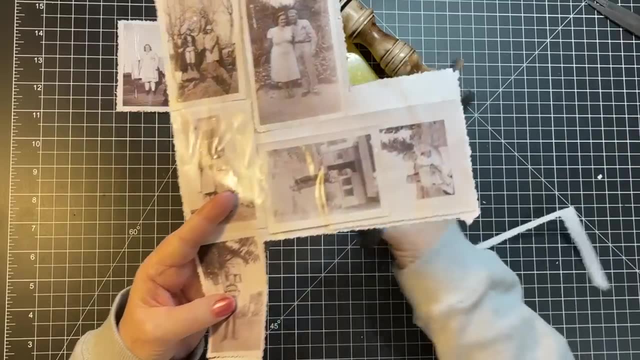 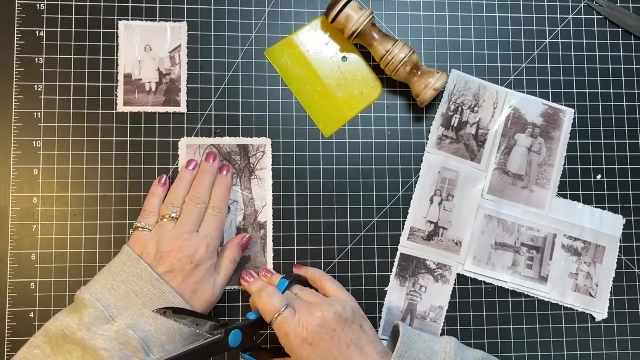 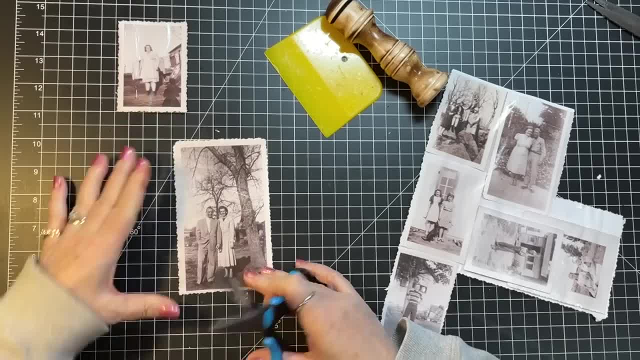 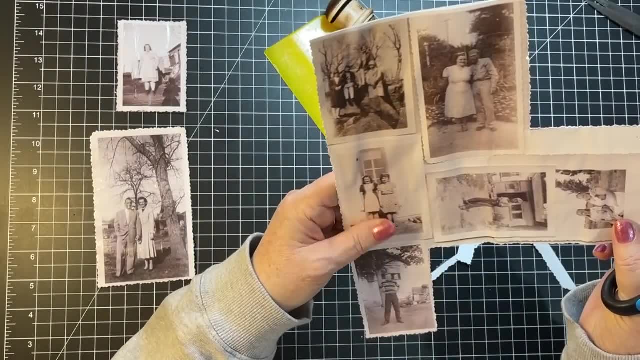 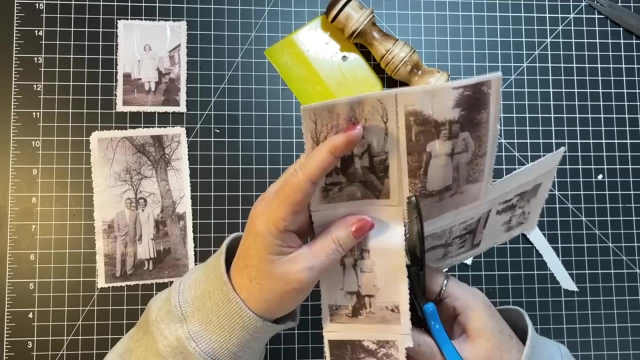 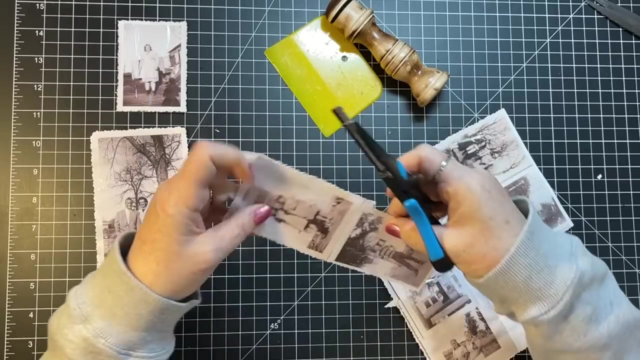 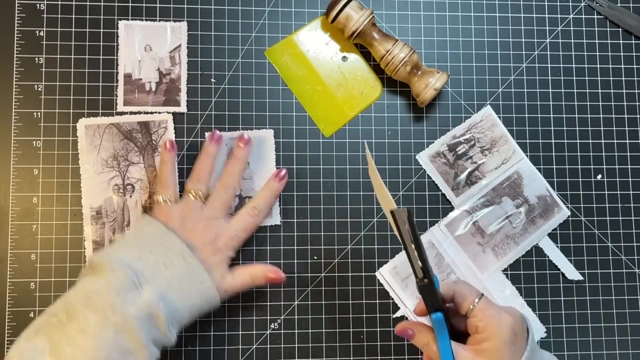 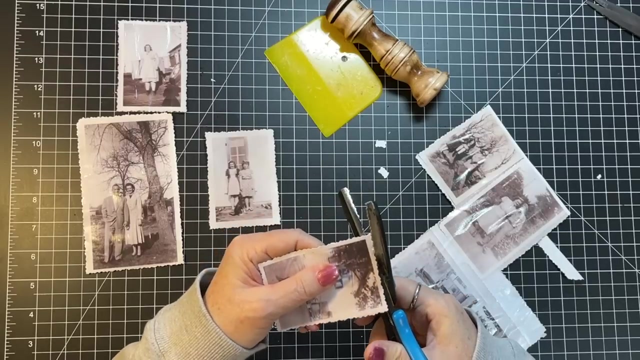 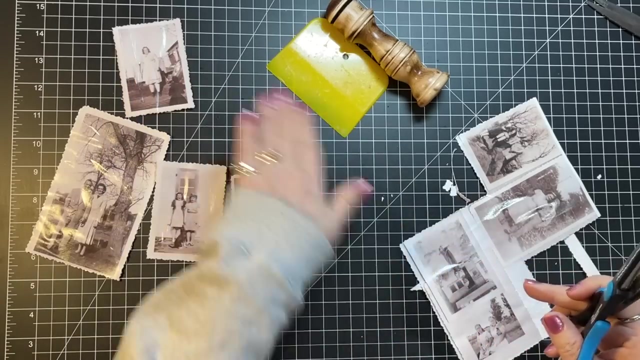 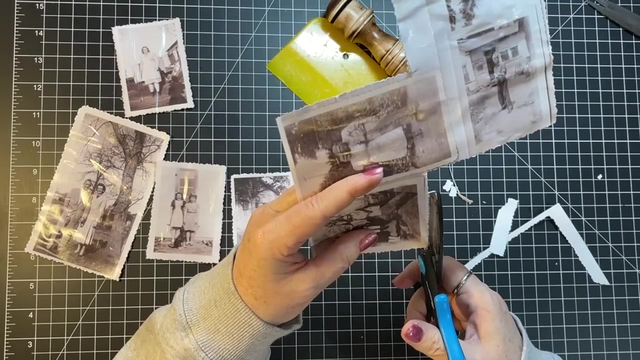 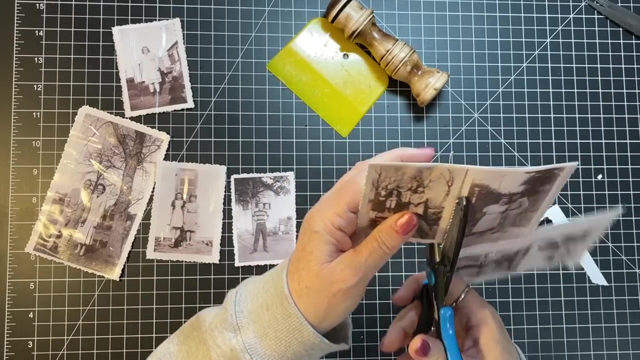 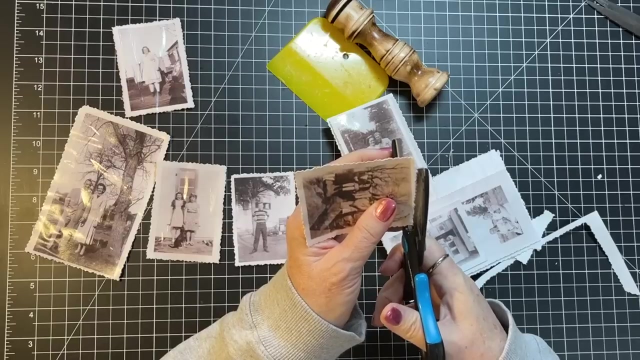 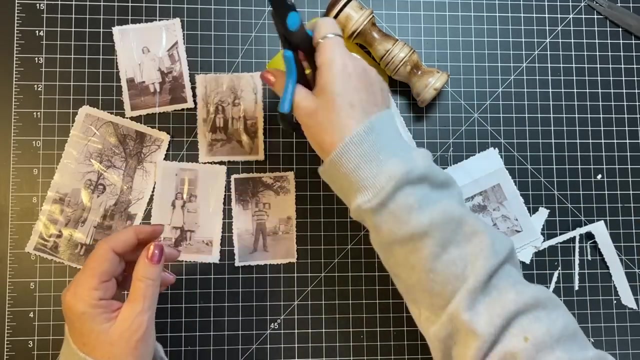 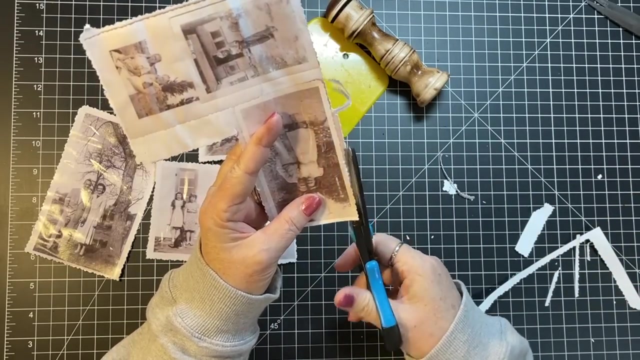 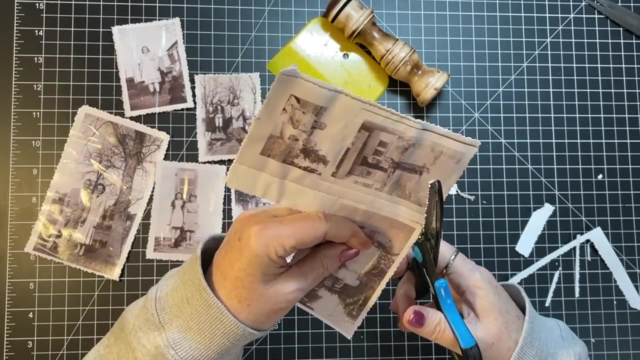 Okay, Okay, cool. i love it when you have an idea and it actually works. you know, these scissors hurt my hands too, but i use them so rarely that it's okay. okay, let's see where am i at. i have a lot of the pictures of me as a little kid. 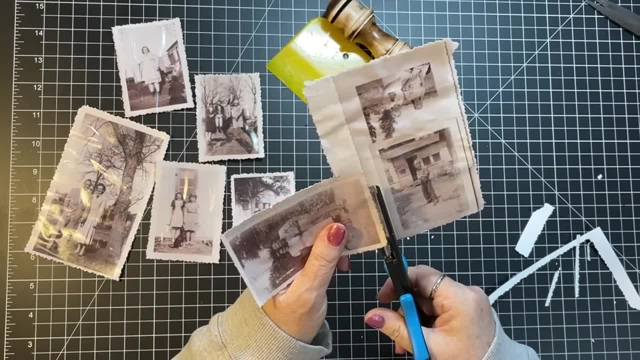 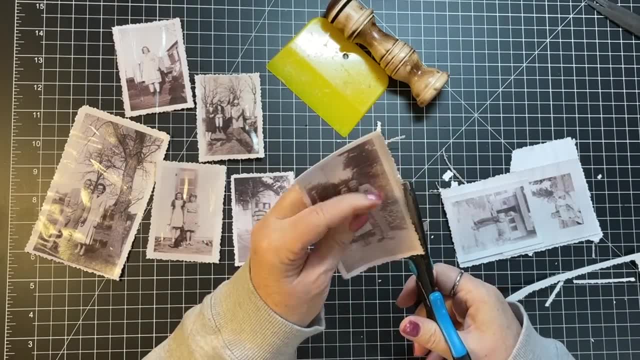 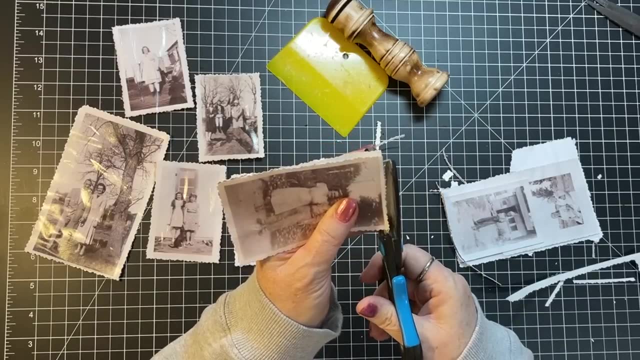 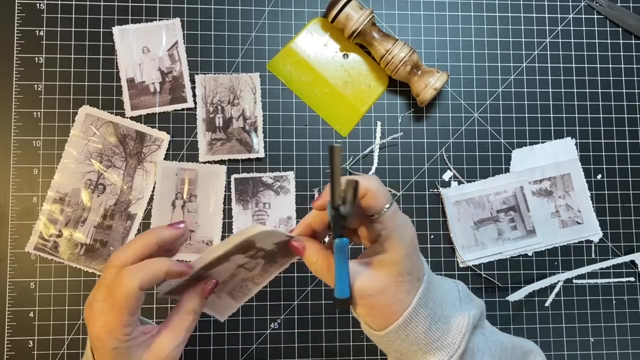 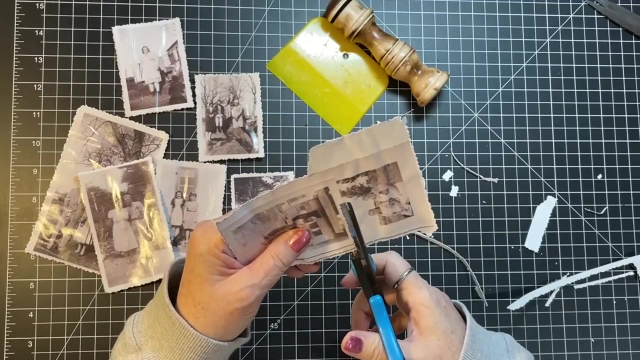 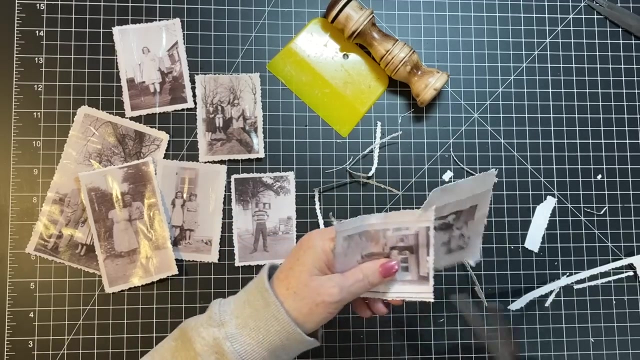 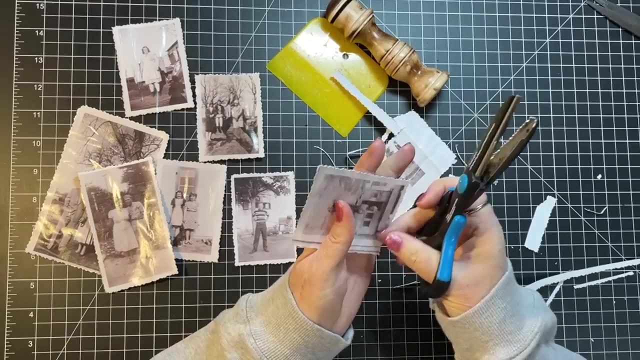 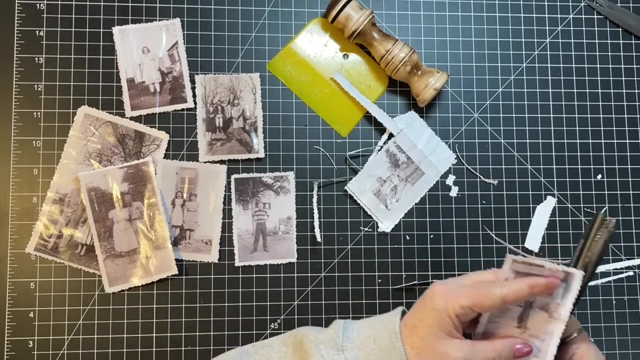 are this kind of photo that, um, um, you know, has the jaggedy edge. okay, just kind of nip the edge of this, i can. oh, needs a little extra glue. okay, we can do that. let's see okay here. So I feel like I need to find a better way to initially glue down the pictures You 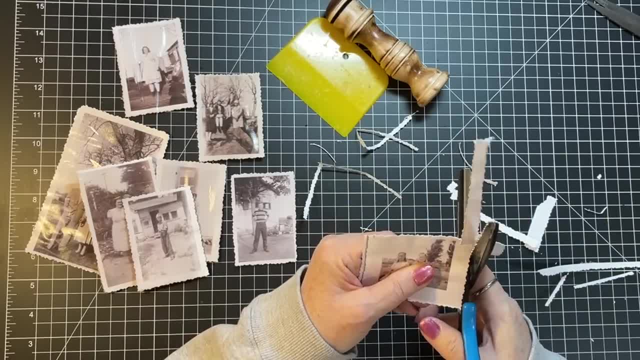 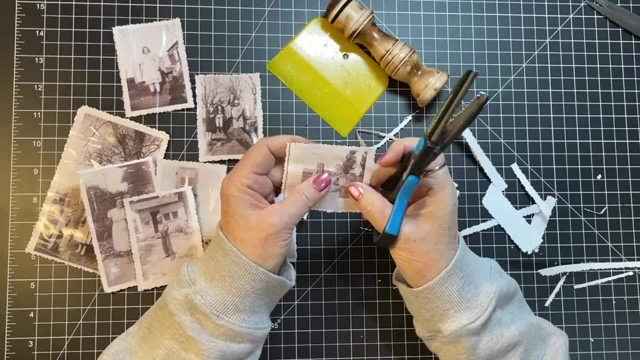 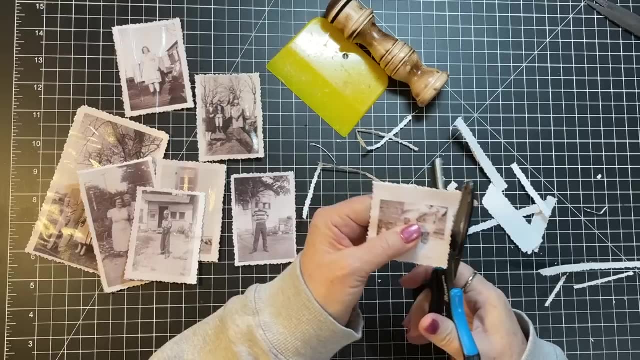 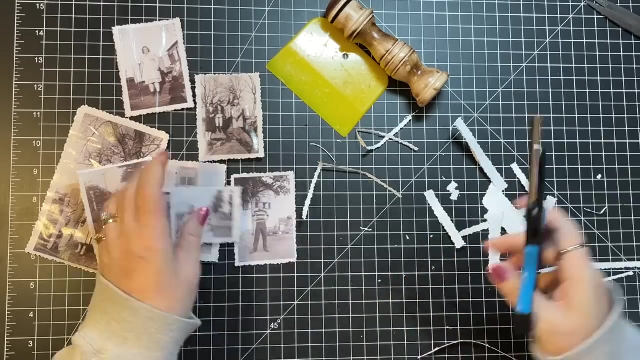 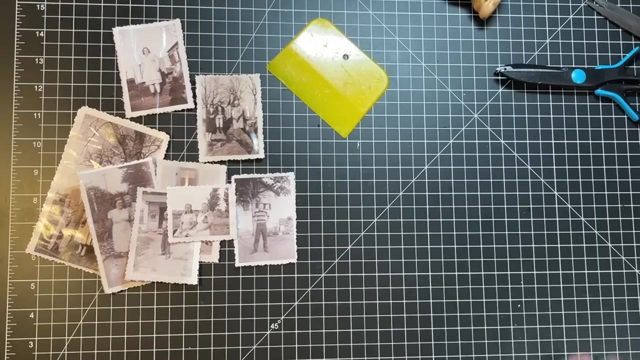 know, maybe I- let's see, maybe what I do is just cut them and do them individually instead of the whole sheet. I don't know, I'd have to work on that. But all in all I'm really happy because I think they it turned out like I had in my head, which you know, isn't always the case. 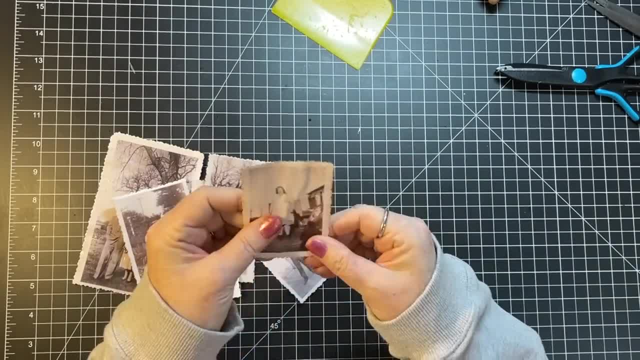 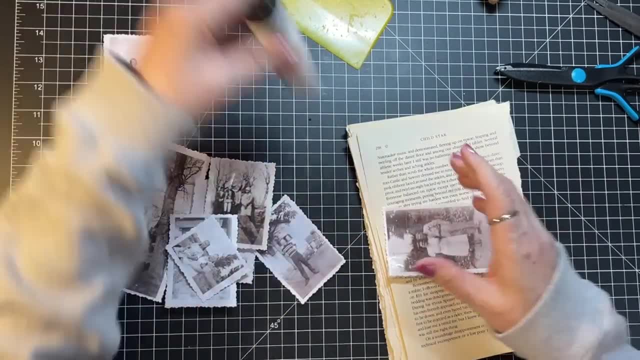 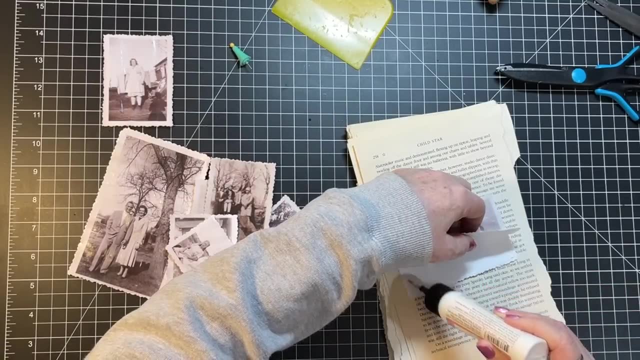 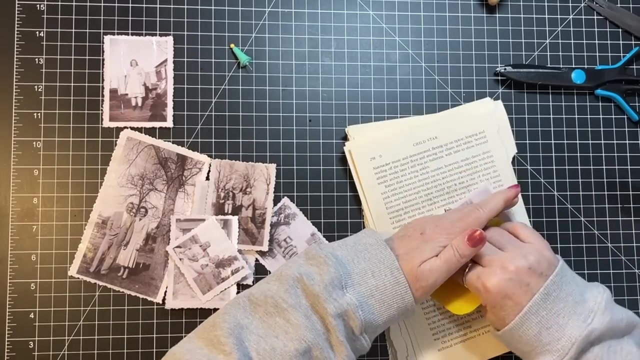 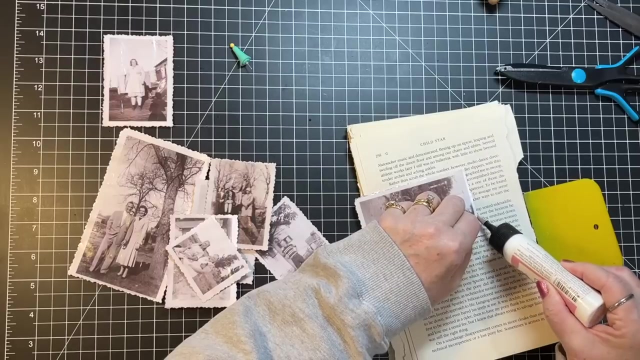 So they need a little extra, does this one? this one's okay, But some of them need a little extra glue, like this one, So I'm going to just use art glitter glue and go on the edges. Okay, Oops, A little on that corner. This one must have been on the edge that I 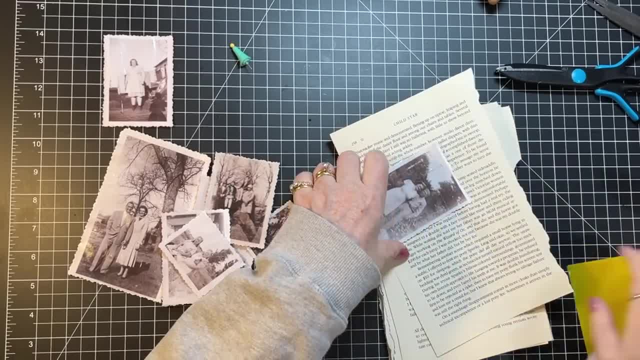 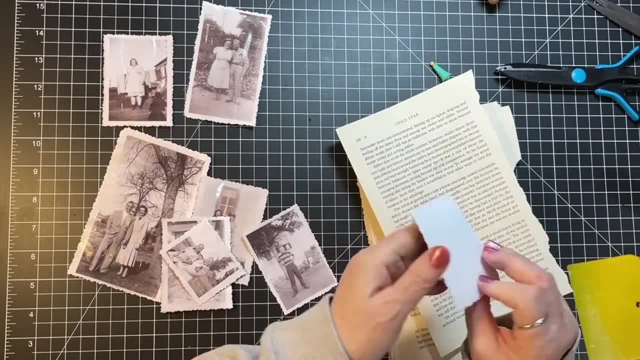 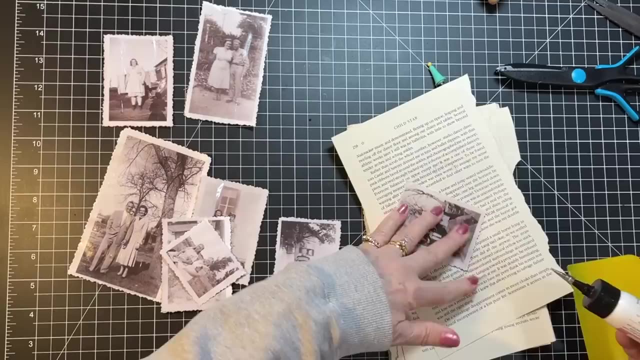 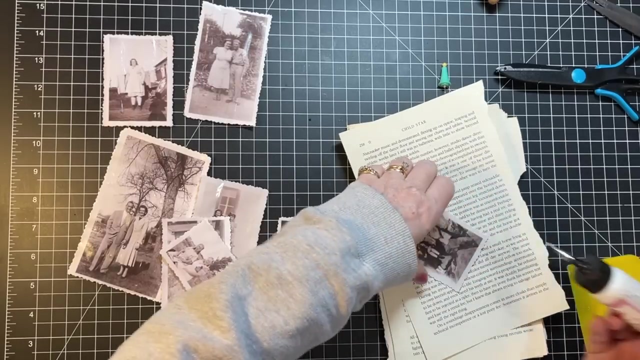 mod podged first and it dried out a little bit. Gosh, I'm excited about that. That actually worked. It's awesome. Okay, Got to do a little tweaking here with the glue, but other than that it worked, Okay, Yeah, I think I can't mod podge them. I have to have to do them one at a time, I think. 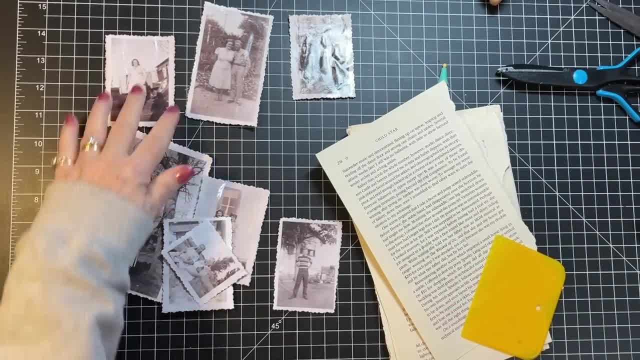 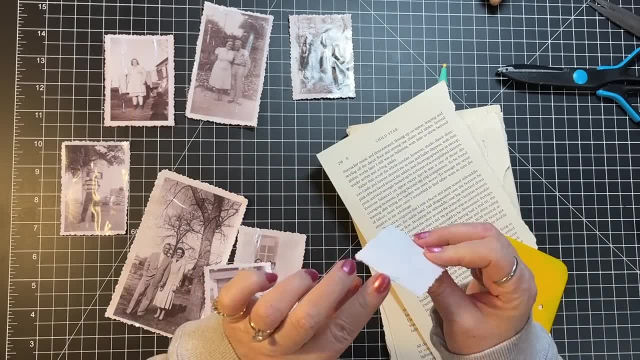 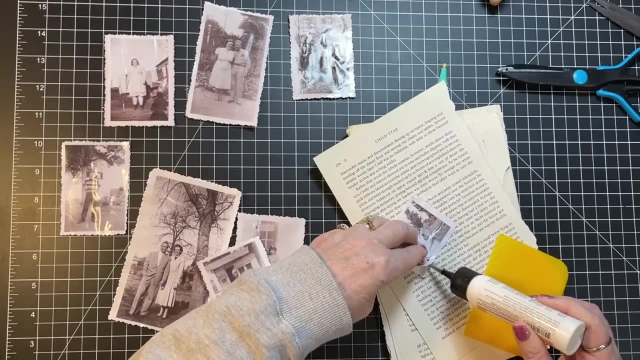 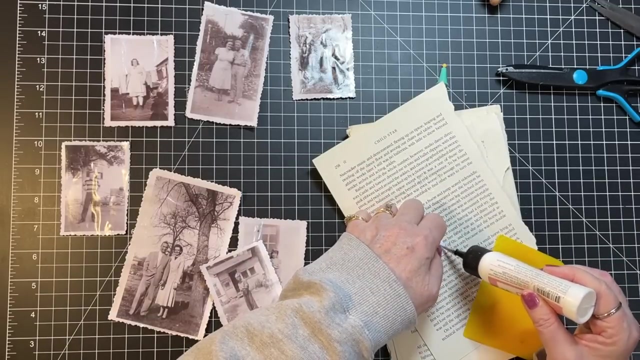 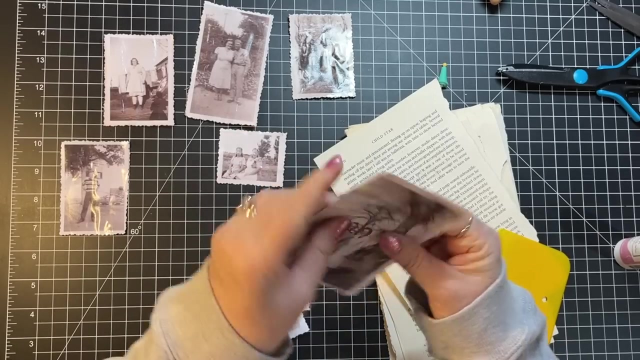 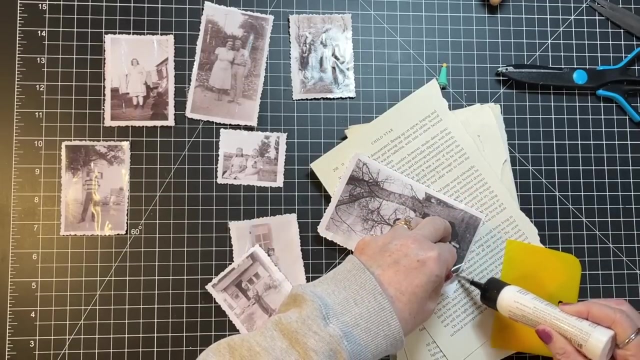 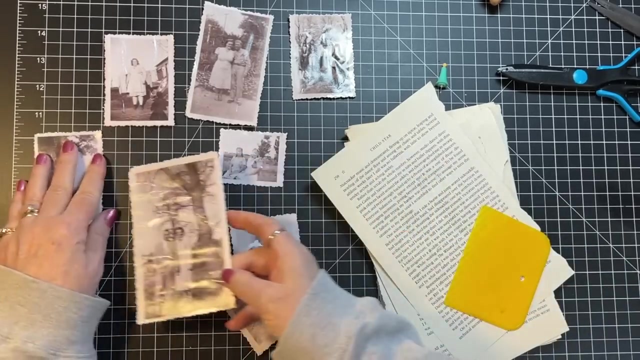 Okay, There's that one, This little dude. he's well stuck down. It's got a corner, This corner. Okay, How about this one? It's pretty good, all except for this corner, Did I feel? did I feel like that one was pretty good? 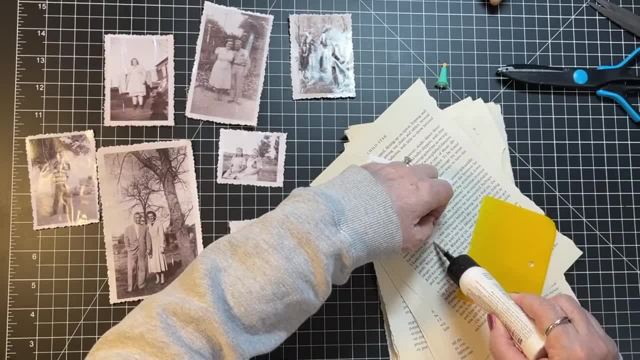 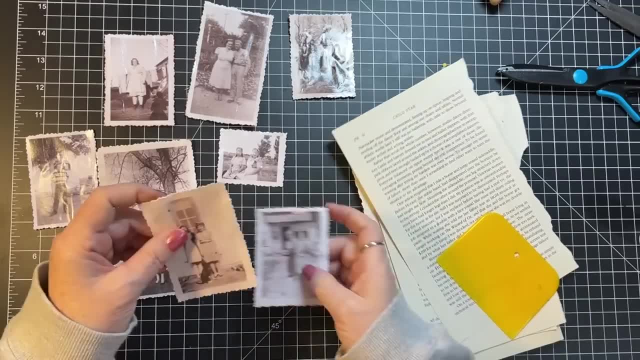 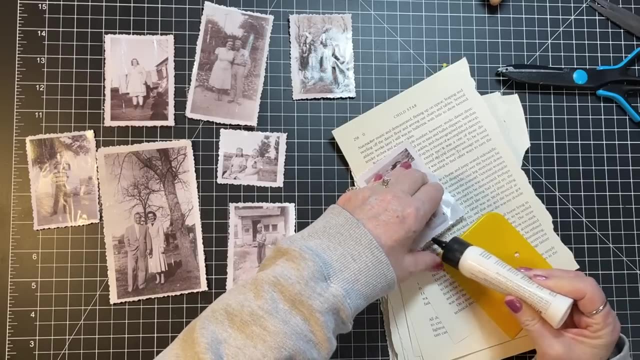 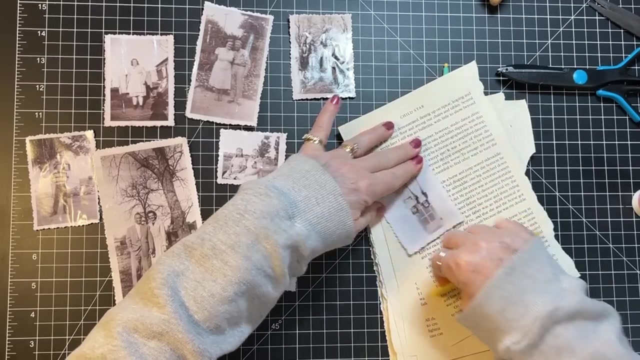 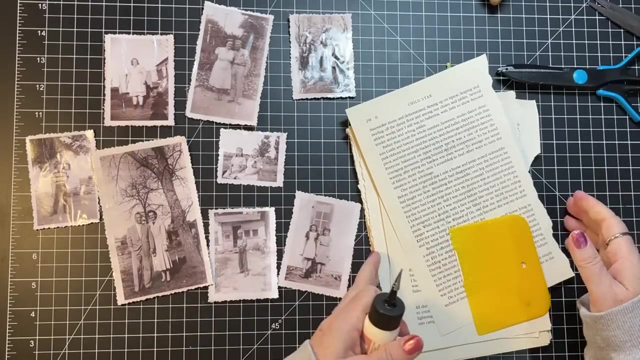 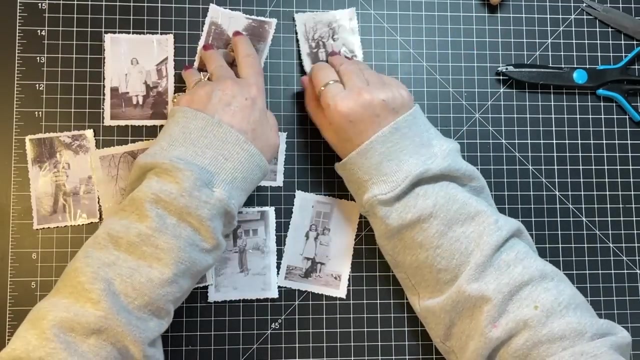 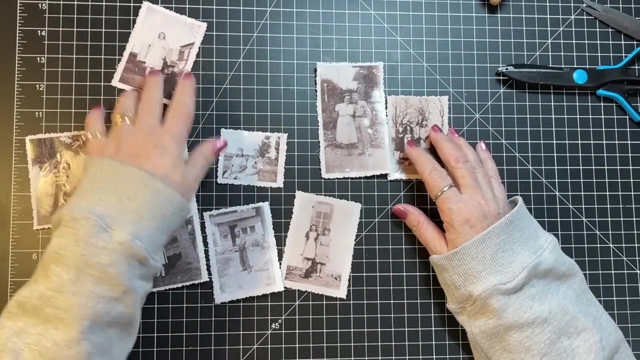 Oh, maybe the corner. Well, those are pretty fabulous. I'm excited. Oh, there we go. They're all all nice and glued down, and then it's just going to be like this one I'm going to do a little distressing, is all. 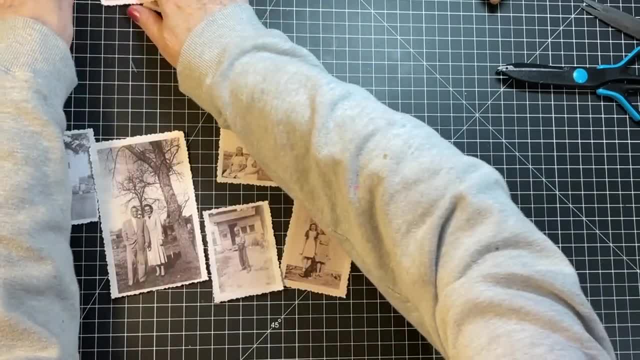 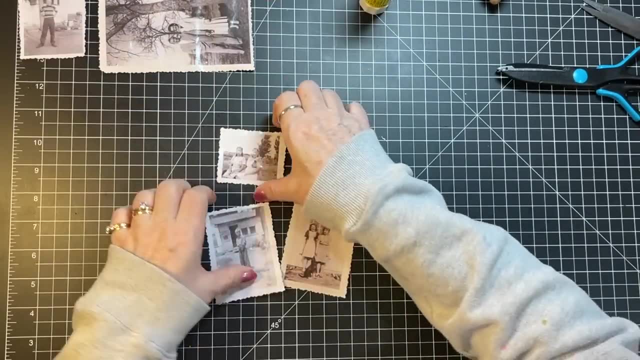 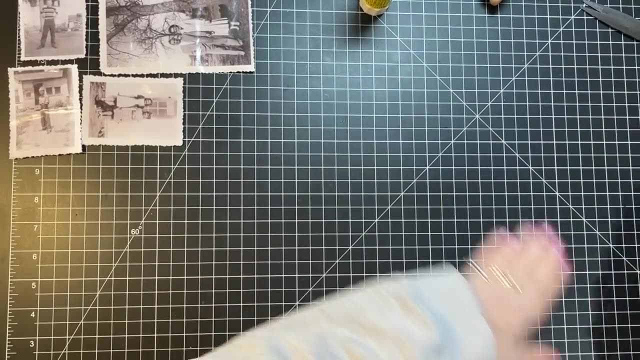 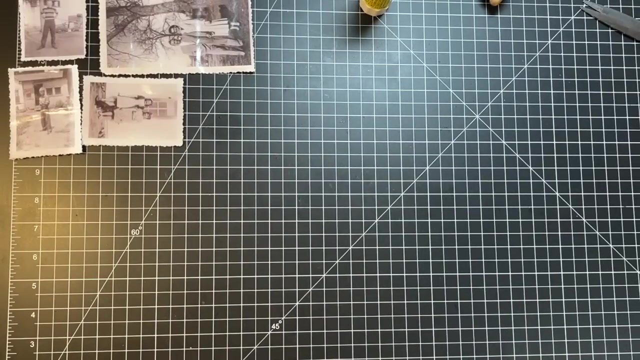 How are we doing? time-wise, Not too bad, Okay, So I'm going to just set these up at the top of my table to dry out a bit more, And I will distress those later. Okay, Okay, Let's look at this giant packed, ever so packed. 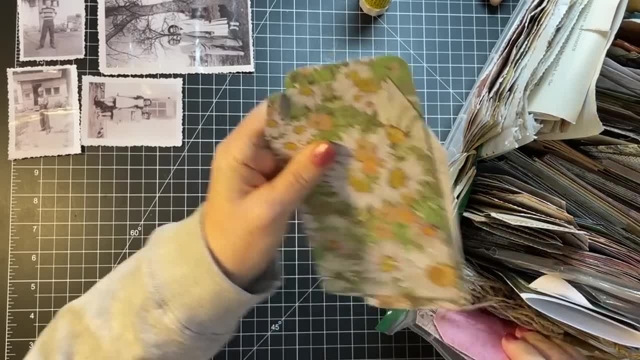 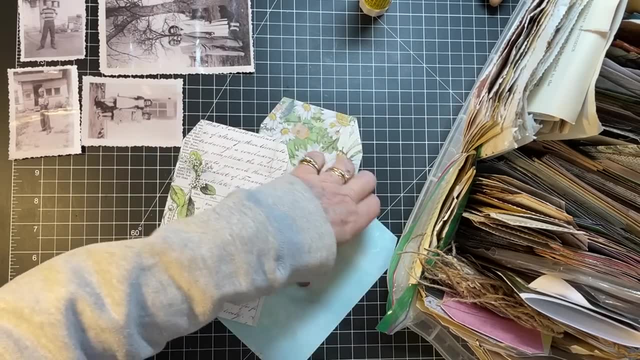 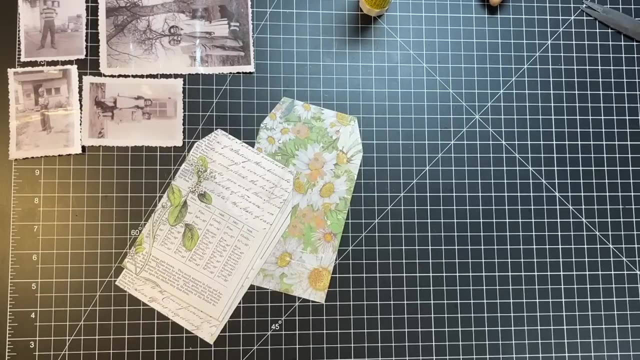 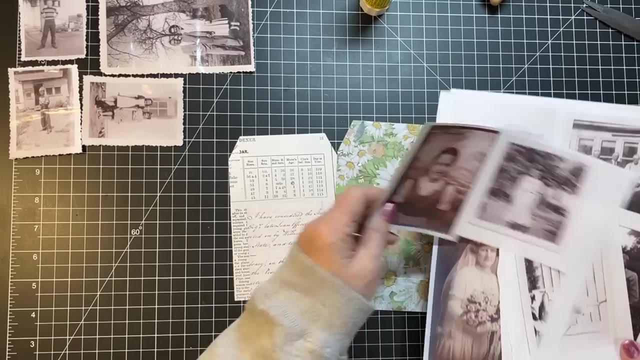 Ooh, that could be fun. What are these? These? I think I did these last time. I did a Scrappy Saturday where I used up scrapbook paper. Let's see if we can use pictures on those. We have left this little guy. 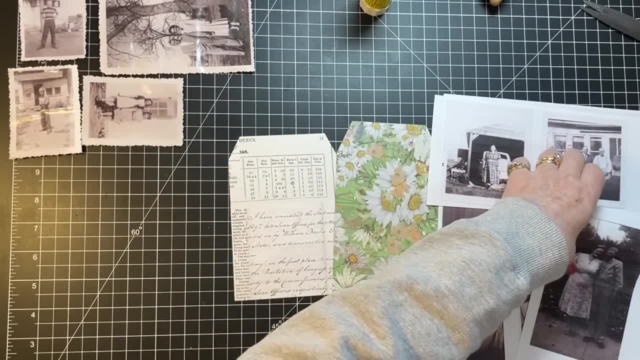 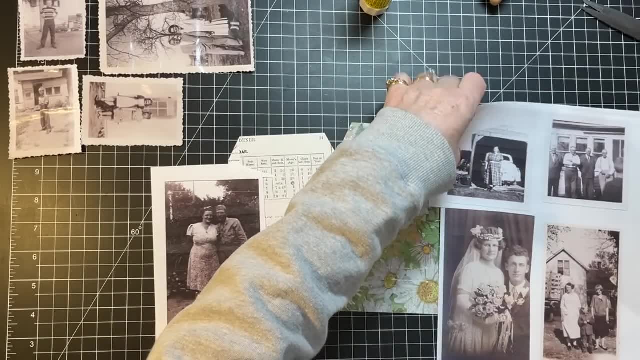 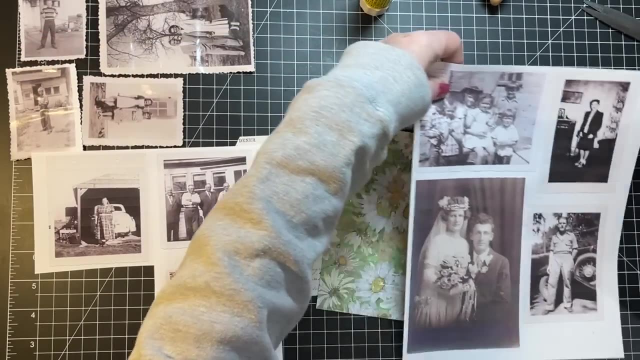 He'd be good on a feature plan. ultimately, We'll have to figure those out. Let's get himкіka um on a journal card. this one could work. this would be a good journal card too. that one could work. i think this one's too big, too big for anything. there be a good um journal topper, though, i think. 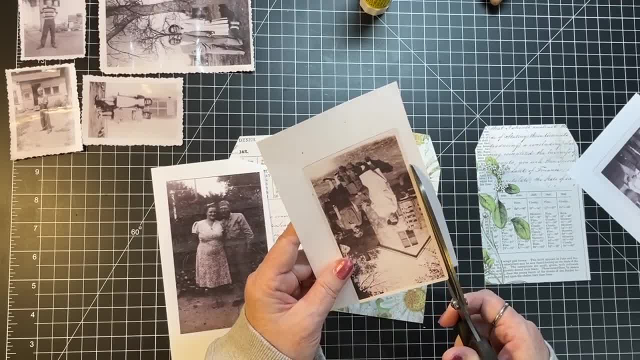 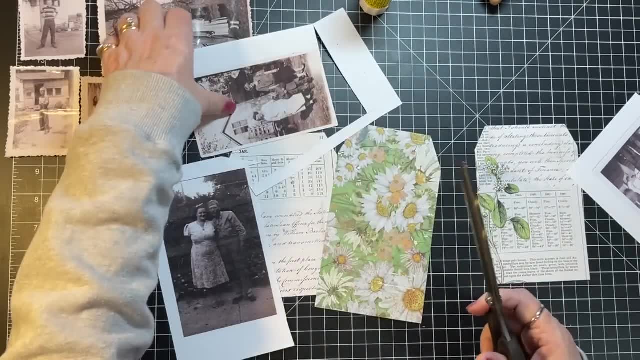 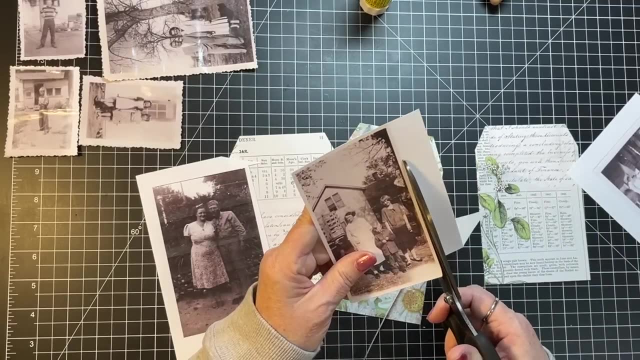 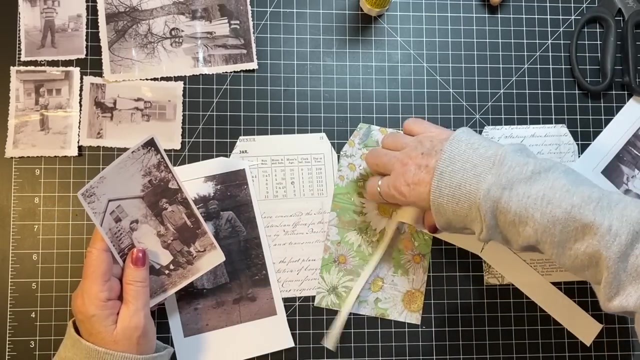 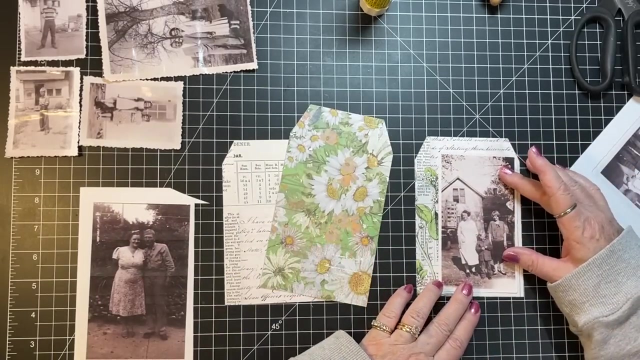 a good journal topper. if you notice in old photographs, often they're in front of a house or in front of a car. i think in those days if you had a house or a car you were pretty darn proud of it. okay, oh, i like that, the flower on the side. 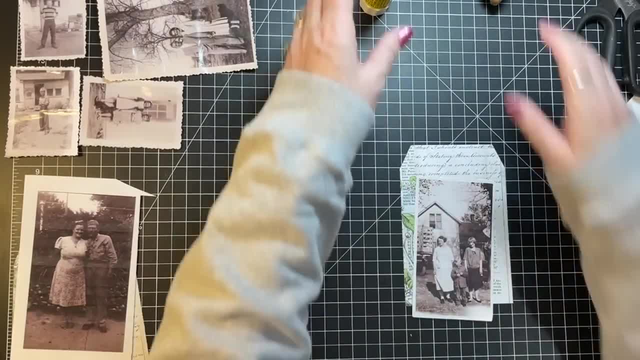 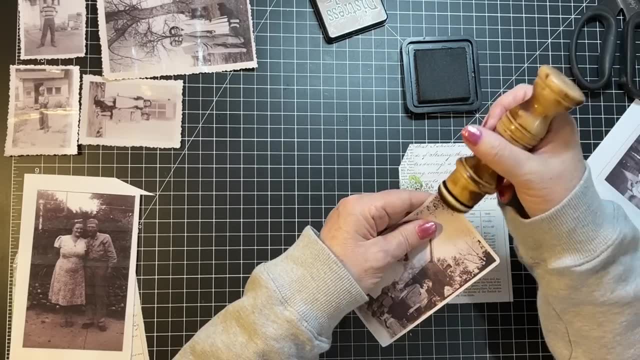 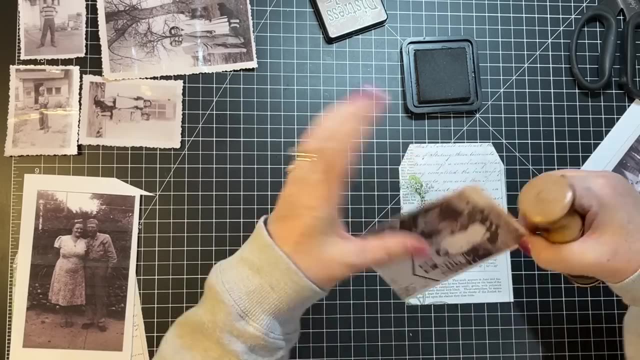 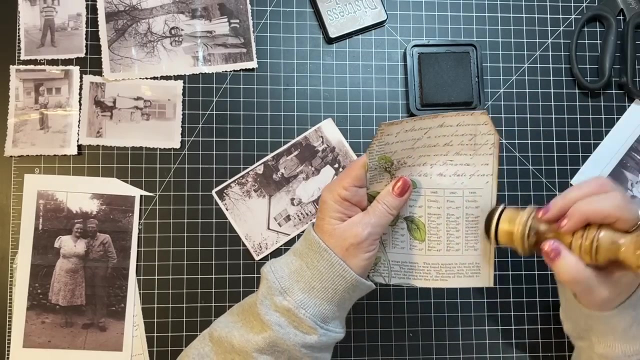 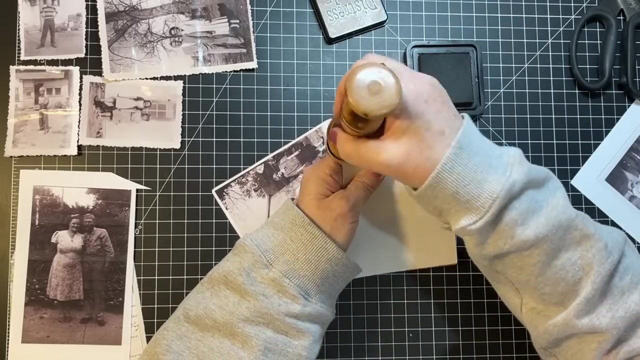 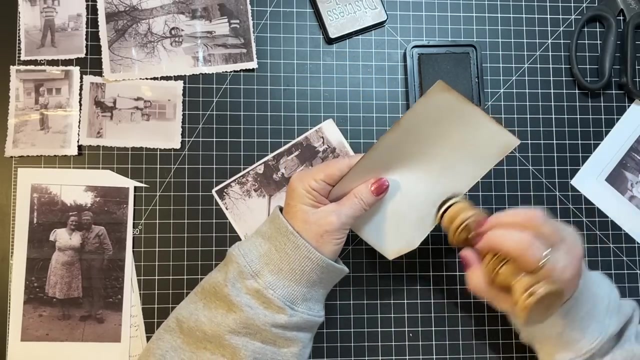 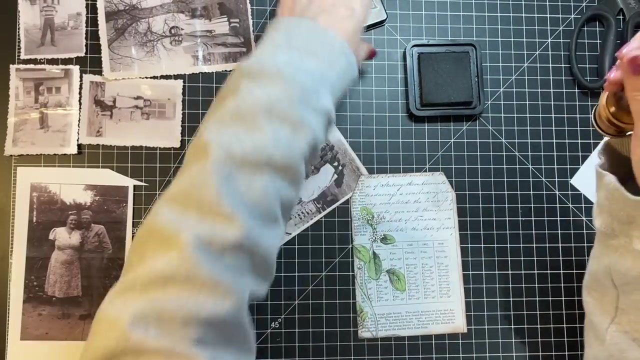 yeah, that could be pretty simple. so i think that's what i'm gonna do, just give that a little on the edge. so, oh and perfect to write on on this side. it's a big old fat journal card. i like it it is. oh yeah, fits on there just fine. just fine, and dandy put that there. 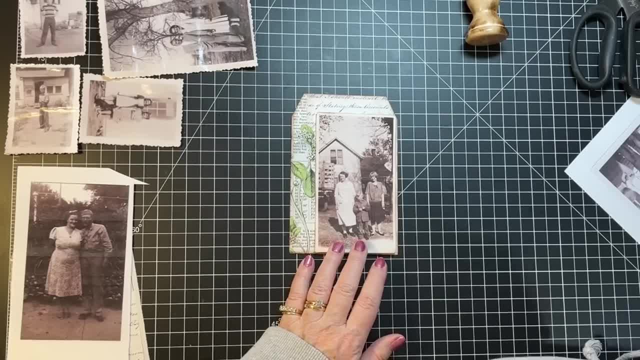 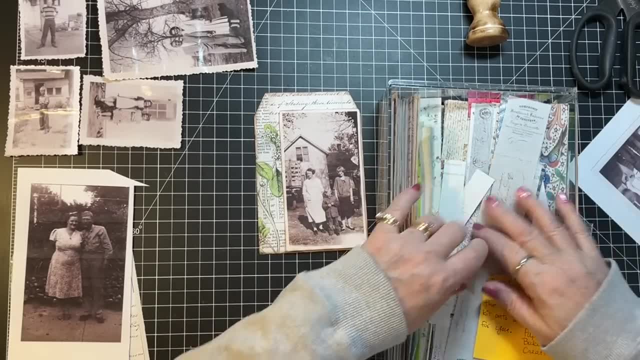 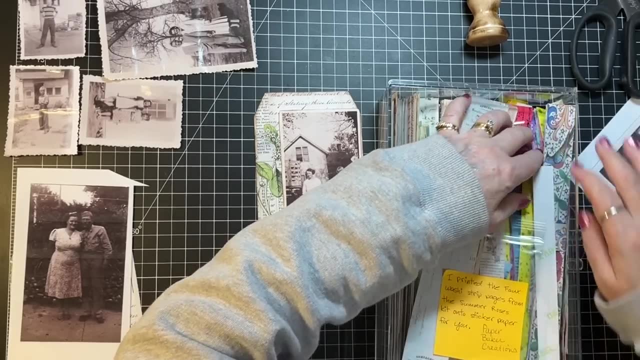 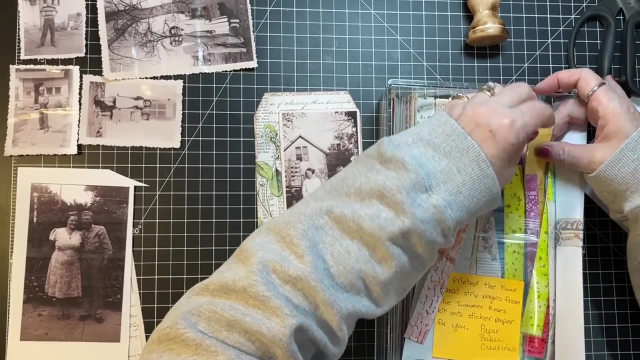 and then do i? i have, i want some of my old looking tape. i definitely think i need more. i don't even know if i have any in here, so me look. aha, i do have a bit, but i'm gonna make some more for tomorrow, okay. 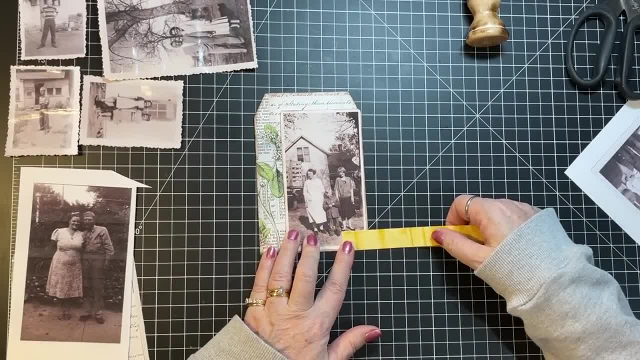 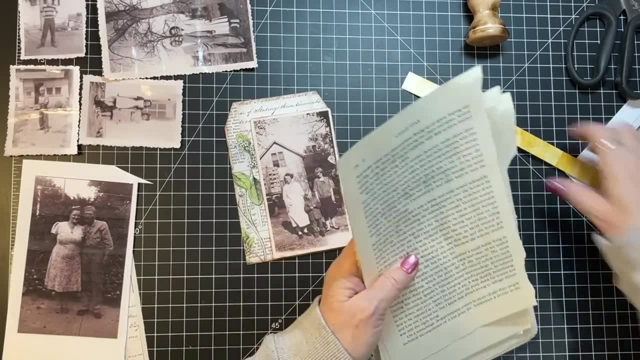 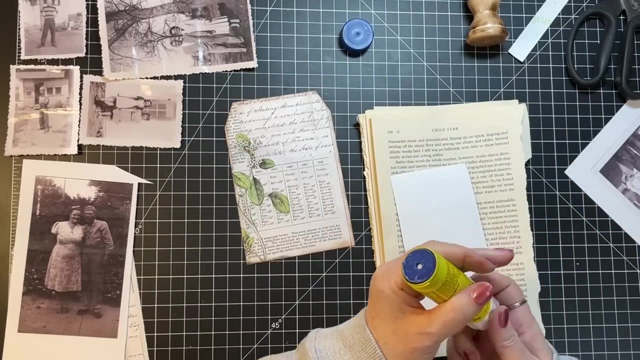 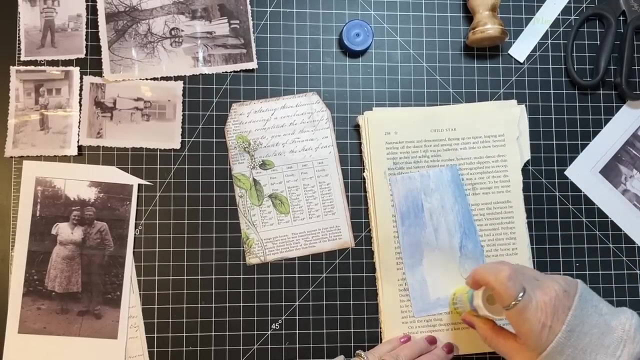 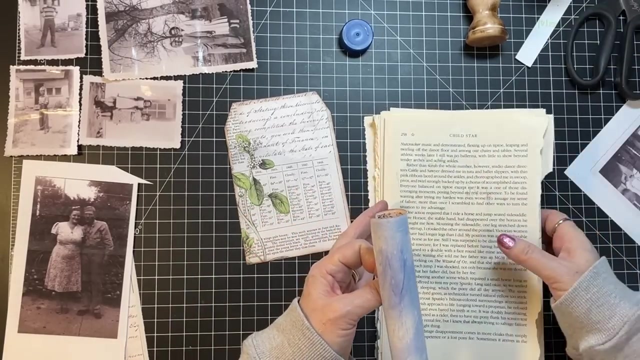 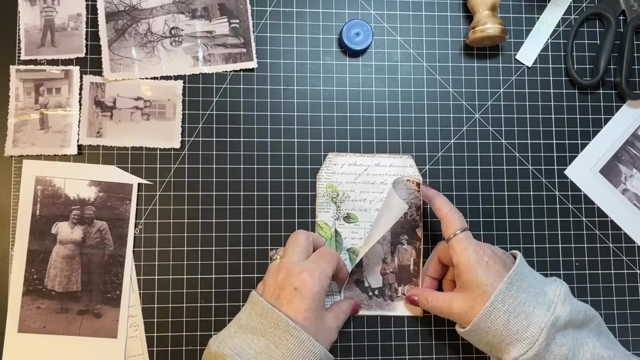 good, because i think i want some old tape, maybe there, and then like: maybe at the top or something, maybe there, anyways, glue stick, that's what i was looking for. yeah, that one big picture, the wedding picture, might be a fun journal topper. i'm a thinking. 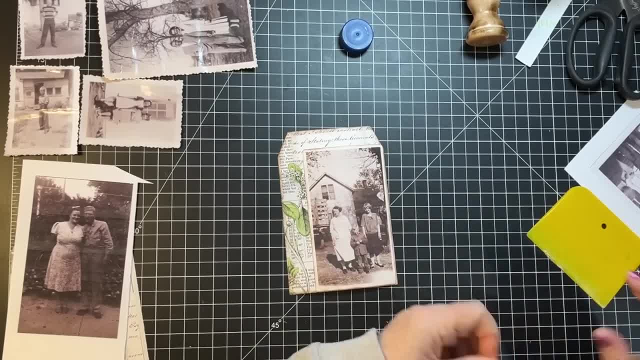 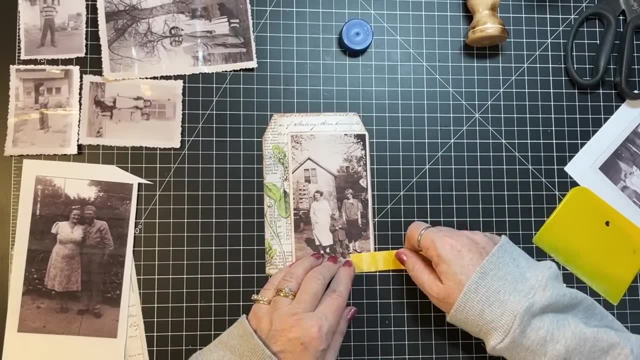 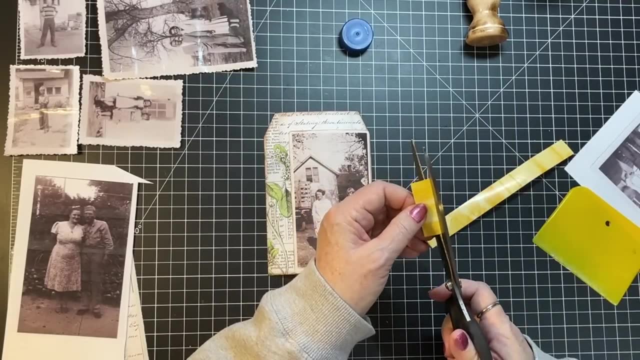 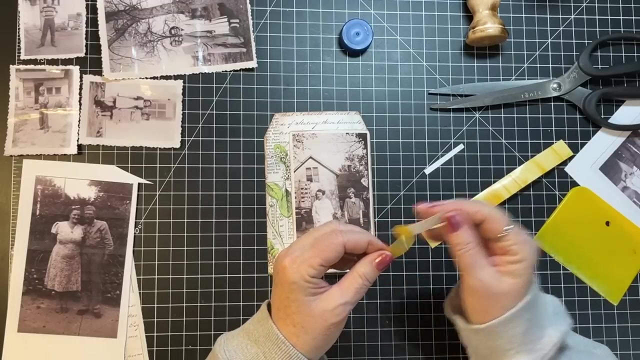 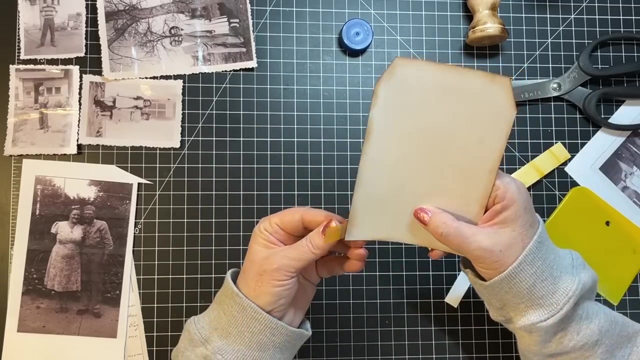 okay. so with that, then i want to put some of this on there. it's a little wide, maybe this: yeah, it's a little wide, but we'll just take a bit off. we don't know what you know. um, uh, whatever, okay, so i'm gonna just combine them all in one. a cat through the knife. 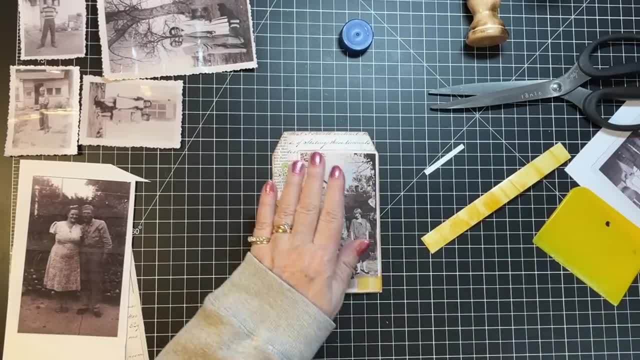 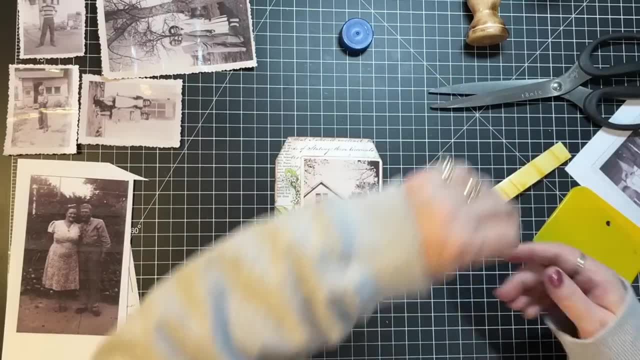 all to make it round this box on here. we're gonna use my folder, which makes it a bit easier to go through this box and then gather up all these samples here. we're gonna use my birthday gift bags, so that's. that's going to make our stuff prepared in a minute too. so these in this bag are the ones that are going to be in the tin bin rigs. so are those angry candles, and with me, hold the mouthworks. so those silver candles and pinks in theEmilyinds はい. 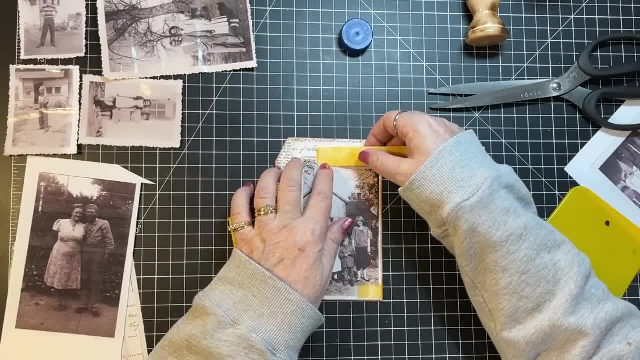 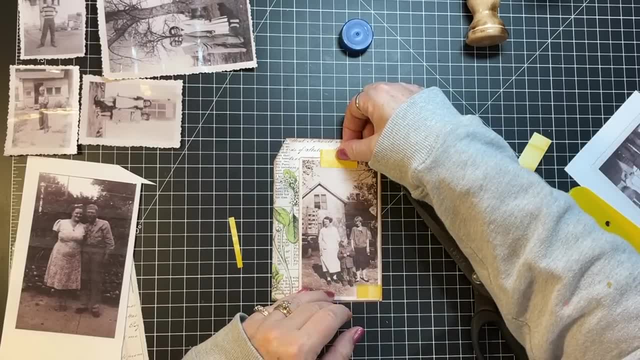 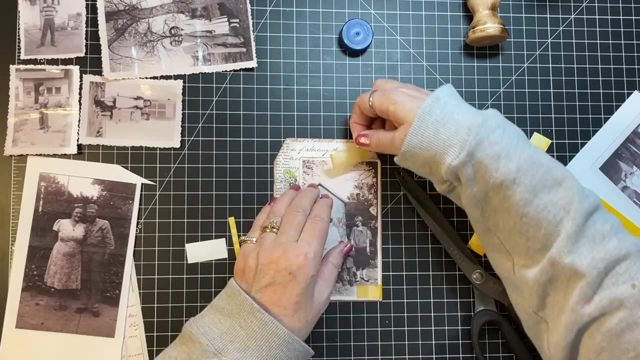 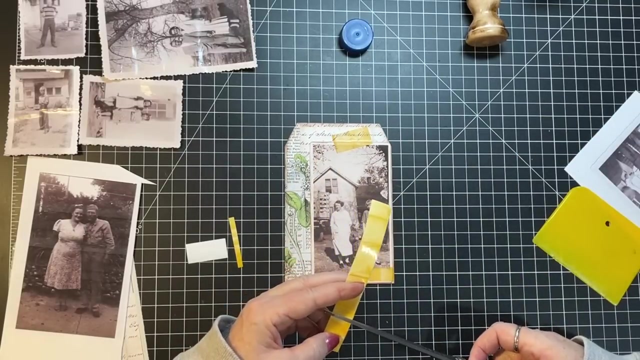 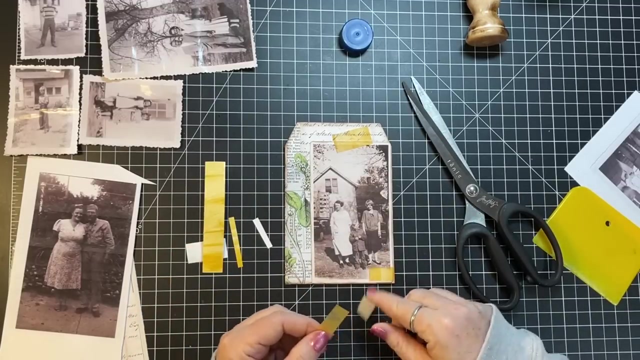 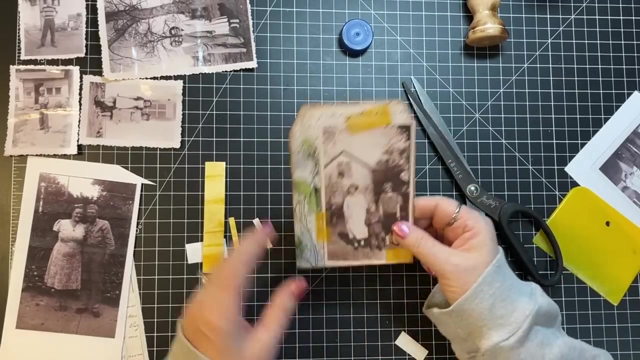 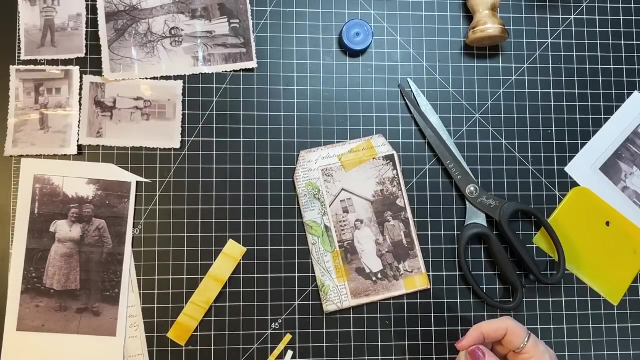 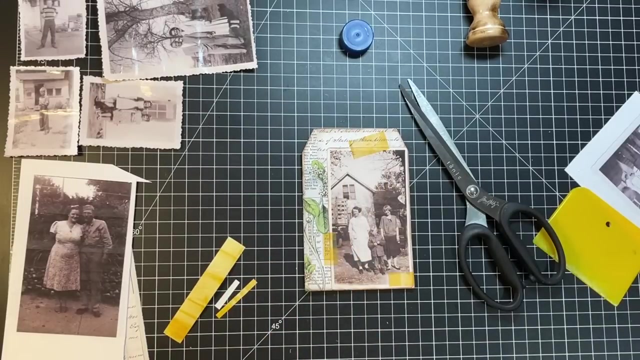 I'm going to put it crooked and just a little piece, and then I'm going to go ahead and put it here: Cute, Okay. I think I want a little slit or something up there. I'm not, I'm feeling my Euro punch, but I think this one might be good. 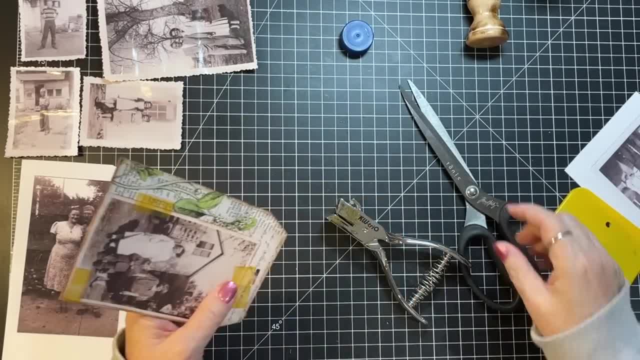 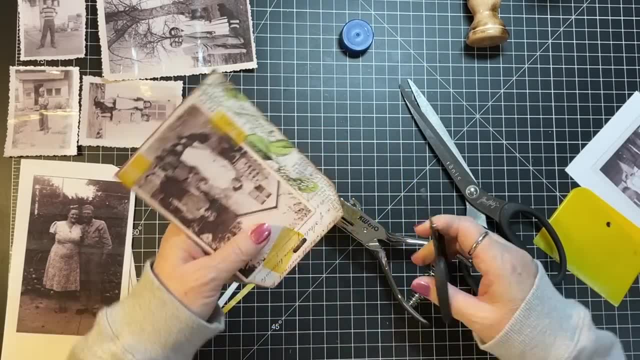 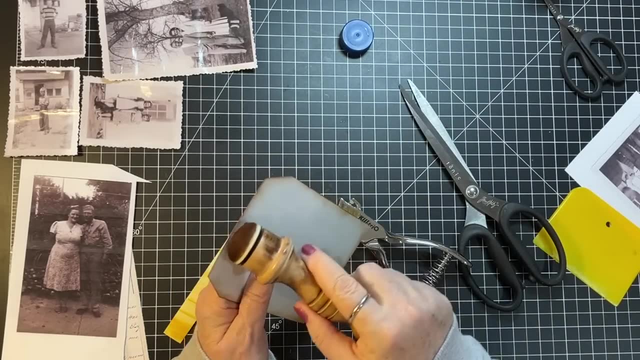 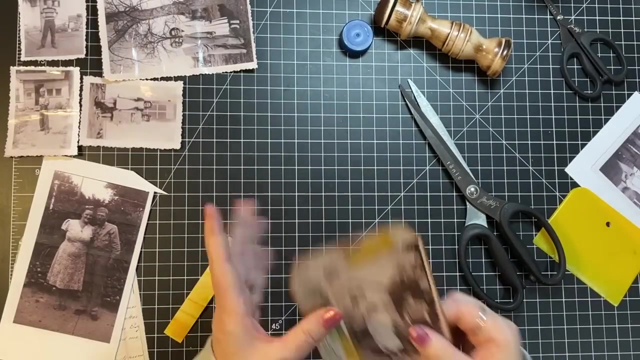 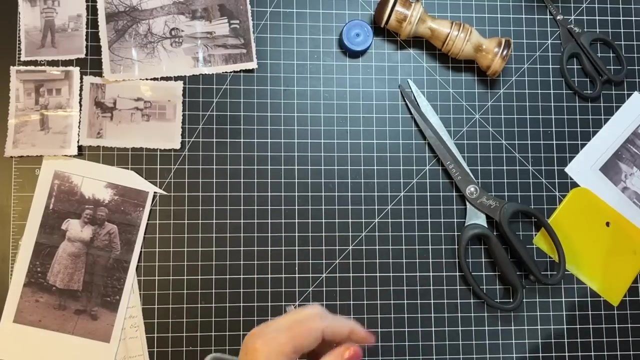 Oh, the tape doesn't want to. Where are my little scissors? The tape doesn't want to cut. There we go. Okay, Oh, that's fun, Very different. Okay, that goes in the stack of duns. Let's slide these over somewhere. Okay, what about you? 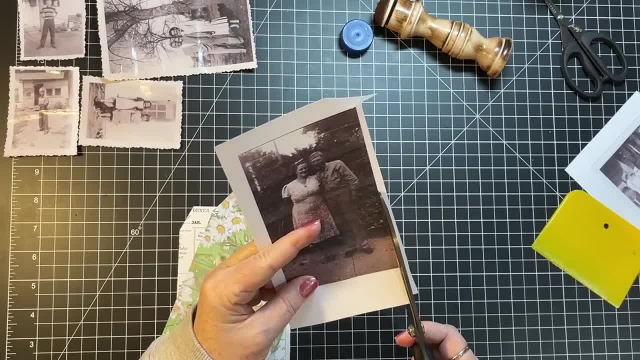 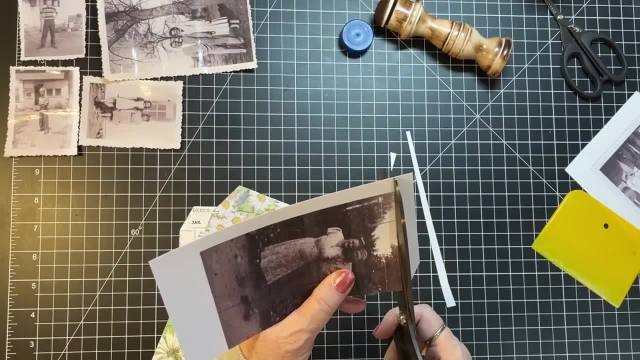 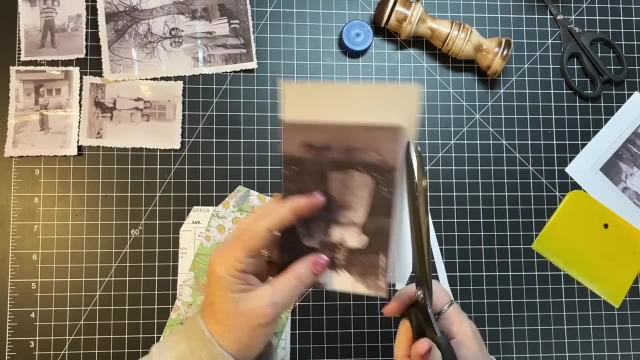 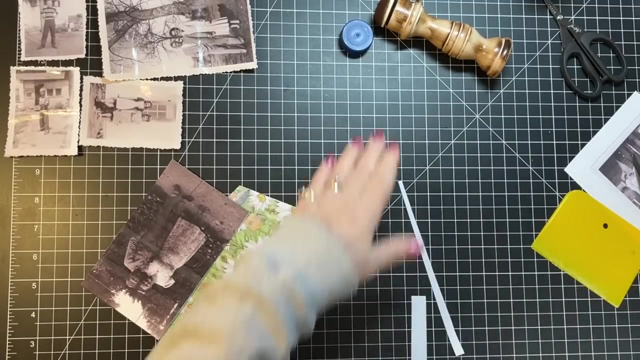 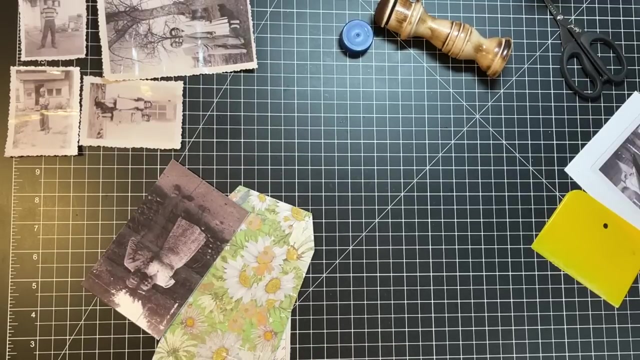 Oh, and I figure if I don't like it on the tag, that's okay. It's cut out for another. Another project along the way. Okay Gosh, I have little bitty jaggedy crumbs all over me from cutting out those pictures. 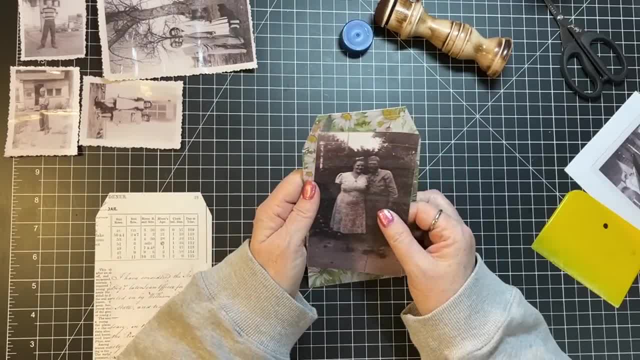 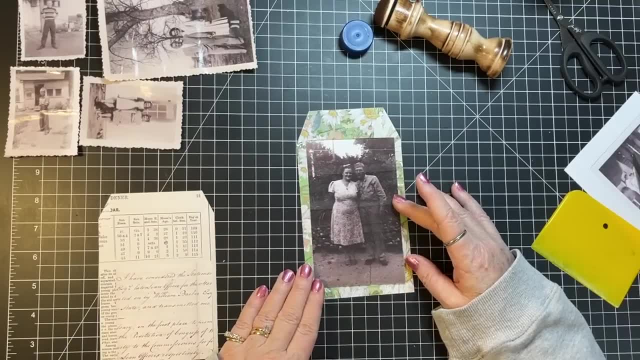 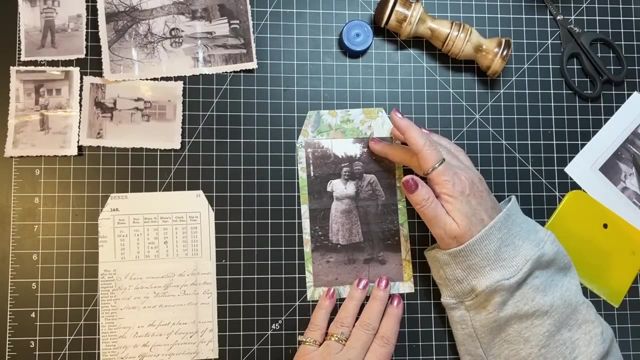 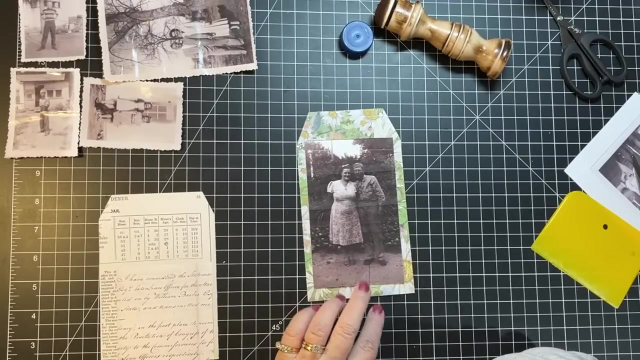 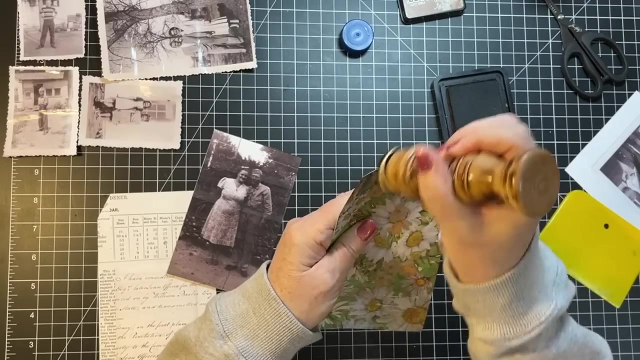 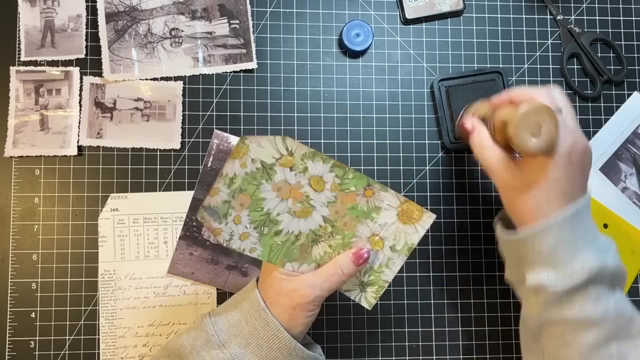 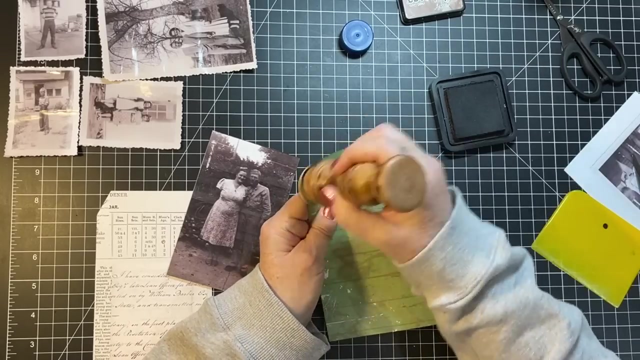 Get those off. Okay, I was thinking for this one. I like it, but I want, I want more on there than that. I think Something down there, Huh, Oops, Sometimes just inking and thinking helps Very, very springy paper, so that'll be fun. and gosh, I can't believe how great those pictures turned out. 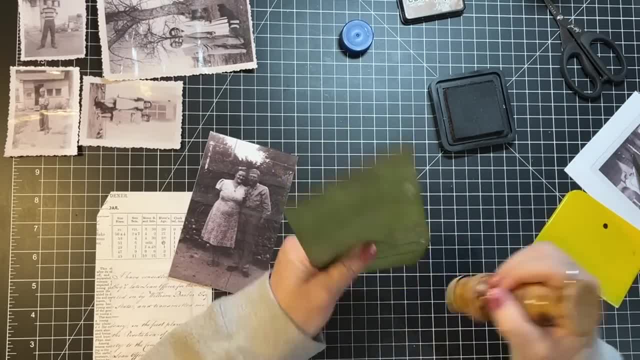 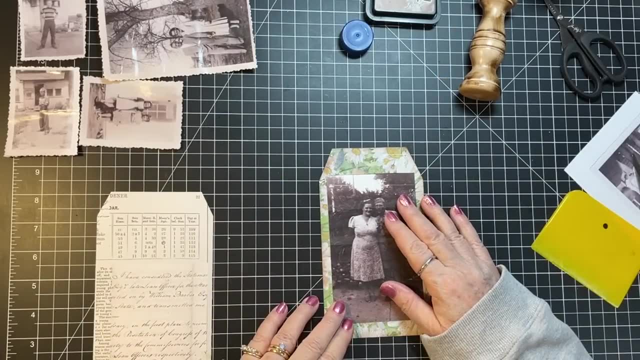 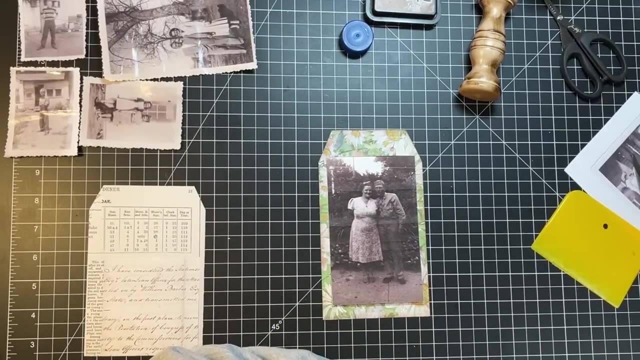 They're drying over there and I'm just, I just keep staring at them. I love them. That's really fun. I just you know, because when you're thinking about something, it's like not necessarily I don't know, you don't know it's gonna work, i don't know it's gonna work. what do i want to? what am i thinking? 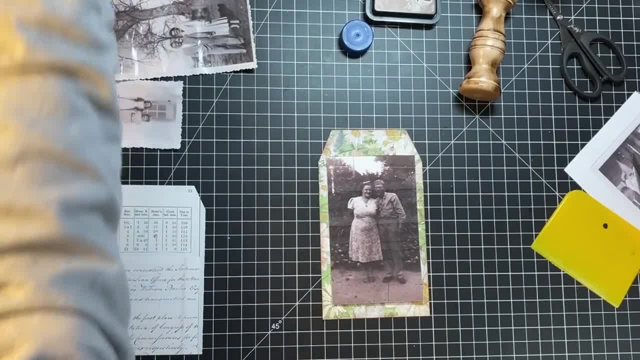 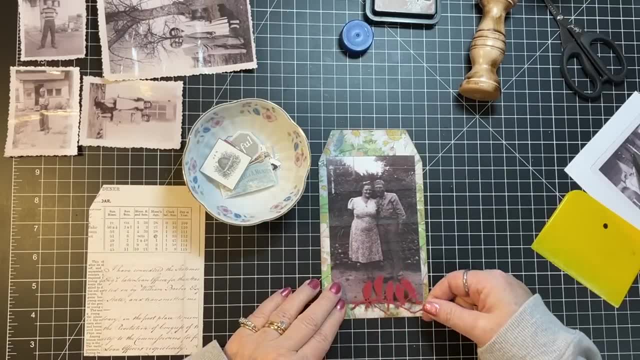 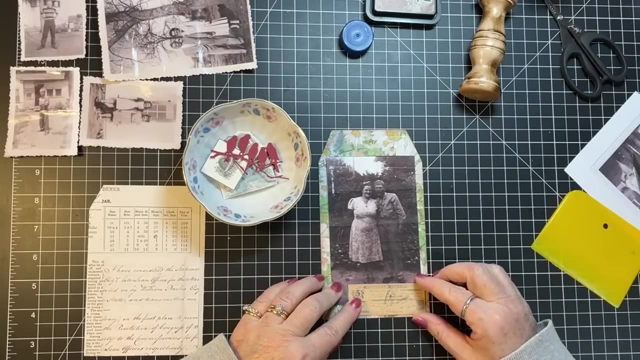 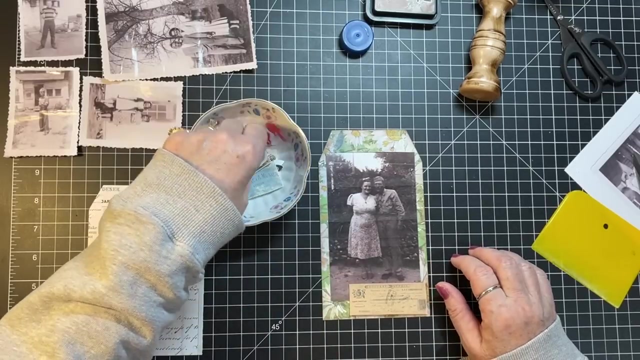 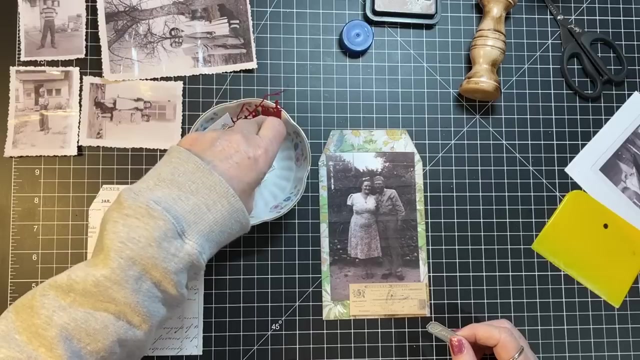 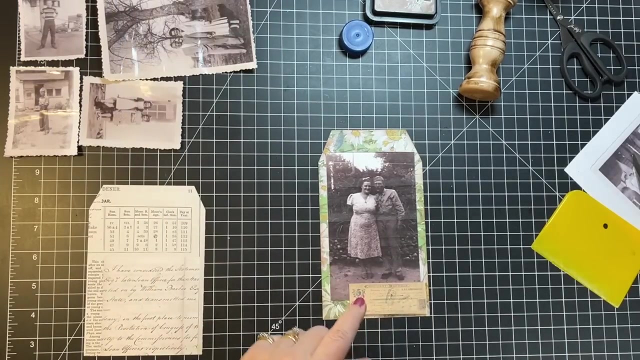 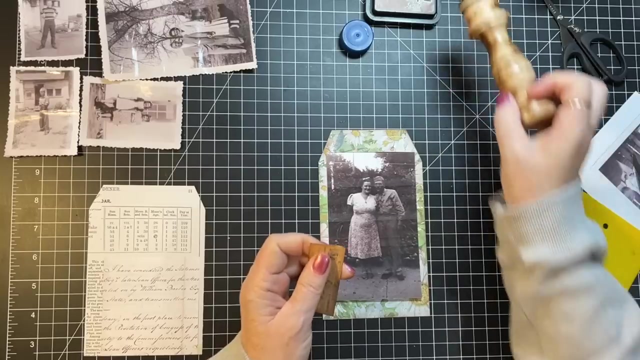 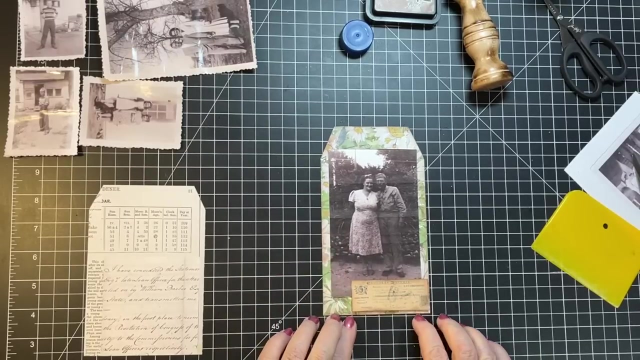 here got some bits in a in my little little jar here. that doesn't go quite right. this isn't bad. and then what? here's a lovely, but i don't think i want that color. i like that. i just gotta figure out something else to put kind of there. um, 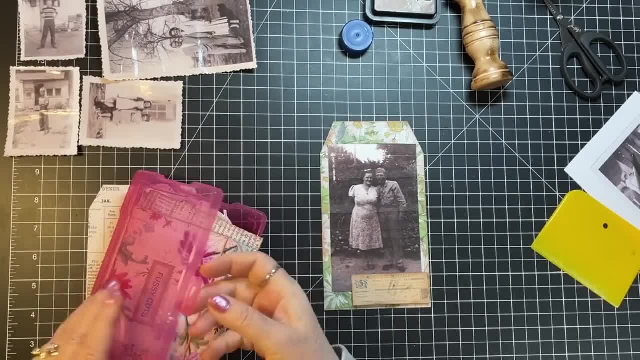 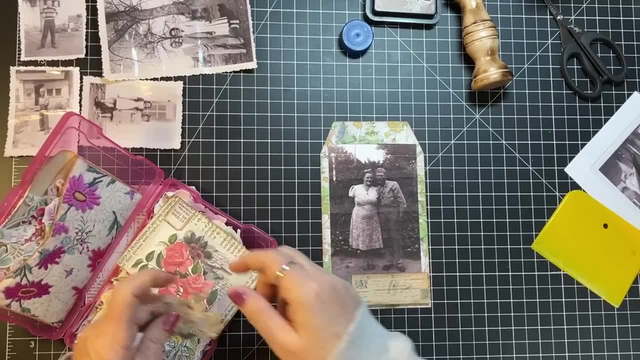 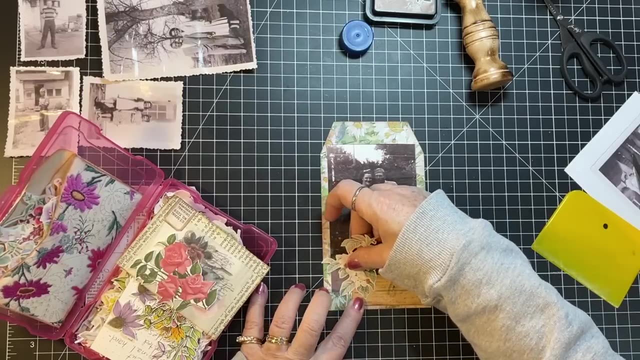 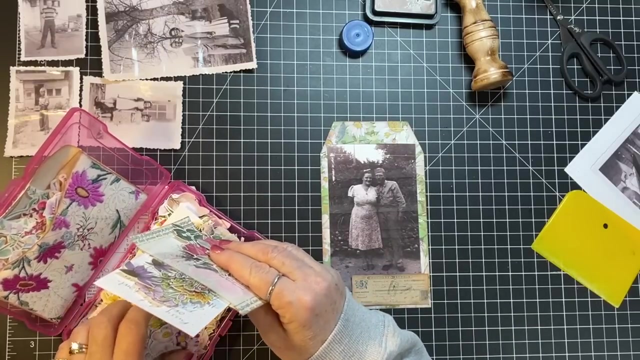 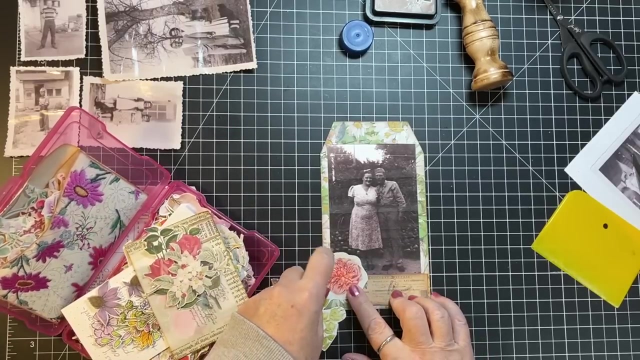 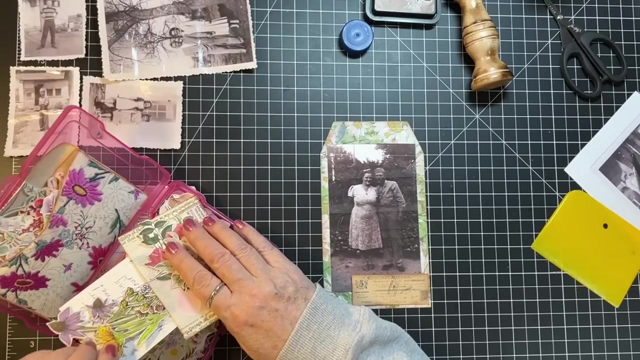 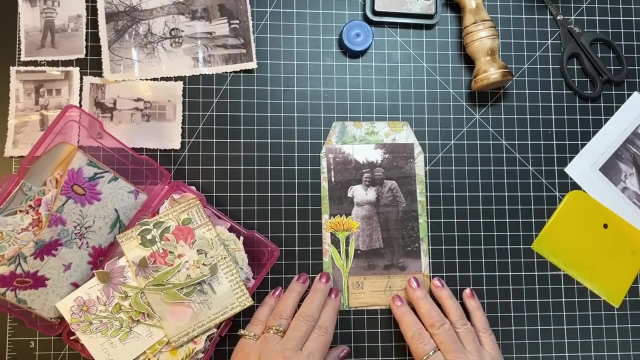 could be a flower, maybe, i don't know. i have something kind of small enough first of all. that's upside down, it's too big. um, what do i have? i almost feel like i need yellow. i've got something yellow in here. i can move this over here. 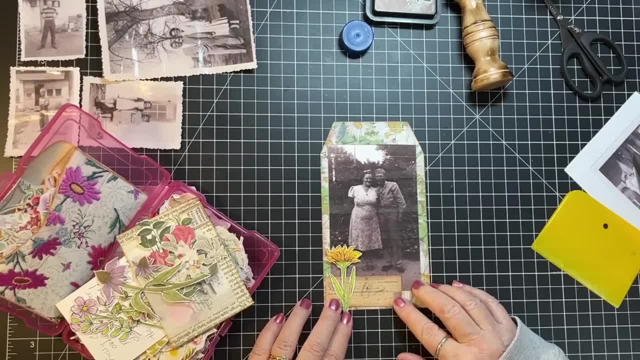 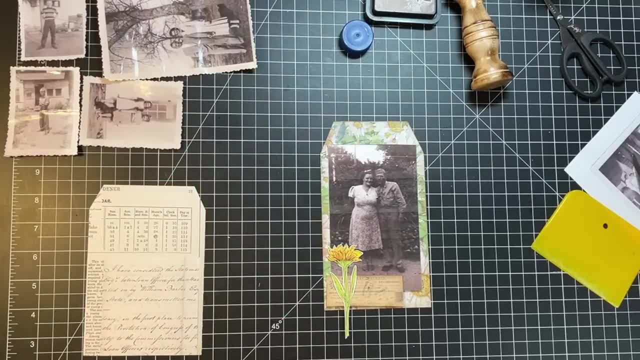 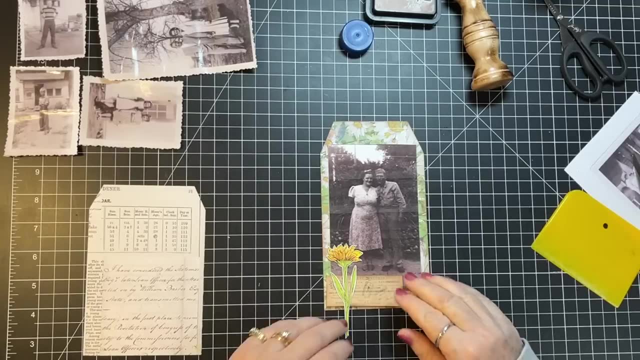 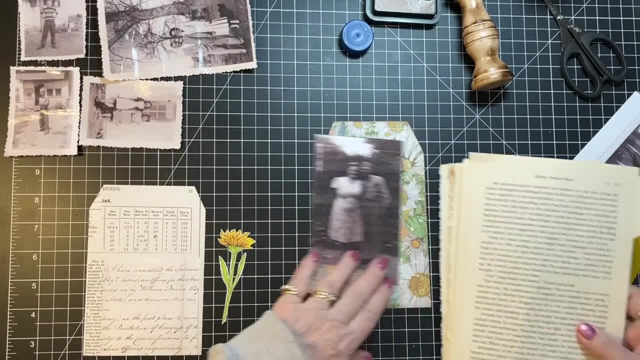 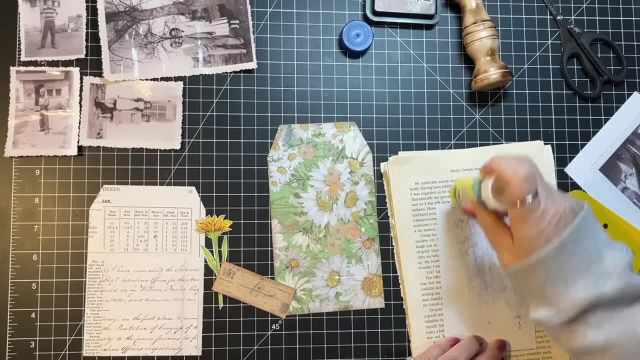 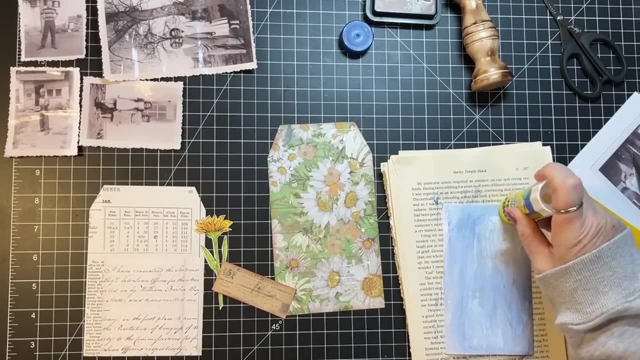 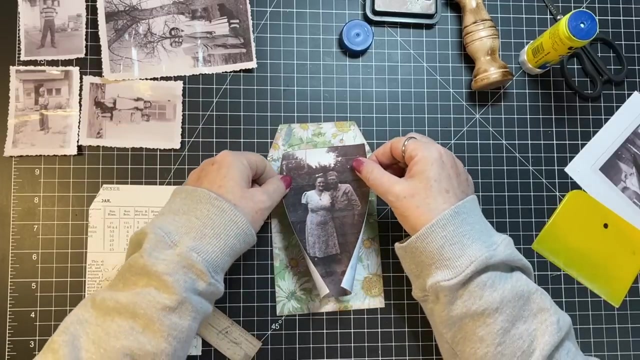 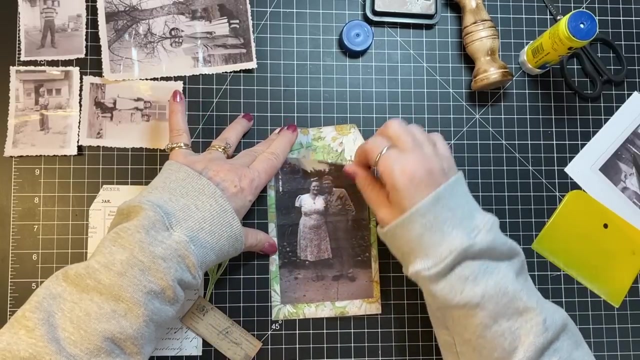 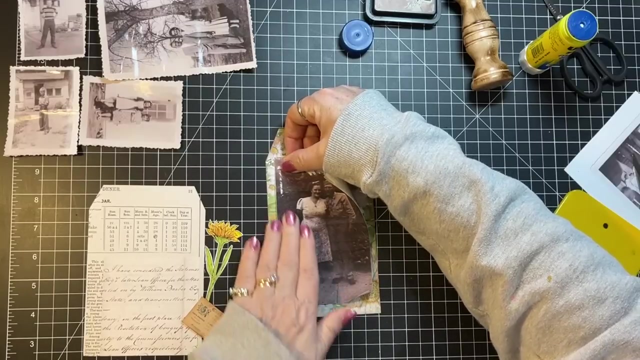 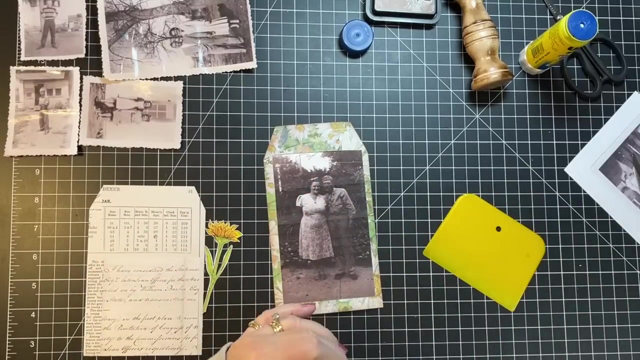 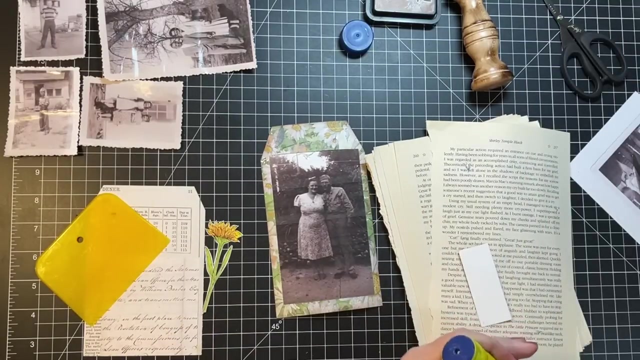 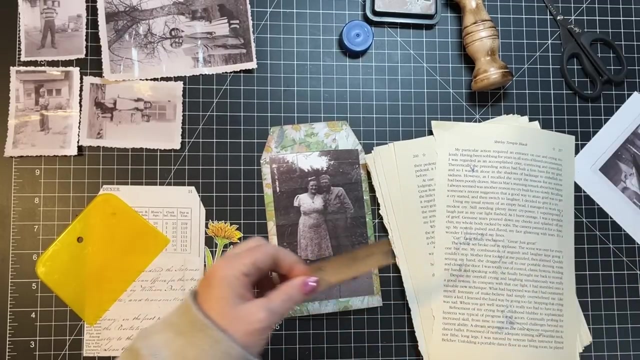 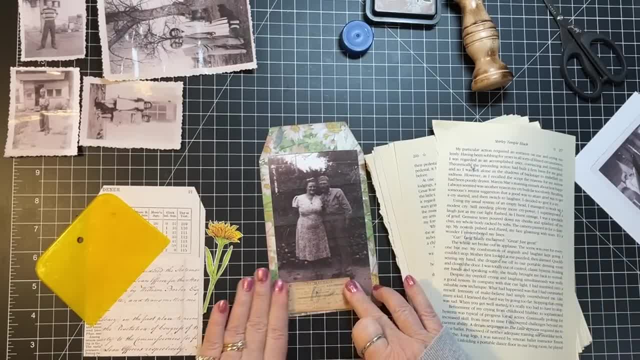 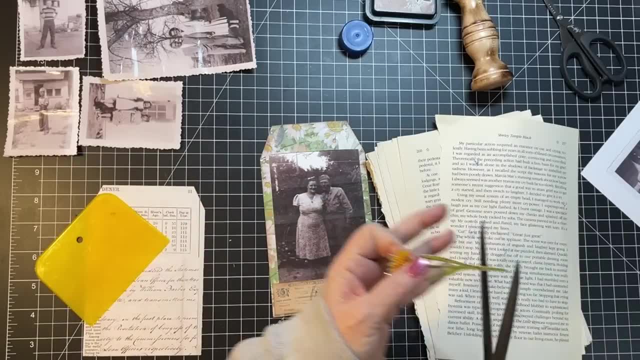 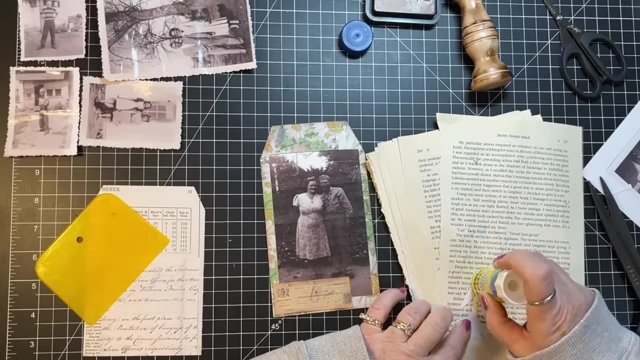 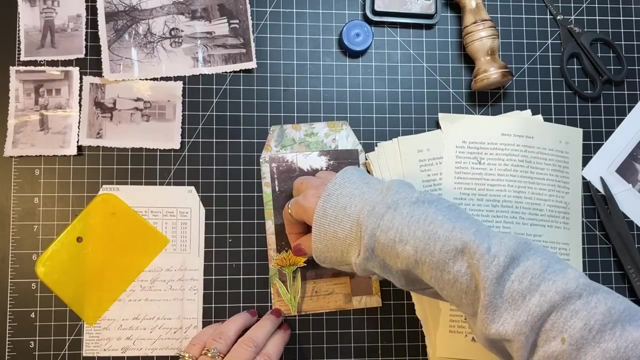 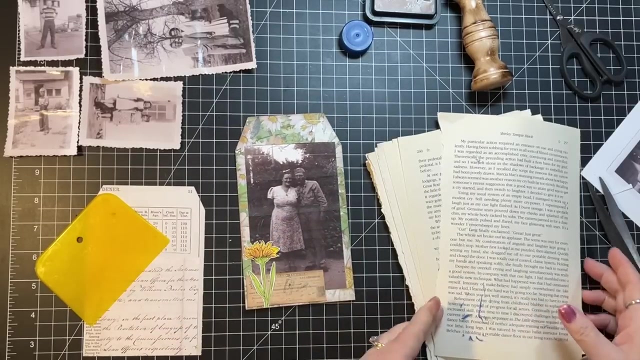 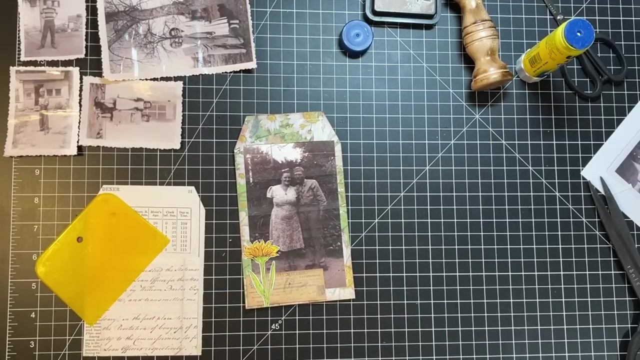 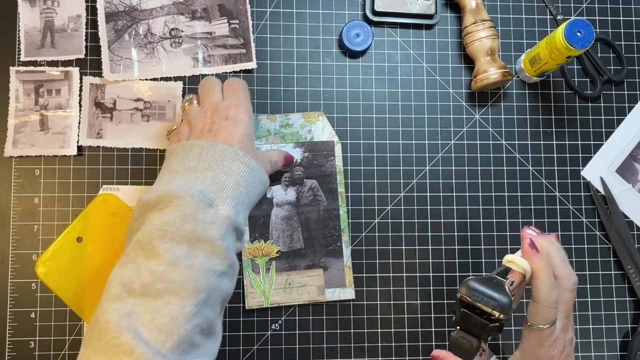 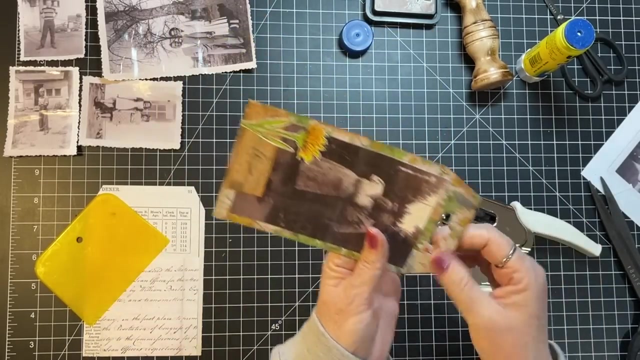 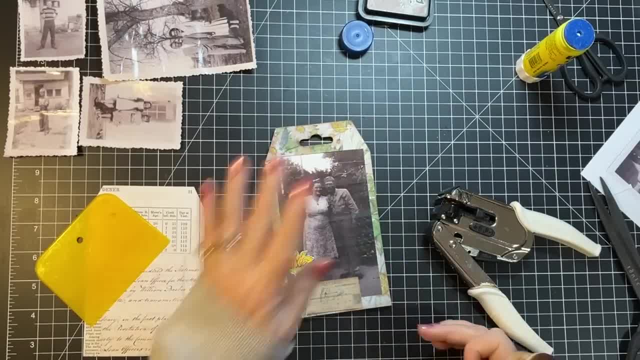 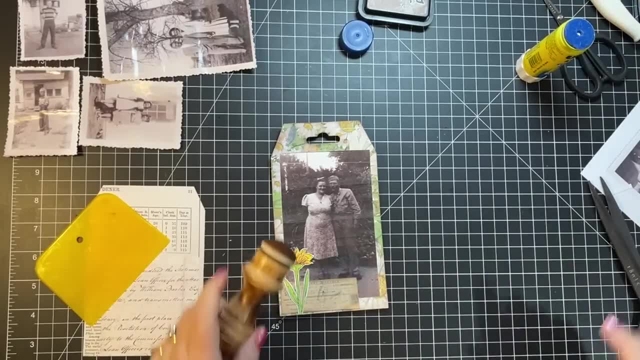 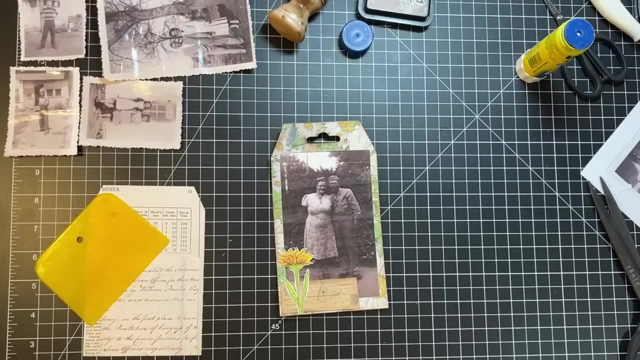 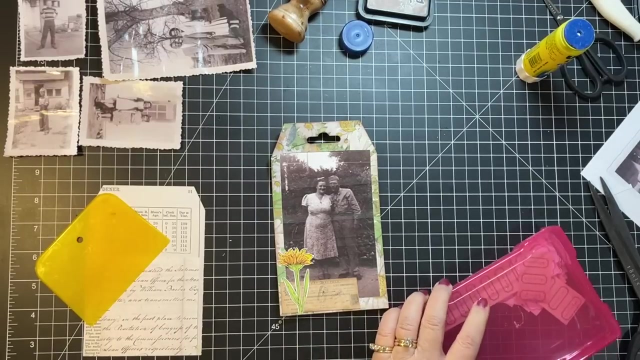 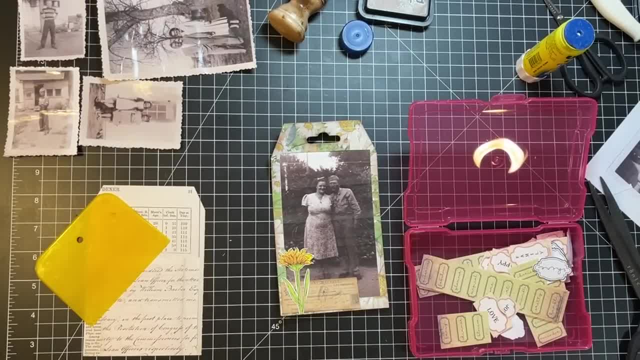 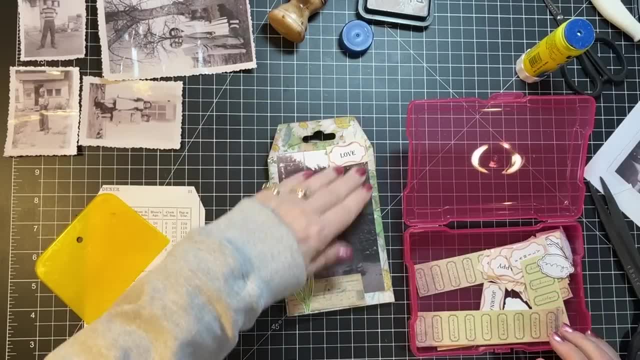 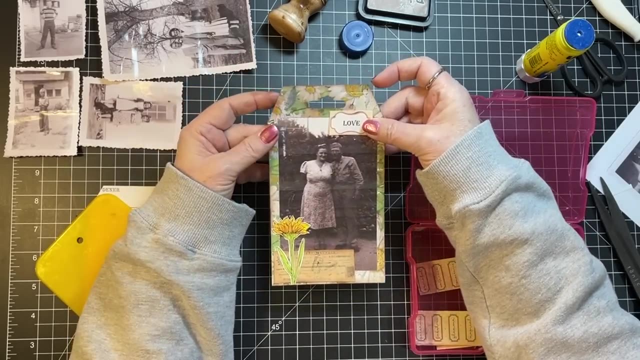 okay, i got some words here. this is okay. i got some words here. this is: these are from, these are from, these are from nancy's fancies and i was wondering about putting that right, about putting that right, about putting that right kind of right. there i think i will. 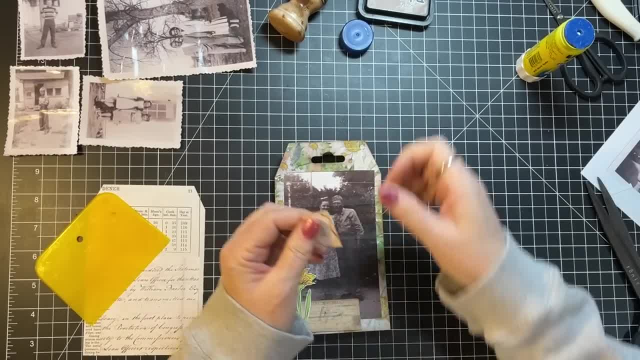 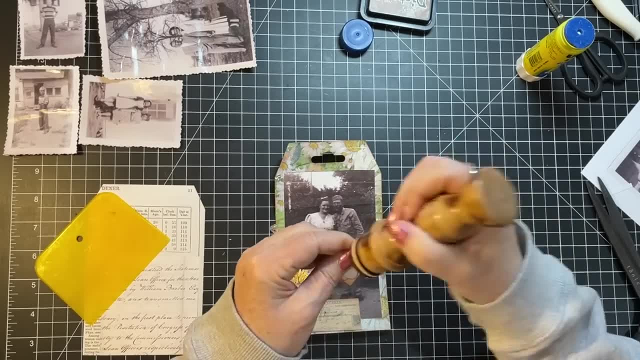 nancy's fancies. i think that's a fun name: nancy's fancies. i think that's a fun name: nancy's fancies. i think that's a fun name for a shop, for a shop, for a shop. gosh, still so tickled with those. 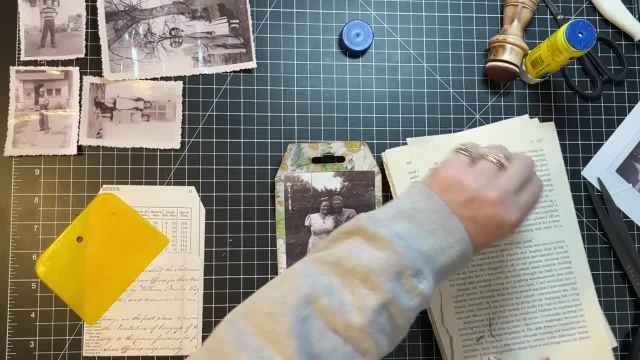 gosh, still so tickled with those gosh still so tickled with those pictures. we used up a good bit. we only have a half. we used up a good bit. we only have a half. we used up a good bit. we only have a half a dozen. 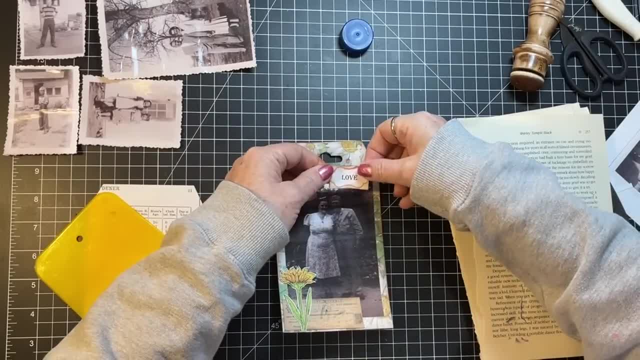 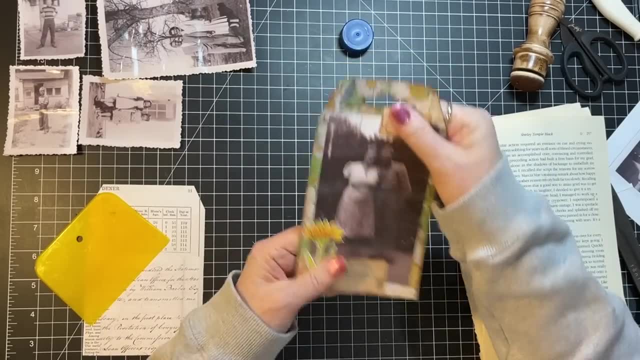 a dozen, a dozen pictures left. i have to reprint pictures left. i have to reprint pictures left. i have to reprint why? okay, there's that one all righty, then okay, there's that one all righty, then okay, there's that one all righty. then where are we? 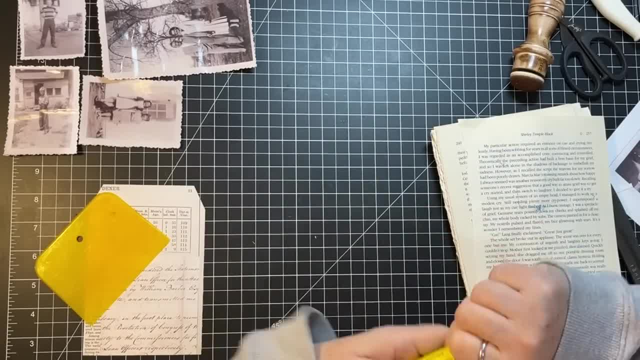 where are we? where are we? oh yep, we're almost there. oh, yep, we're almost there. oh yep, we're almost there. so i'm gonna go ahead, and so i'm gonna go ahead, and so i'm gonna go ahead and scooch things over, and we'll take a. 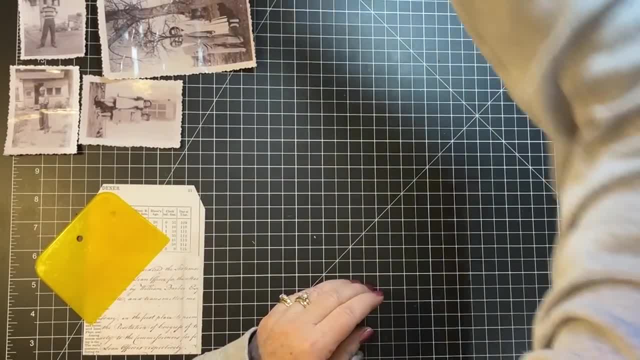 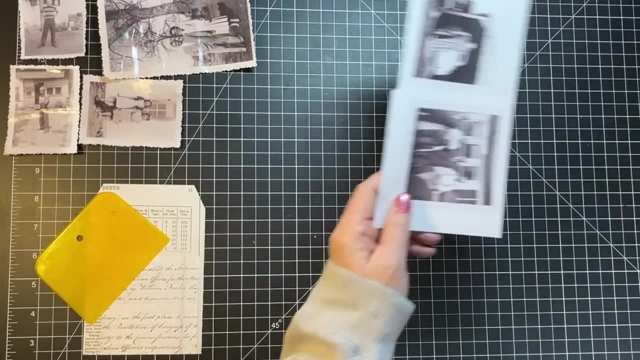 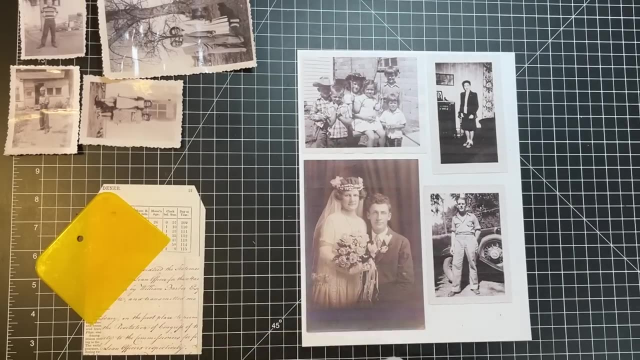 scooch things over, and we'll take a scooch things over and we'll take a look at what we did. so what do we have left? we just have just have a few. this is the only full. just have a few. this is the only full. just have a few. this is the only full sheet left. 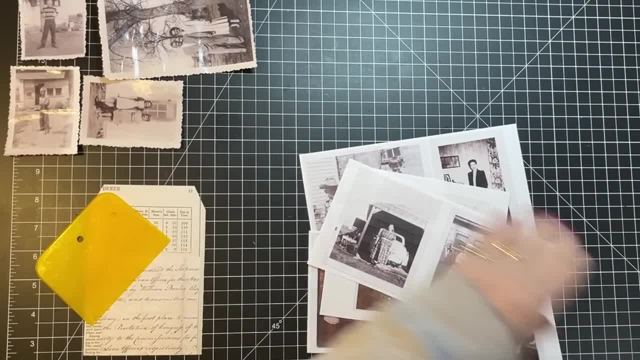 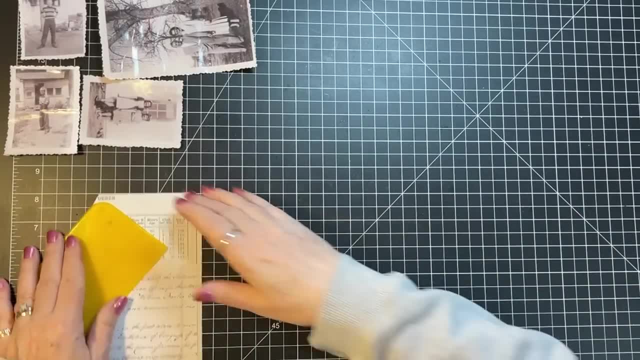 sheet left, sheet left. so that is awesome. so that is awesome. so that is awesome. more to play with later. more to play with later. more to play with later. there's some great ones for journal cards. there's some great ones for journal cards. there's some great ones for journal cards there. let's see, this guy has to go back. 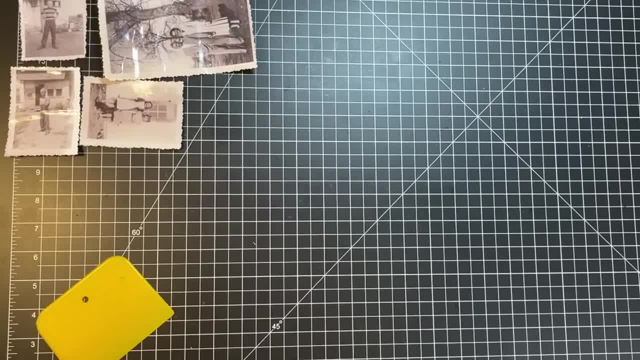 there. let's see this guy has to go back there. let's see this guy has to go back in the to-do. but we got a couple of them done okay, so, but we got a couple of them done okay, so, but we got a couple of them done okay. so here's these. 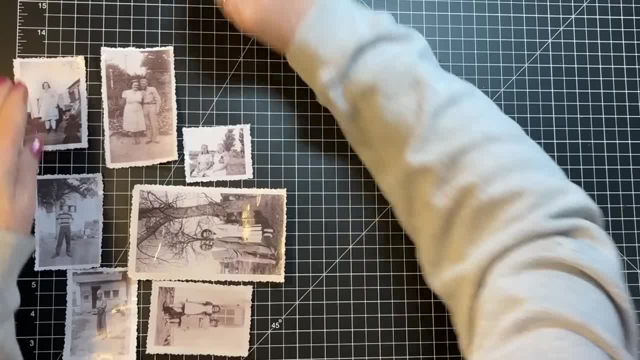 here's these. here's these that we did and journal cards. they will that we did and journal cards. they will that we did and journal cards. they will be be be just little. this will be fun to tuck in. just little. this will be fun to tuck in. 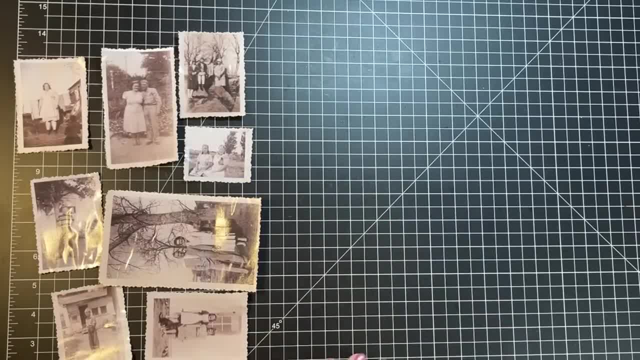 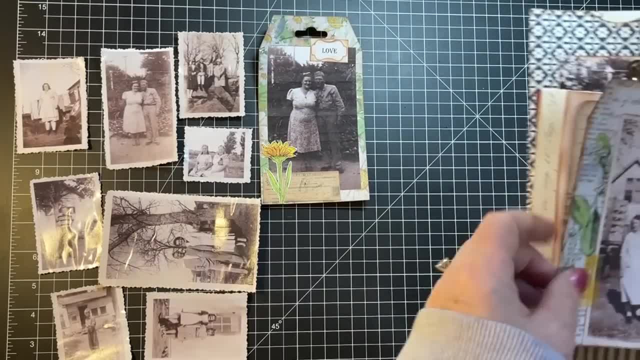 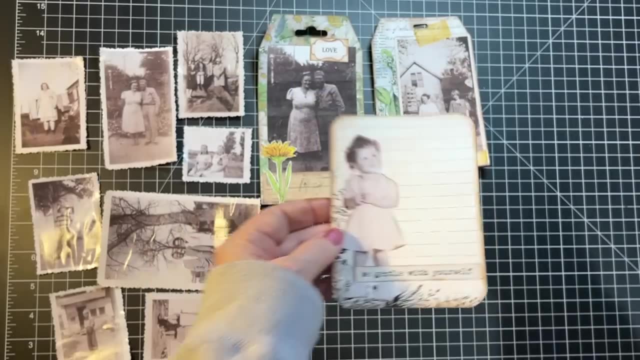 just little, this will be fun to tuck in. just a little pocket, just a little pocket, just a little pocket. these two little girls and these two little girls and these two little girls, and we just did this one and that one did this little sweet girl. we embellish the front of this little.